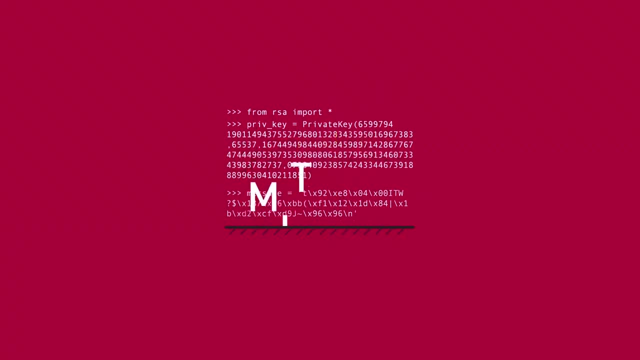 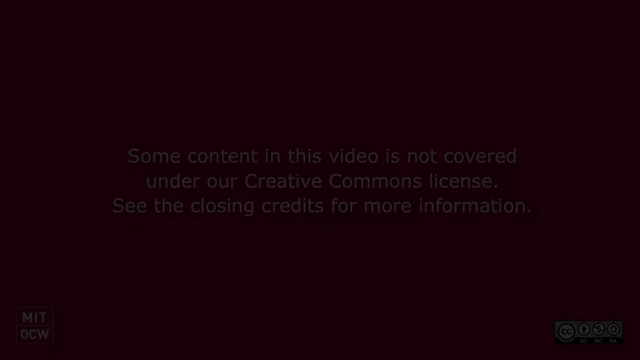 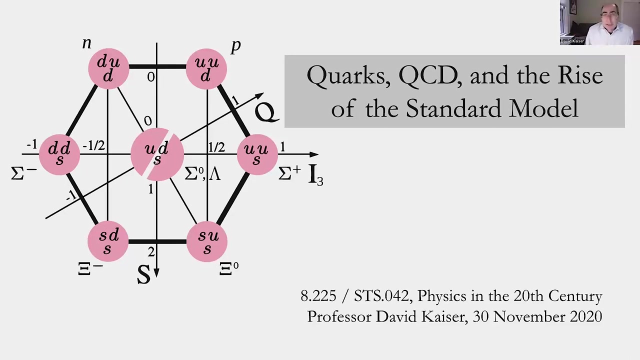 Today we're now sort of in the middle of our unit, of our, of our last main unit on a kind of quarks to the cosmos, high energy, trends in high energy physics, astrophysics and gravitation and cosmology, and so today we'll be picking up part of the kind of threads that we, that we were looking at before. 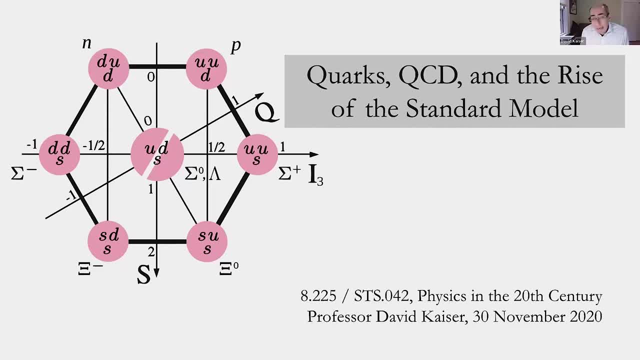 the thanksgiving break and and we'll be looking in particular. how was it, and over what kind of time scale was it, that most physicists came to be convinced that many, many types of matter are actually formed of quarks, that there's a constituent sort of elementary unit within many 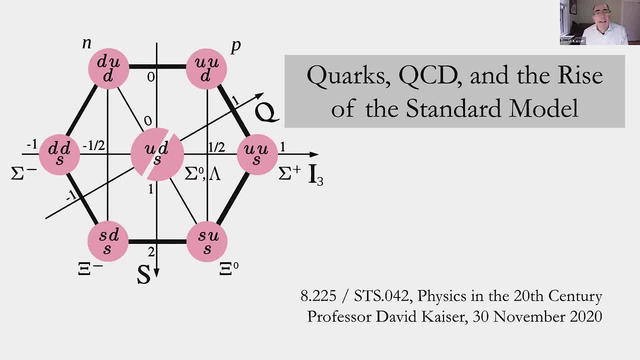 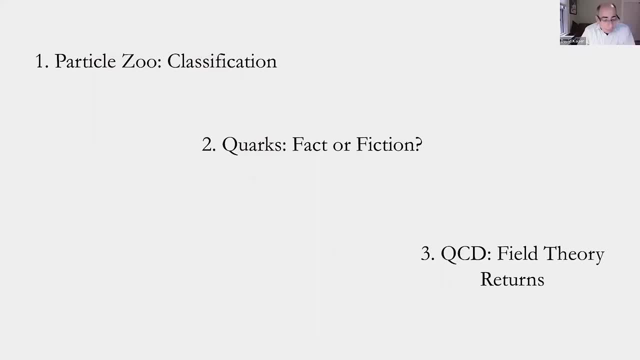 kinds of matter. how did people come to be convinced of that and over what kind of time scale? so that's what we'll look at for part of today. so the three parts will revisit some of the trends that we already began looking at briefly again in the class sessions before the thanksgiving break. 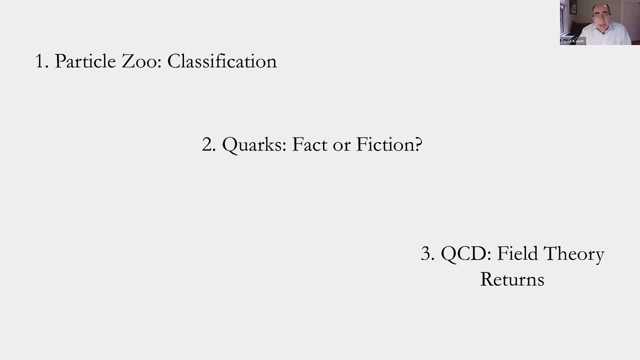 in particular this: what seemed to be a really unexpected and at times almost overwhelming proliferation of the number of particles that seem to come out practically every time that the physicists turned on their often brand new particle accelerators, we saw there's a huge spate, a kind of 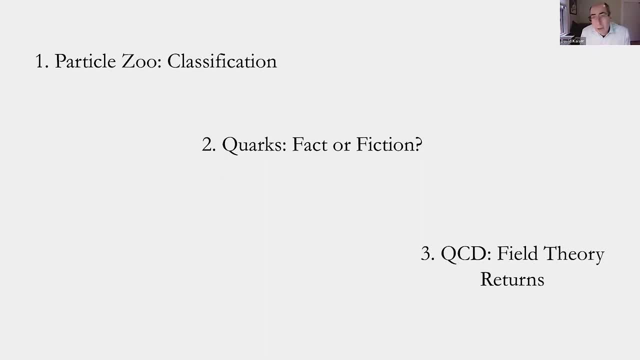 building boom coming out of the atmosphere, and then we'll be looking at some of the trends that we we'll be looking at some of the trends that we'll be looking at, some of the trends that we of the second world war, of making larger and larger, more and more powerful accelerators mit. 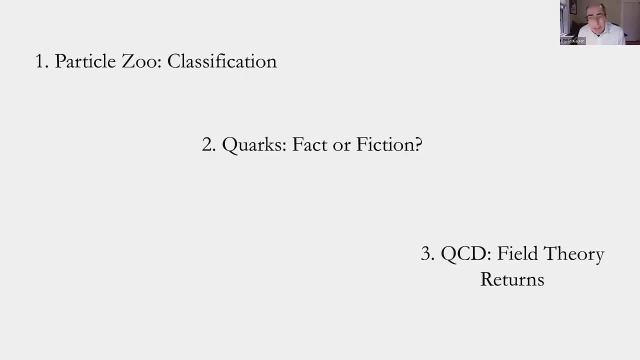 had our own synchrotron in operation for many years. many, many individual universities had them and of course there were larger um national laboratory facilities as well. all a kind of carryover into the post-war period of um of the wartime manhattan project. these were atomic energy. 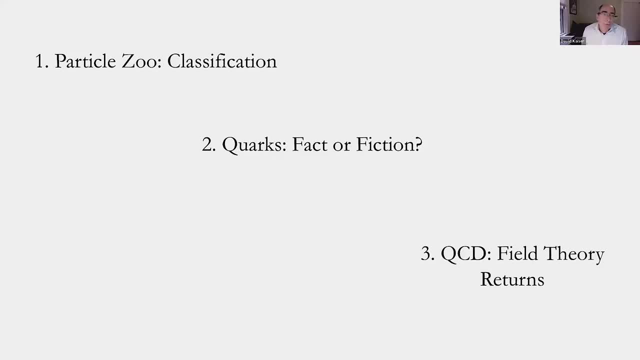 commission facilities- uh, by and large. so what? what were some of the responses to this proliferation of new kinds of particles that seemed to be popping up all over the place? so what, what were some of the responses to this proliferation of new kinds of particles that we'll see that that was really on many people's minds when they began thinking about what we now. 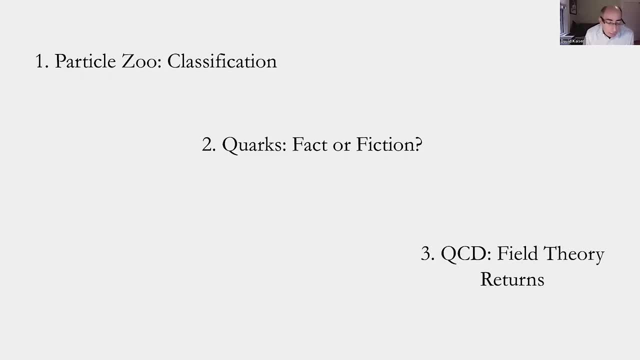 call quarks. the idea about quarks itself has a really, i think, fascinating kind of up and down history where not everyone was on board at the same time and the same for the same reasons. there was a kind of long ambivalence or confusion, or what are they? are they real, are they not? and so 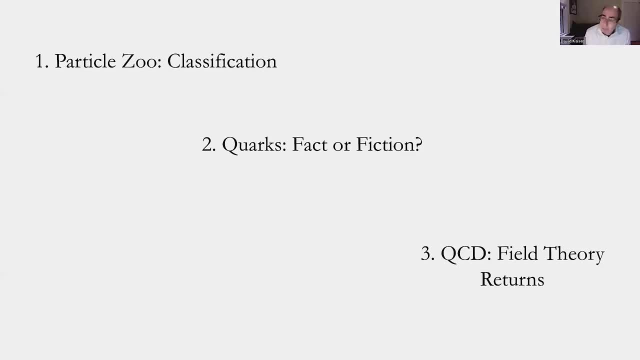 we'll look at that for a good chunk of today's class session and the last part will be a kind of um, what? what has become called, uh, the, the so-called standard model. we'll look at a key part of that called quantum chromodynamics or qcd, which you probably heard of, at least you probably recognize the name. 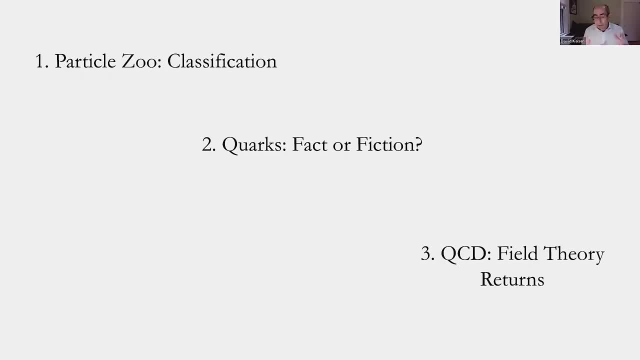 we'll talk a little bit about where that comes from and how that fits into, um, a kind of larger picture today, and it's drawing on this uh sort of many decades coming, uh, coming before it. that we'll look at for today, so that's where we're heading. to quick reminder, as i just mentioned, 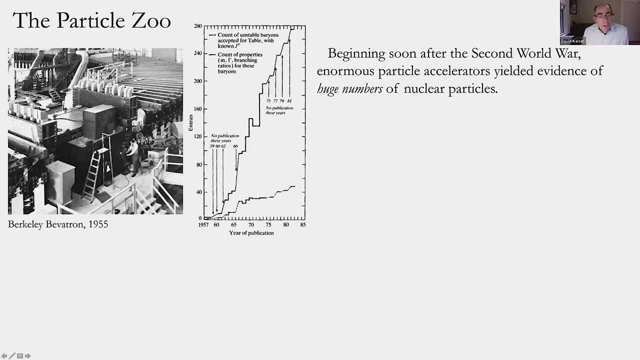 after the war pictures like this were becoming more and more common. so by 1955 berkeley's bevitron, a billion electron volt accelerator, was filling kind of factory room floors. again, here's a human operator to give you a sense of the scale: absolutely enormous. 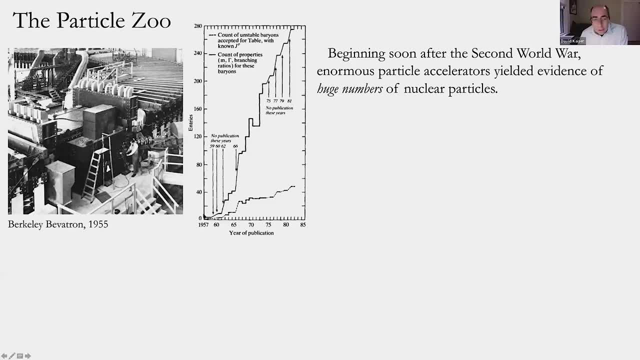 certainly for its time, and, as i mentioned, that that was driving this exponential rise in the numbers of seemingly new, seemingly elementary nuclear particles. uh, when physicists could achieve higher and higher interaction rates, they found not just higher energy stuff flying out, but new kinds of stuff flying out, and so that's what we're going to look at today. 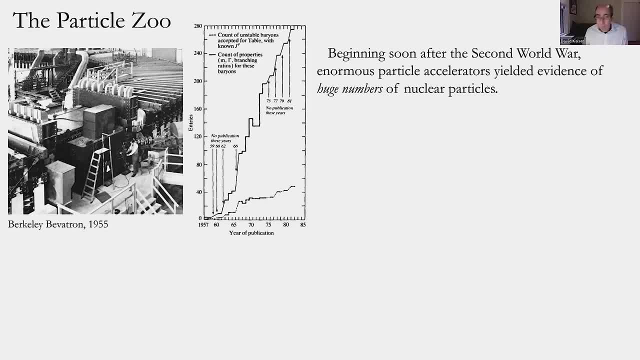 new kinds of particles among the decay chains and all that. so that was often called the particle zoo we saw in the previous class session. one of the first challenges, uh kind of intellectual challenges among uh to try to make sense of this very large number of nuclear particles, is that they 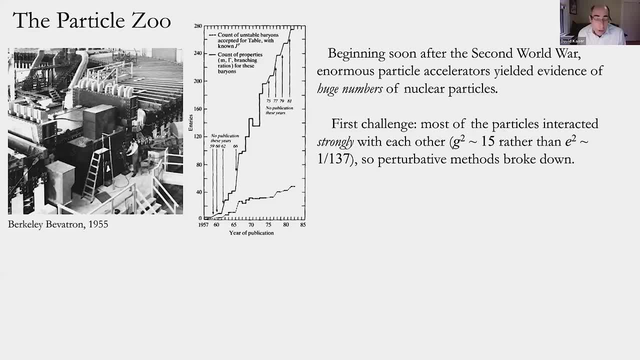 interacted strongly with each other. in fact, we now call this the strong nuclear force. uh, it's called strong because the, the, the analogy to the electric charge um, which we often abbreviate just by the letter g, the, the coupling constant is very big. so, whereas the electric 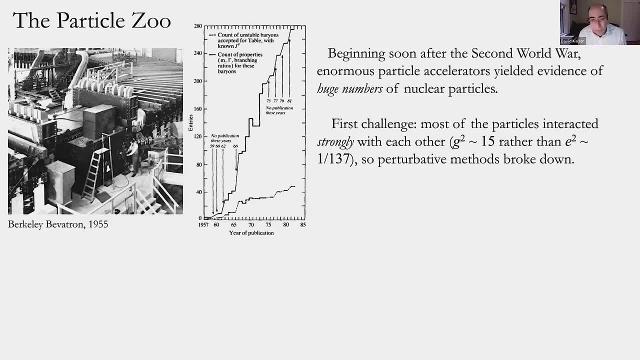 charge is small in kind of appropriate units it's roughly 1 over 137. so you could do a perturbation, expansion kind of tailor, expand and uh and more and more complicated contributions just count less because they have more and more factors of a small number in front. the opposite seemed to happen for 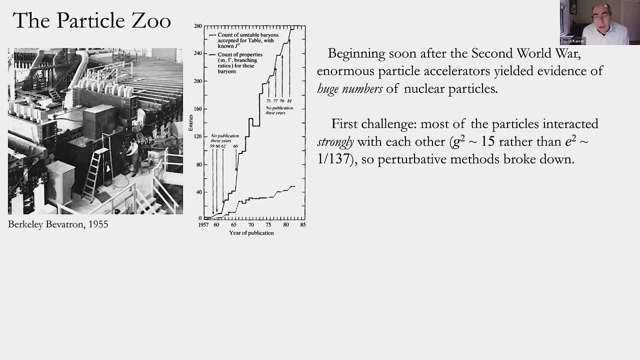 these strongly interacting nuclear particles where an arbitrarily complicated interaction of finding diagram with many, many vertices would actually weigh more in your final answer than the simple ones, and there was, in principle, an infinite number of complicated ones. it really didn't make any sense for how to calculate in this strong nuclear force regime. there was a second challenge. 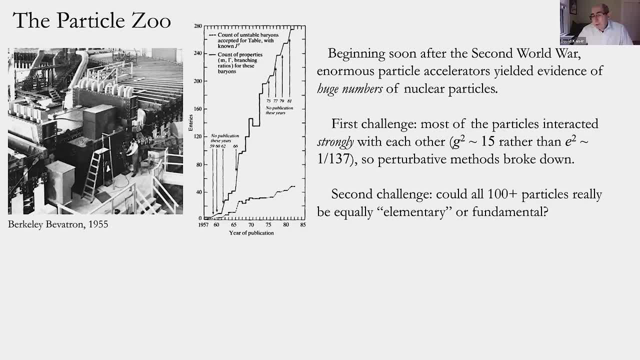 which was maybe a bit more meta, which was really this question of: could all these hundred or soon 200 or almost 300 seemingly elementary particles, are they all really elementary? are they all kind of to be understood on the same footing? uh, is there any pattern or any underlying kind of order? 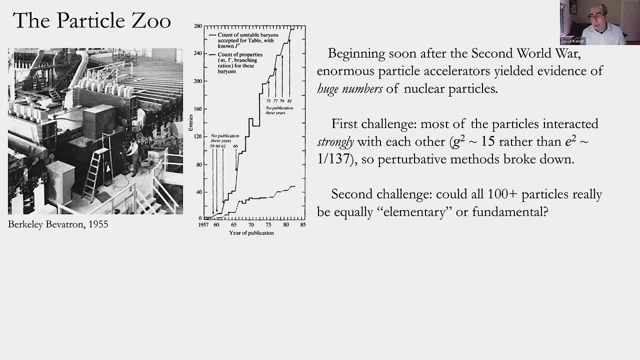 that one might be able to bring to what otherwise looked like, really just a kind of scatter shot, um display of soon hundreds, many hundreds of seemingly elementary particles. how do you make sense of all that, uh, all that stuff. so we saw just a brief recap for last time. one response: 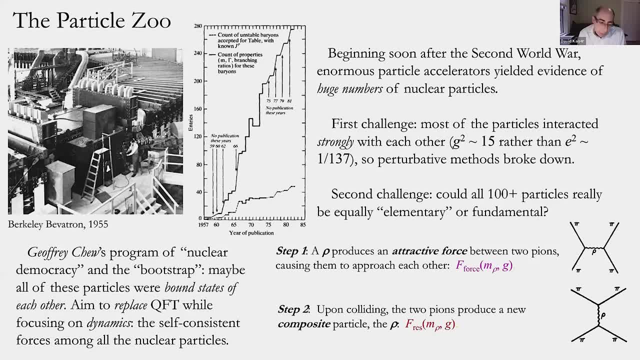 to this very creative response, which was really dominant for the better part of 15 years or so, was associated with the particle physicist jeffrey chu, and we talked a bit about him and read about some of his work. last time he introduced the idea of nuclear democracy and then, with some of his 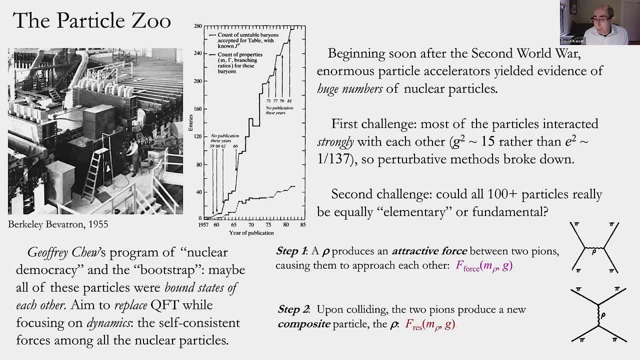 students the idea of the bootstrap, and they were really being very creative with, uh, these simple feinman diagrams where if you simply rotate the diagram, turn it on its head by, you know, by 90 degrees, then the roles that these particles seem to play could sort of swap. and so maybe 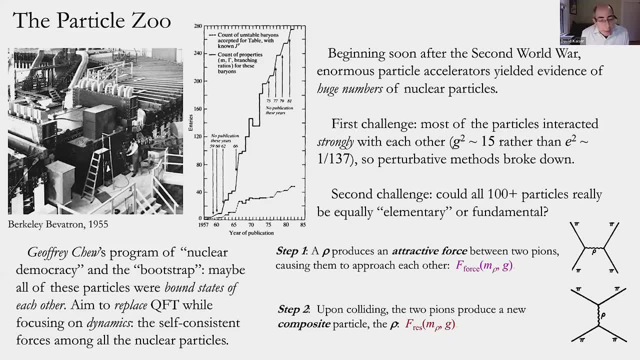 jik chu and his very active group. maybe, maybe they wondered that all these many hundreds of particles are actually in a sense, equally elementary because they're all bound states of each other, they're equally composite and equally elementary, and that the labels we apply to them really depend on which orientation of a kind of 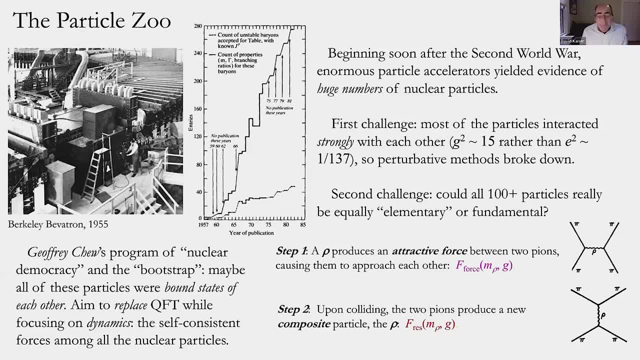 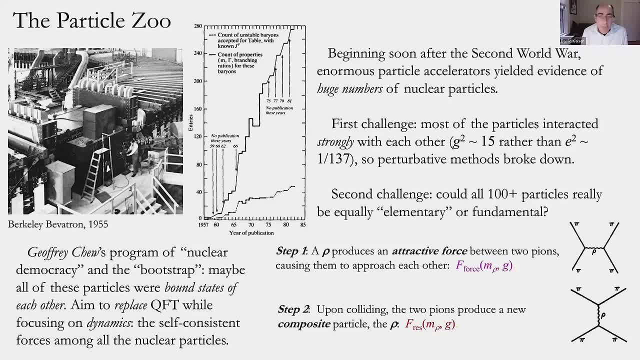 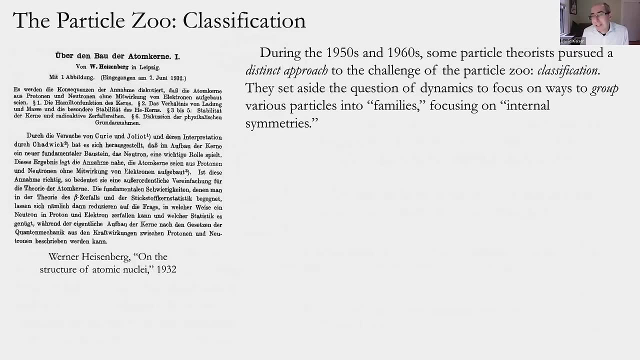 types of particles and their scatterings and interactions. so one of one response to the strongly coupled particle zoo was to look for a single kind of self-consistent bootstrap that might encompass more and more examples, uh, of this nuclear domain. so what we'll mostly talk about today is actually a distinct approach, a kind of- not even rival, but a complementary approach. 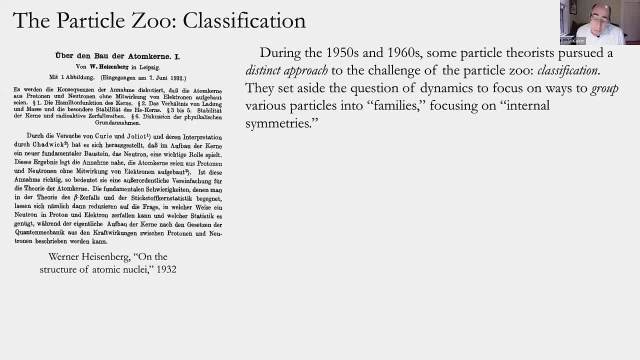 that started to gather more and more attention, uh, around the same time period during during the 1950s and 1960s, and that was to basically ignore- or kind of bracket for the time being- questions of forces or dynamics and just say that's beyond us right now, but focus instead on classification. 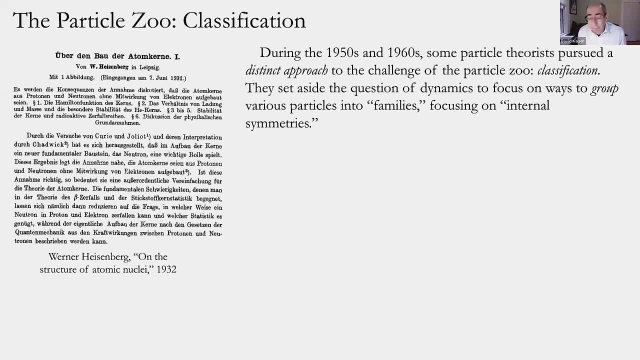 were there patterns among those dozens, and soon hundreds of nuclear particles that came out of the accelerators? was there? were some more like others, more like each other than and distinct from others? are there family groups? are there symmetries? are there are there ways to group, uh, this plethora? 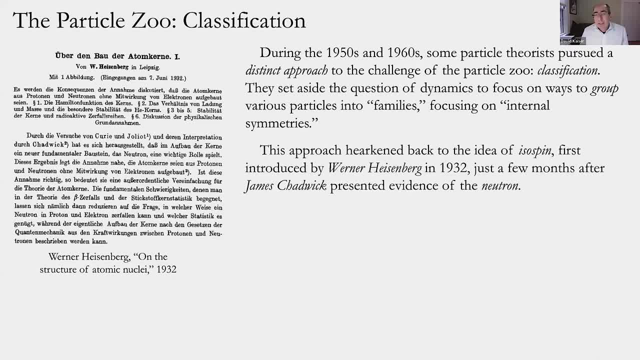 uh in in a kind of ordered fashion, so to classify. so in some sense that approach was really also not very new. as we'll see. it actually reached back to some ideas from the earliest days of nuclear physics in the early 1930s. one idea in particular i'll talk about now. uh was introduced by werner. 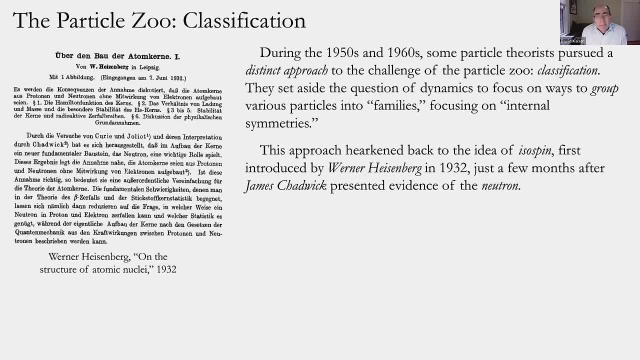 heisenberg as early as 1932.. uh, heisenberg, it was a series of articles under the title on the structure of atomic nuclei, the first of which was received in june of 1930 and was published in 1932. you may remember those. several weeks ago, james chadwick presented the. 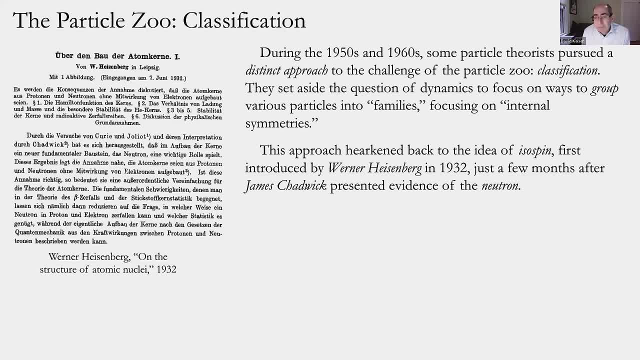 first really kind of compelling evidence that the neutron exists, that atomic nuclei might have more than one kind of particle within them, both protons and neutrons. he presented that evidence very early in 1932, january, february ish, pretty early in the in the year, within not even half a year later. 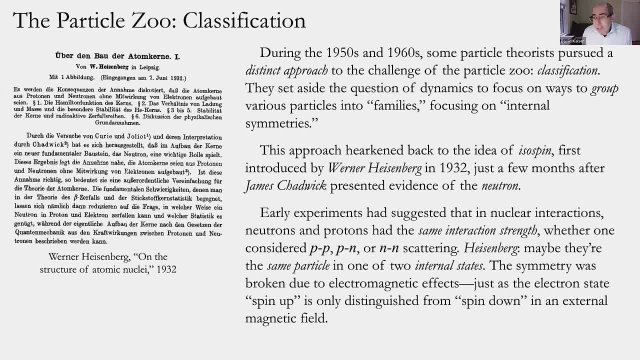 heisenberg had really picked up that idea and run with it and introduced this idea called isospin. so heisenberg had the early experiments with both protons and neutrons in these early months after chadwick had kind of isolated evidence for the neutron itself. the early follow-on experiments 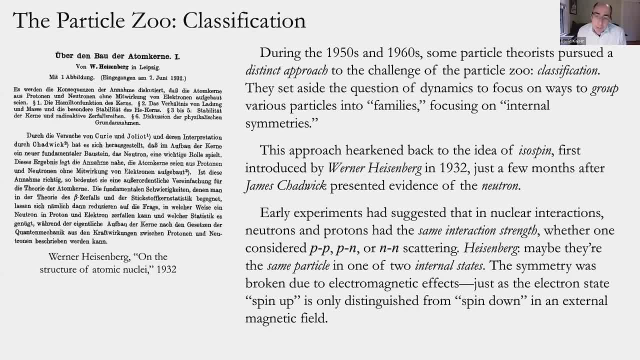 suggested that protons and neutrons were kind of interchangeable when it came to nuclear reactions, that they seemed to have, for example, the same scattering strength that that what would later be called the coupling constant g, the analog to their electric charge. it looked to be the same, so. 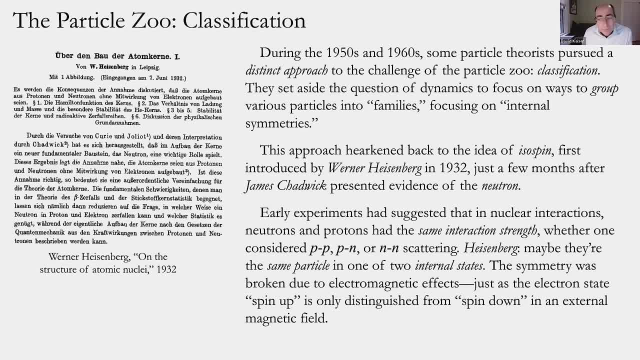 heisenberg had a very similar pattern to the electron scattering. so heisenberg had very similar patterns, reaction rates and so on. whether you were considering proton proton scattering, proton neutron scattering or neutron neutron scattering, it looked like it was just one kind of particle, not two very different seeming particles. there was a kind of symmetry in. 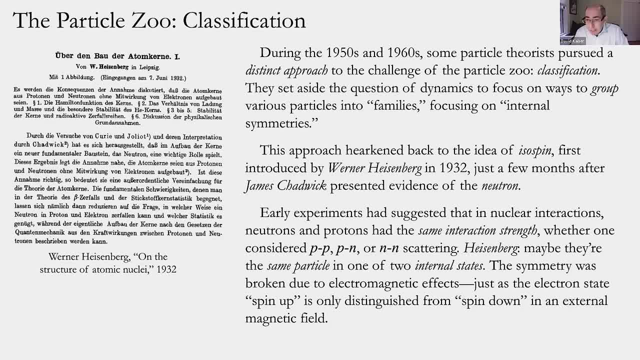 the way these particles were were experiencing the nuclear force. so heisenberg suggested in this series of papers back in in 1932 that maybe it's actually not two separate particles. after all, these are two separate particles and separately neutrons. maybe it was one kind of nuclear. 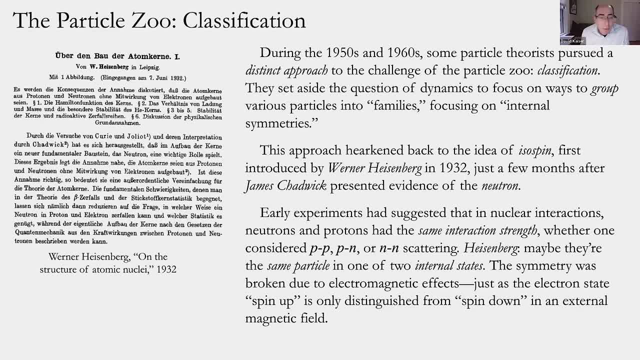 particle inside the atomic nuclei but it had different internal states and so be one particle that could be um in one kind of condition or another, but not actually different kinds of particles altogether, and that the symmetry- one particle, uh, that could show up as either proton or neutron, that symmetry would be broken. we would notice the difference when we put those particles. 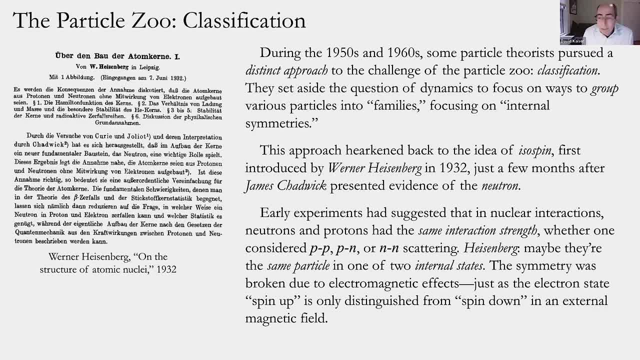 in external electromagnetic fields. we'd see quite obviously, for example, that the proton has one unit of positive electric charge, whereas the neutron is electrically neutral. but we only notice that if we're measuring electromagnetic effects, if we're putting these, these particles, in an external field. so heisenberg. 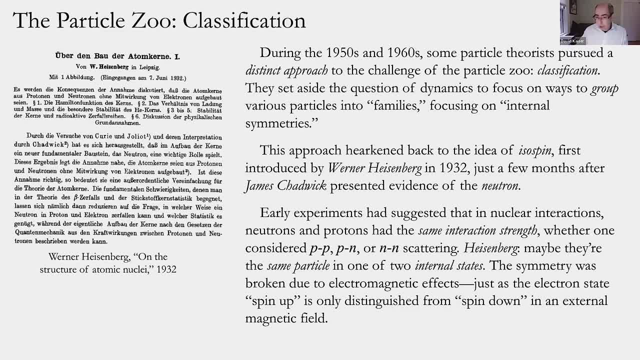 said that could be just like an electron, which could be either spin up or spin down. its internal angular momentum could be spin up or spin down along some direction of space. but we'd only notice that if we put that electron in some external magnetic field like a shtern gerlach um device. so it's. we don't say there's two separate electrons, we'd say there's. 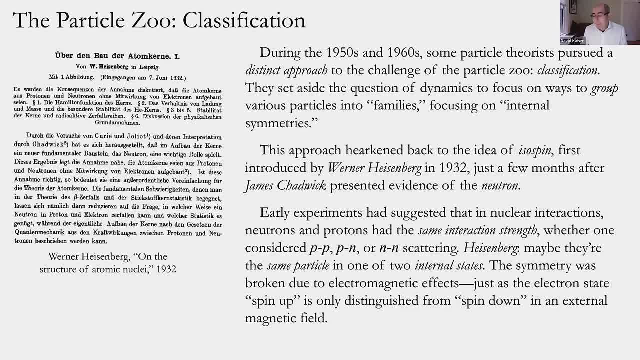 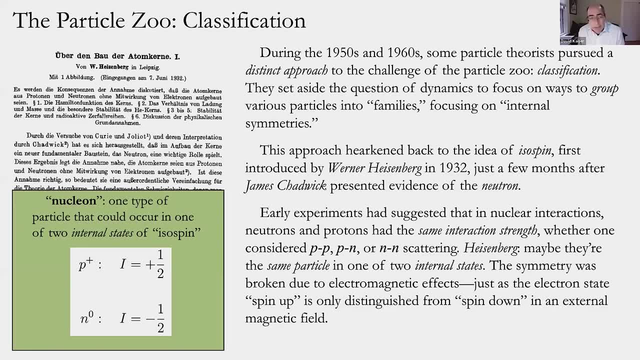 one electron that could be one of two internal states. heisenberg was saying maybe these nuclear particles were similar. so uh, maybe it's not protons versus neutrons, maybe there's one kind of particle. after the war it became common to call that single type of particle the nucleon. 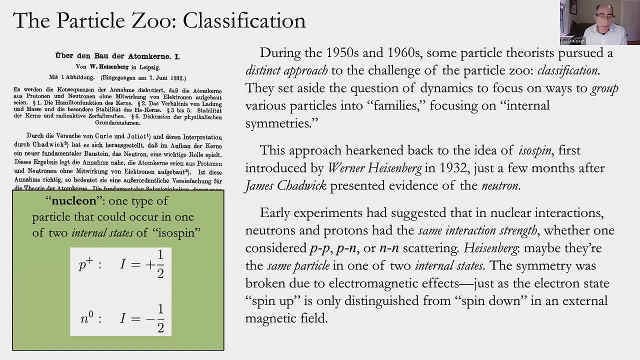 which could manifest as either a proton or a neutron, depending on its internal state. but they weren't. uh, it was. one could imagine them as not being literally separate or distinct particles, so there's a kind of internal symmetry. uh, they would be distinguished by a new quantum. 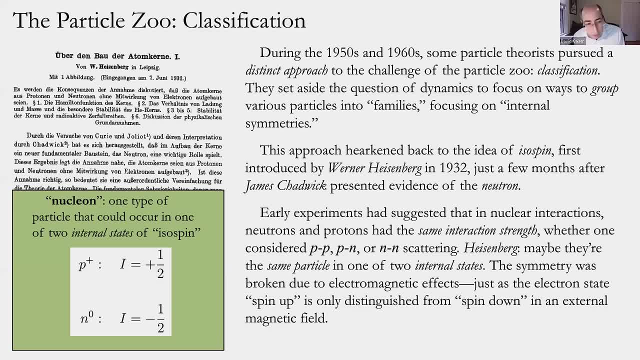 number, not the same set that people have been thinking about through the 20s. an additional way to characterize that state called isospin and the proton. we would assign to say uh plus you know, one unit of isospin and the neutron would be uh sort of isospin down. but maybe they're just. 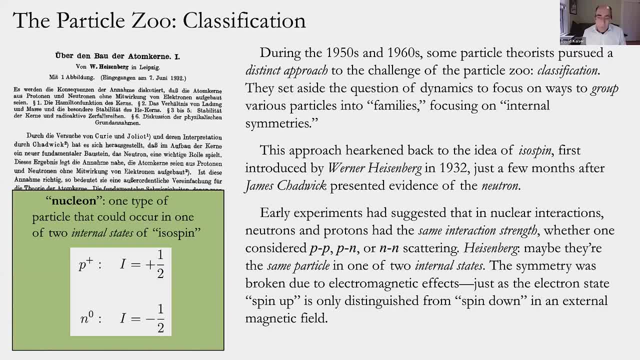 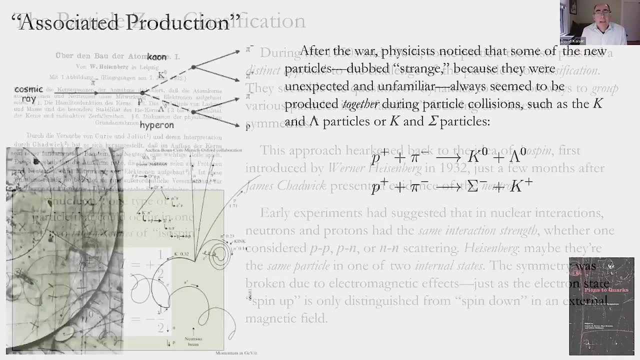 internal states of a single nucleon. so that was the idea that heisenberg suggested very creatively in the earliest days of nuclear physics and a lot, and after the second world war a number of theorists kind of went back to that and said: let's, let's look at that again, let's maybe take that a bit more seriously, because there were 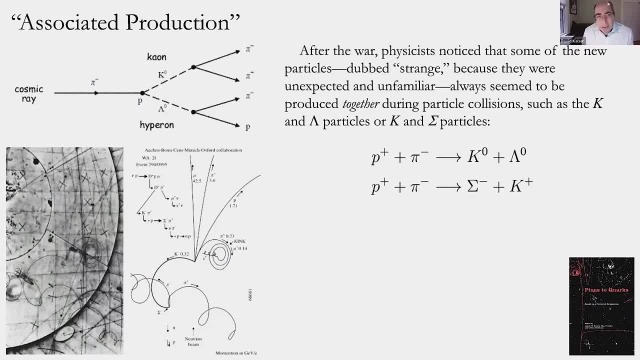 now many, many more particles to try to to sift through and make sense of. so one of the first patterns that a few physicists began to notice soon after the second world war was that certain of these new particles- they were often dubbed strange because they were unexpected or unfamiliar. these strange 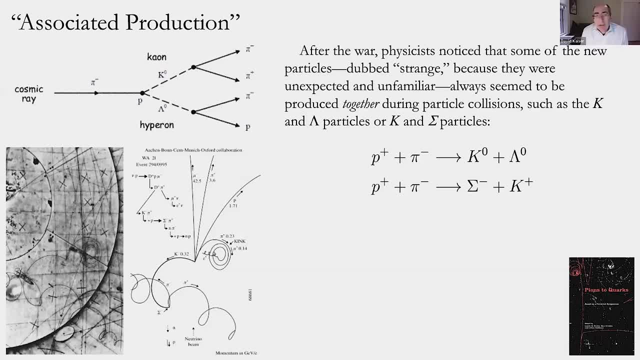 particles didn't show up sort of one at a time. they seemed to come in pairs, they seemed to come together. this became known as associated production. they were produced in particle scatterings in association with each other. it's a fancy way of saying you didn't get only one of these strange. 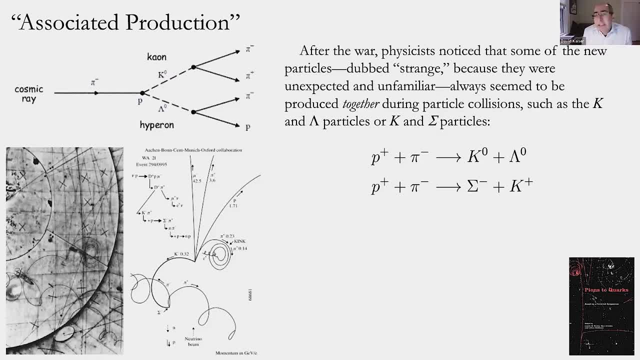 particles, they seem to come often in pairs, and so the idea then was: i could, could one, assign to these chambers day-by-day experiments and use these human molecules to make sense of these patterns. and so then again on yet another internal quantum number, not isospin, but a whole new kind of charge or or quantum quantity, and so uh. 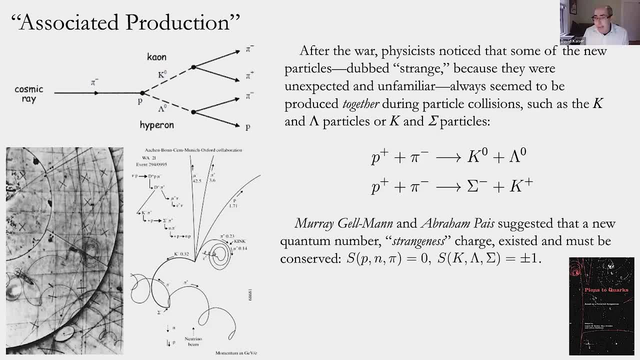 independently murray gelmon, who was a very young particle theorist at the time, and avram pious, a little bit older, still pretty young in his career. they separately came up with the idea that maybe to make sense of these patterns, that these sigma particles were produced with kaons but not separate from these kind of other strange 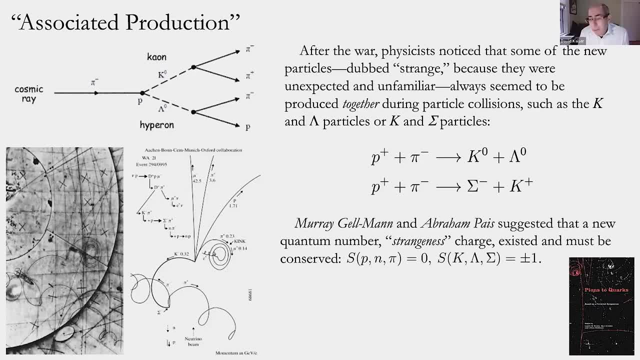 particles. Maybe there's a kind of charge called strangeness, and some particles were strangeness neutral, like the familiar proton, neutron and pion, whereas other particles carried one or minus one units of strangeness. and strangeness had to be conserved, And so it was. 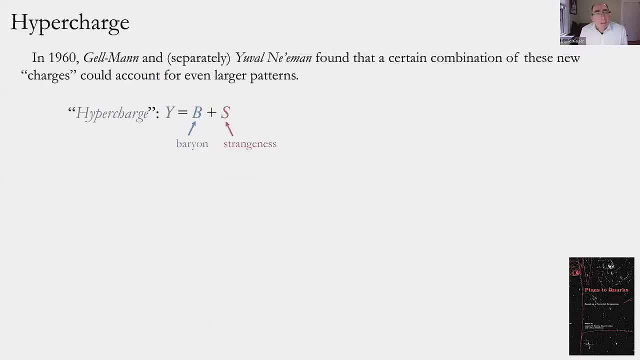 out of the way to make sense of these patterns. And so, a few years after that, a better part of a decade after that, Gelman, and then again separately, in this case a theorist based in Israel named Yuval Neyman. in 1960, they separately introduced a new way to try to account for these. 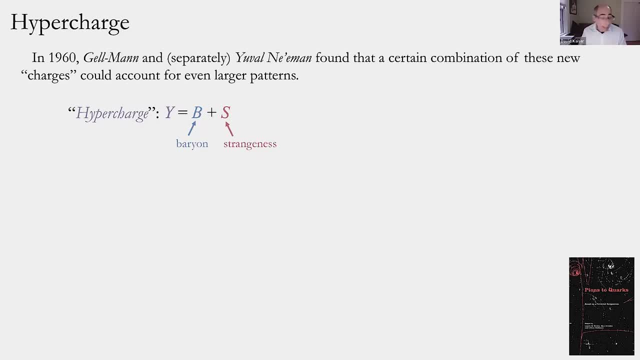 kind of patterns? Remember that no one yet is talking about forces or decay rates. They're really just trying to say: is there a kind of pattern to this very large number of new particles? Are there new ways to make sense of why some particles seem to appear with others? 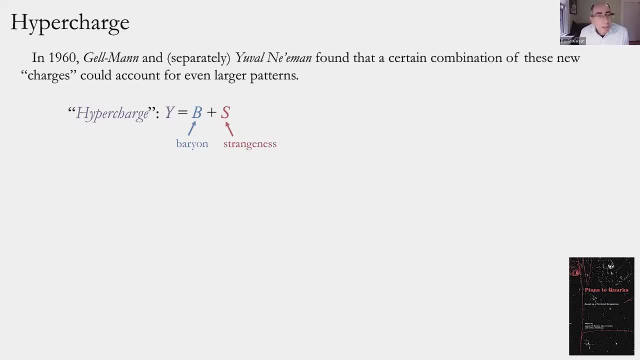 in these patterns. So they introduced something that came to be called hypercharge. So take a couple of these as yet entirely hypothetical internal quantum numbers. They just keep inventing new ones to see. would that help us sort what goes with what One of them they called baryon number? 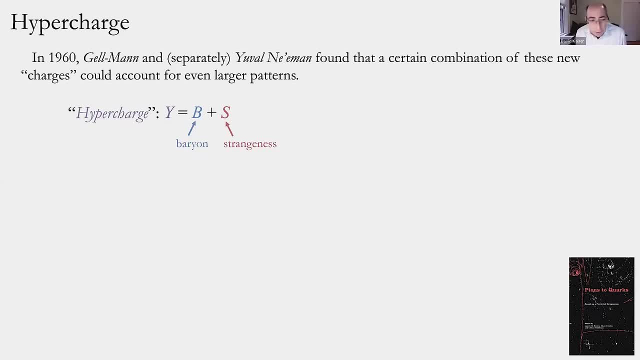 and that applied to many familiar particles like protons and neutrons. It would also apply to many of these new strange particles. So one kind of charge would be baryon number or baryon charge. Some of those particles would also carry this so-called strangeness charge. So the hyperon. 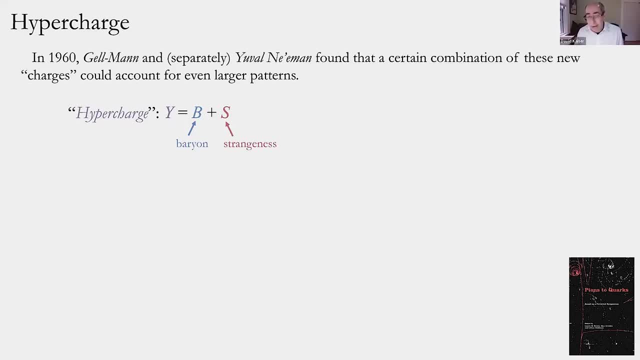 particles or the sigma particles, would have one unit of baryon charge and one unit of strangeness charge, whereas the more familiar, the not strange baryons would have one unit of baryon charge but zero units of strangeness that kind of thing. So it's a new way to try to sort out this large 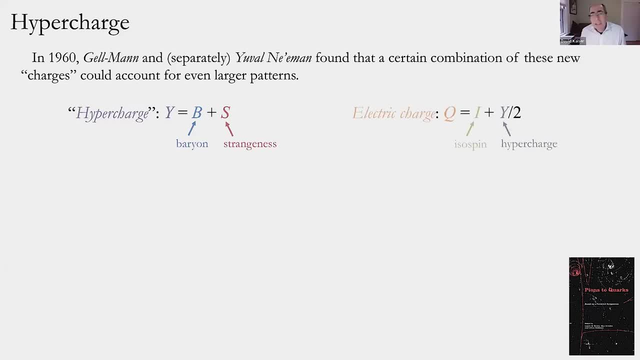 kind of Sudoku puzzle of new particles. And then again Gelman and Neyman showed in 1960, if you pick up on Heisenberg's notion of isospin as internal state, that could distinguish, for example, a proton from a neutron and then add in one half of the hypercharge, this new one. 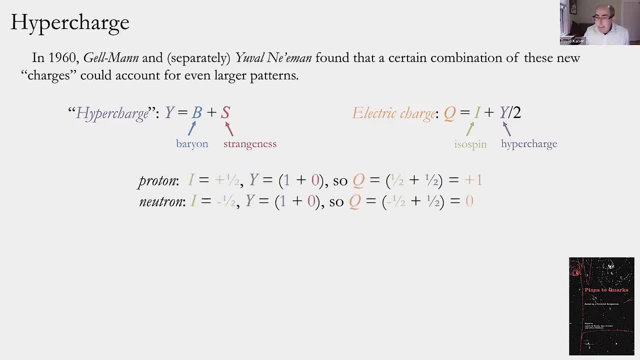 they had just basically made up, then you could again start making kind of sense of these patterns, of these particles. So if you go back to the familiar nucleons, the proton, according to Heisenberg we could assign it as this isospin upstate, So it's isospin ispotent. 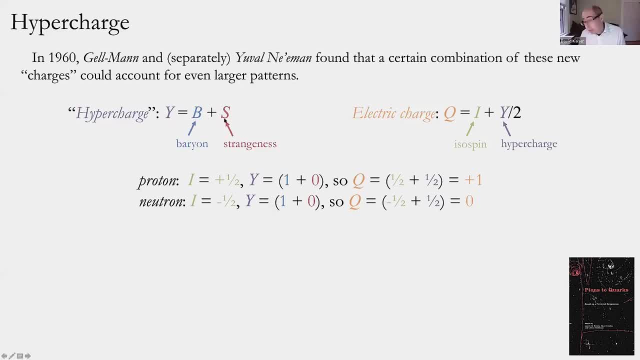 plus one half. It has one unit of baryon charge, but it's not strange, So it's hypercharge is plus one. Plug in over here, you see. well then you'd expect in the appropriate units it should have. 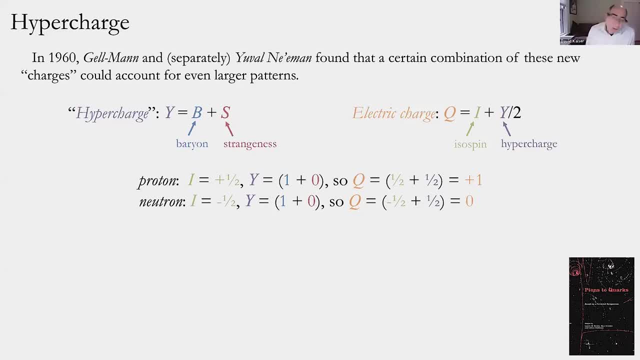 one positive unit of electric charge. Conversely, the other state of that nucleon, the neutron, would be an isospin down state. It also has one unit of baryon charge, but no zero strangeness, And so you'd expect it to be electrically neutral, And then you can play that game. 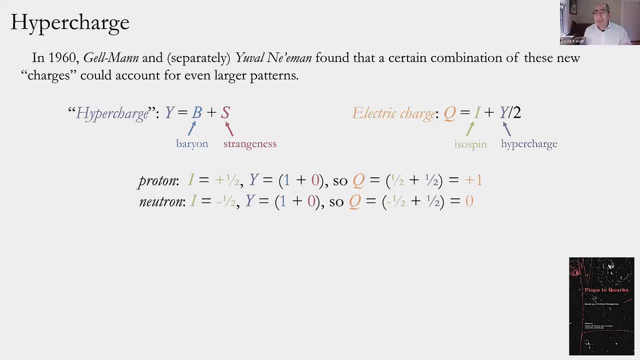 dozens and dozens of more times to see. is there a kind of single, self-consistent pattern with which you could start grouping like with like among the even less familiar particles, not just protons and neutrons. And so, in 1960, Gelman presented these groupings. 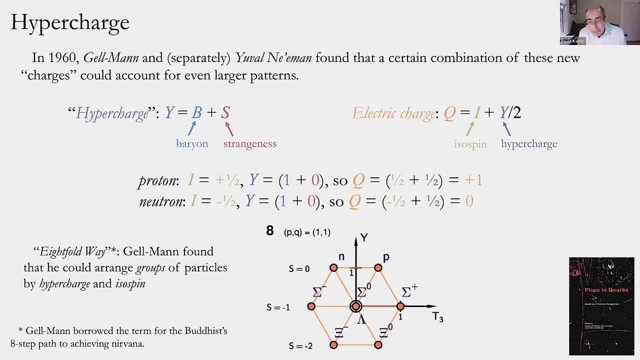 these group theory structures that seem to make sense of families of particles, And he could array them by mapping them along two axes of hypercharge, this new internal quantum number he'd invented. So hypercharge versus isospin as opposed to other ways. one 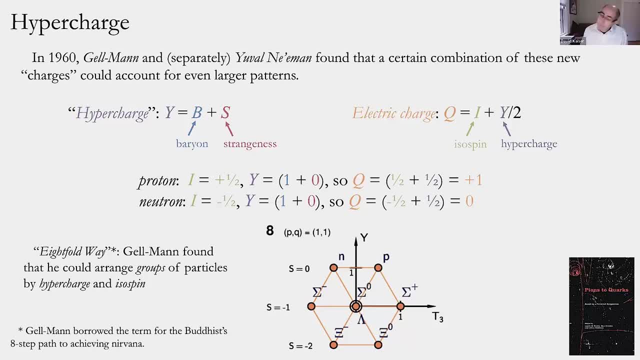 might try to group particles, electric charge and mass, and like that He was finding order by placing them in this abstract kind of mathematical spaces, grouping them based on their hypercharge and isospin. And he found these very distinct patterns, Some of them, 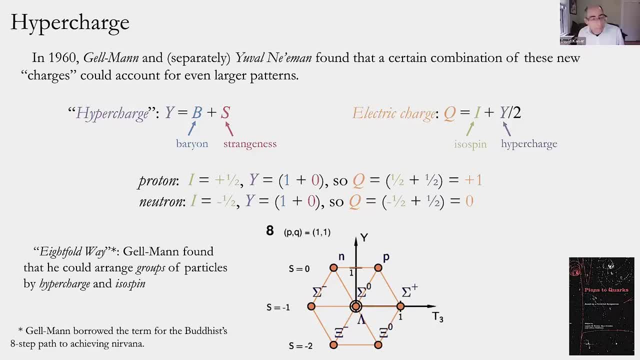 were eightfold patterns, others were tenfold or decouplets, So he labeled this first one the eightfold way. He was being very playful, Actually he was just kind of showing off. Gelman loved to the very end of his life. He only died a few years ago. He lived quite a long life. He loved showing off. 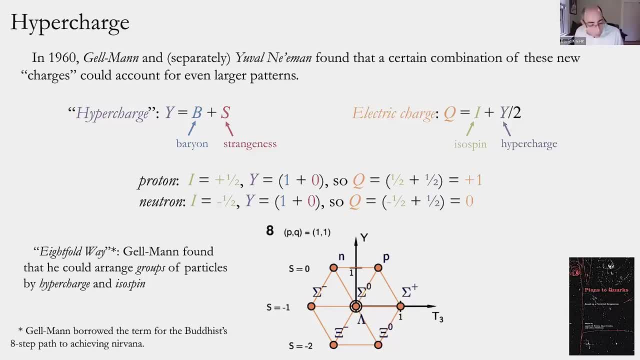 his knowledge of many languages, many literatures and cultures of the world. We'll see more examples of that even today. So he very playfully borrowed the term for this from the Buddhist's eight-step path to achieving nirvana, which for a long, long time had been known in English translation. 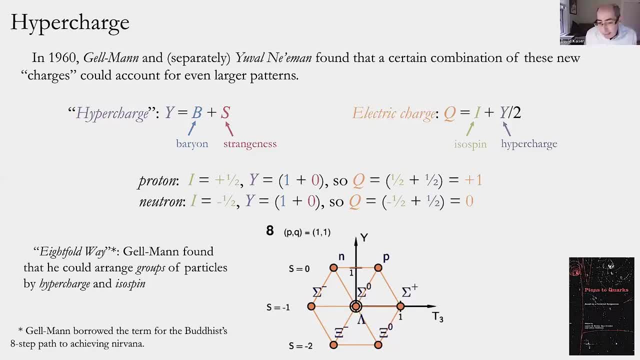 at least as the eightfold way. Gelman said. that's just as important or just as evocative a term for these eight-fold particle groupings he was finding when he mapped some of these nuclear particles in hypercharged isospin space. So here the familiar neutron and proton. they have 0 strangeness charge. 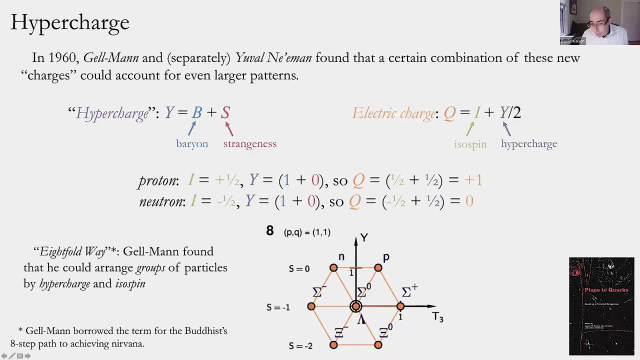 they're not strange because they've been known for a while. Here are the sigma particles. here's the neutral hyperon. here are other particles with 2 units of strangeness charge instead of one. So he called that the eightfold way. 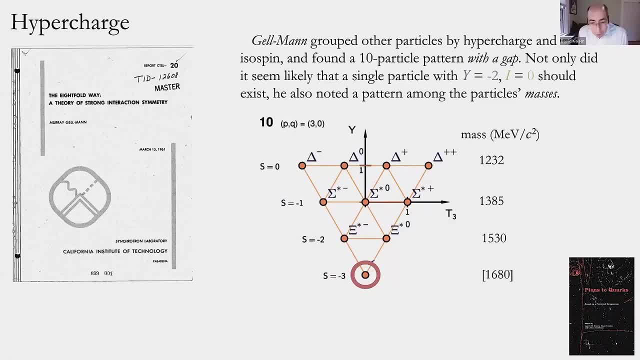 He went on to show there are other groupings, other very specific group theoretic structures, again in this abstract hypercharge isospin plane which no one in their right mind otherwise would have thought to use. But there were sometimes not just eightfold patterns but tenfold decouplets. 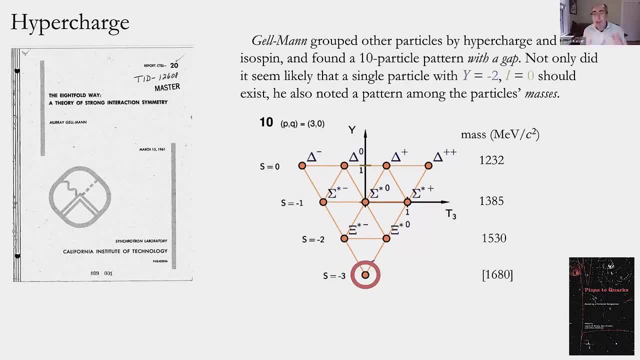 Again of particles that seem to be kind of associated with each other based on their varying hypercharge and isospin, And this involves again some of the both unstrained and strange particles. So the delta particles seem to have zero strangeness. 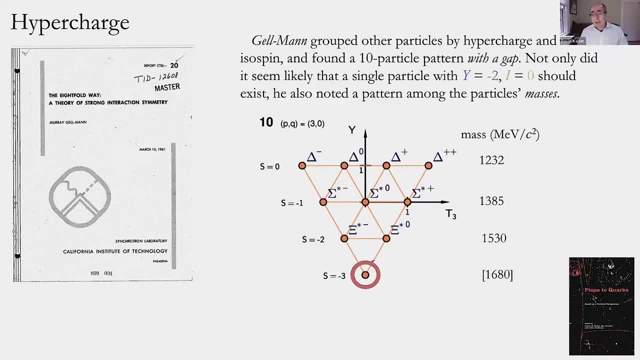 That meant they weren't subject to that associated production. You didn't have to make a separate strange particle with them. so they seem to not carry conserved strangeness charge. Here are the sigmas, the cascades and so on What he pointed out. 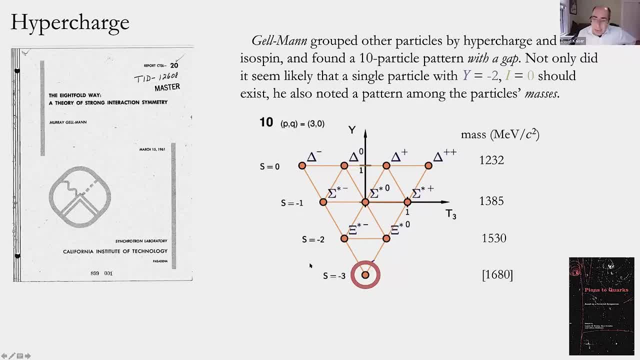 This time was that there seemed to be such a pristine geometrical pattern and yet a gap. There was a missing and as yet unknown particle that Gelman suggested maybe really is out there after all, To fill out this very clear pattern. he thought maybe there should be a particle with minus two units of hypercharge but zero units of isospin. 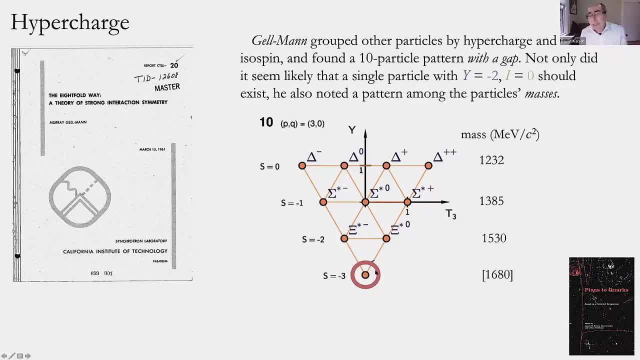 That red circle here, the kind of gap it has otherwise very clear mapping. Moreover, for this particular example, there was a missing particle. There was a missing particle. However, for this decouplet, he went further and found that there was a kind of pattern in the masses between these rows as you went down in hypercharge. 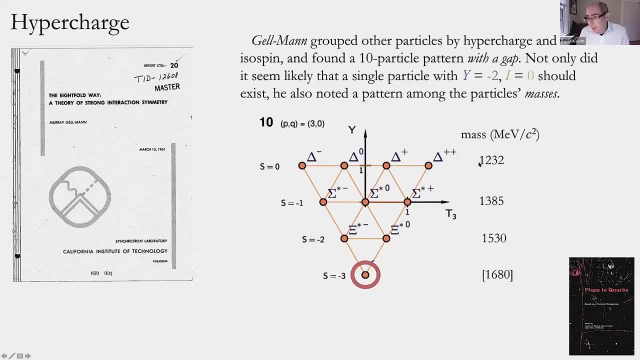 So the delta particles all had a mass of roughly 1,200 million electron volts, whereas the sigma particles had around 1,380, a gap of roughly 150 MeV. The cascade particles were another 150 MeV heavier still, So Gelman went even further. 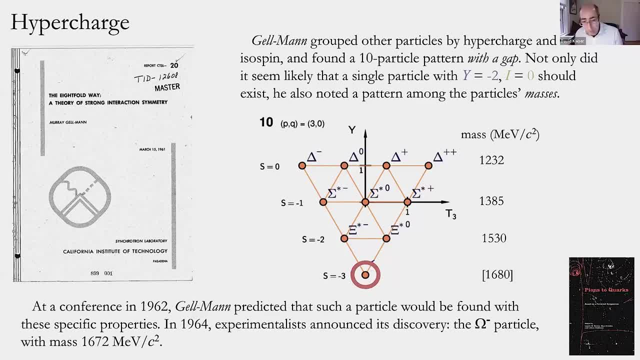 In fact, very dramatically, in the middle of the conference with a number of experimental physicists in 1962, he basically stood up and challenged them. He said: I bet if you look hard enough you'll find a particle with exactly these properties. 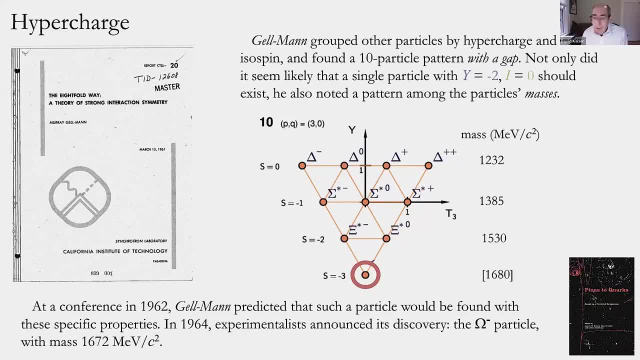 With hypercharge minus two, isospin zero. he could then work out it should have one unit of minus electric charge and he could even give a mass estimate. He said it would probably be about 150 MeV heavier than the cascades and, sure enough, about not quite two years. 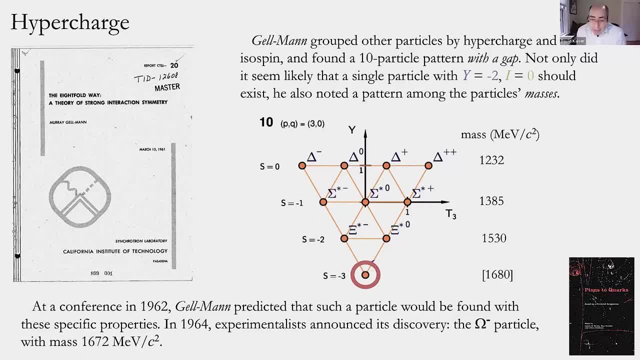 But two years later experimentalists came back and announced that they had actually found evidence for exactly that particle, almost exactly with the properties that Gelman had very dramatically predicted. The mass was extraordinarily close to Gelman's kind of back of the envelope estimate. 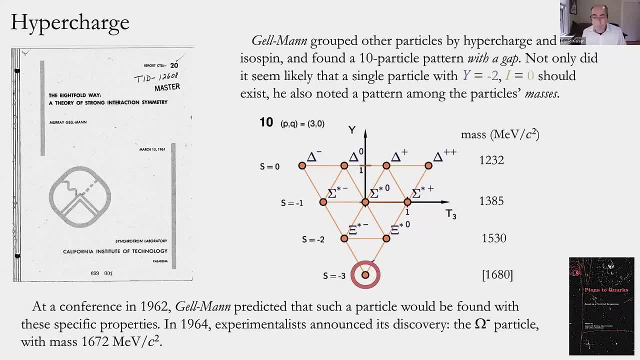 It had indeed one unit of negative electric charge. It seemed to be consistent with the strangeness of minus three and so on, The so-called omega minus particle. That was a big big deal. In fact, it was such a big deal that Gelman was awarded the Nobel Prize only five years later. 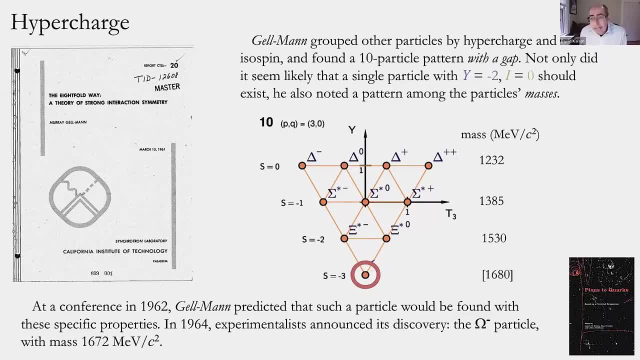 In fact it was such a big deal that Gelman was awarded the Nobel Prize only five years later for all of these efforts to bring a kind of classification order to what it seemed like an orderless, just this kind of sludge of new particles. this kind of development impressed many of his colleagues very, very quickly, in real time. 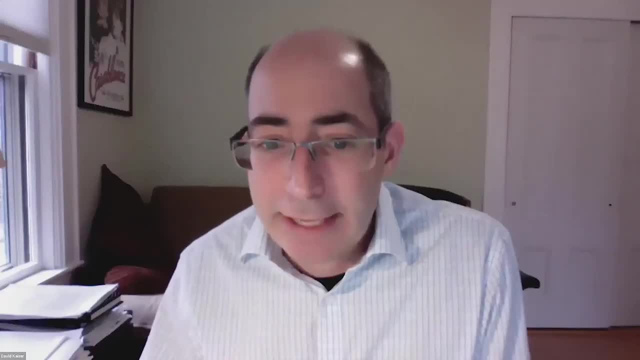 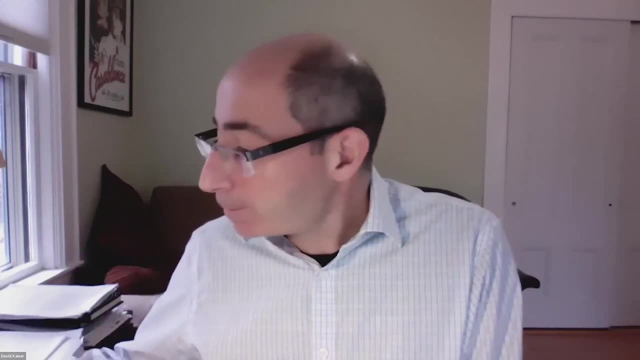 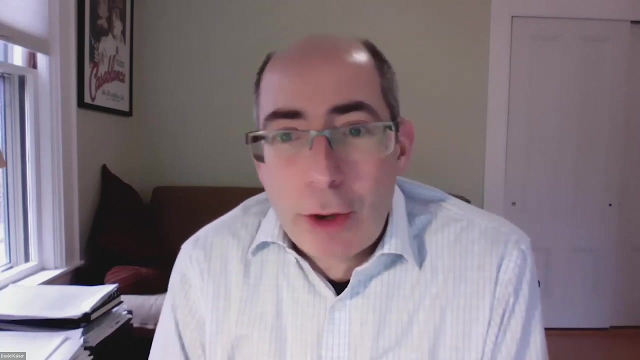 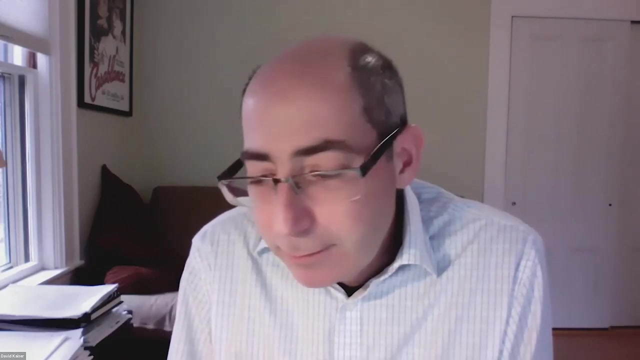 So let me pause there and ask if there are any questions on that classification approach. I really find it astonishing. I don't have any fans of puzzles like Sudoku or they're like highly constrained. You can go here, but not there kinds of pencil and paper puzzles like a, like a crossword puzzle. 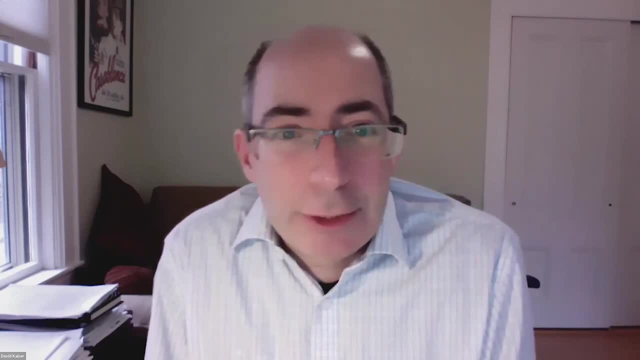 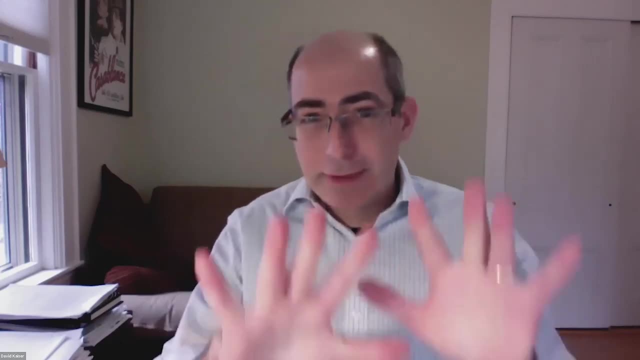 But he's doing that now with, with you know, 300 seemingly elementary nuclear particles and finding- I think he's very abstract, or at least not not the most obvious properties to focus on, but he just sort of rearrange things, then began finding order where. 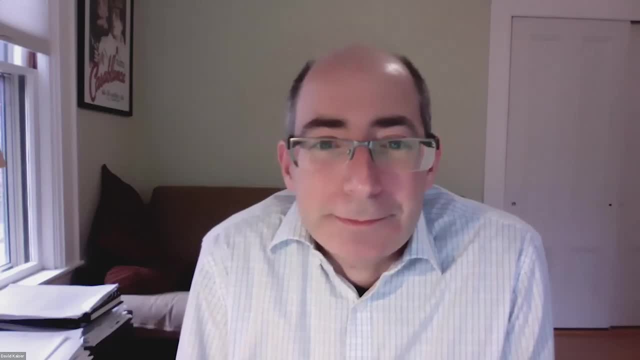 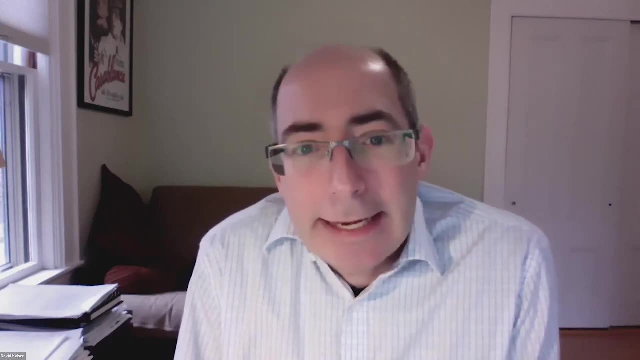 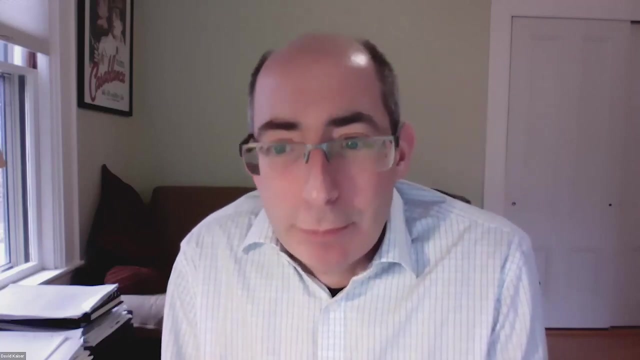 where where few had found it before. So it's pretty cool, I should say. Galman did his PhD at MIT, so we should be proud of him for that. I guess local fella He had been in grad school in I think he finished in 1951. so this is some work he was doing pretty soon after his PhD. 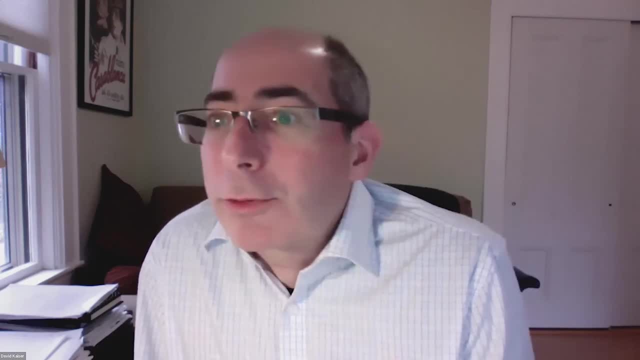 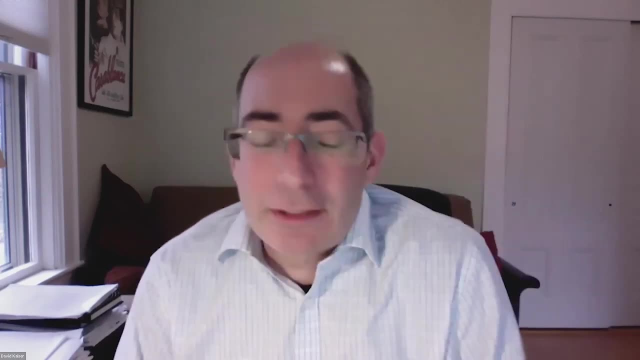 Any other questions? if not, I'm happy to press on. Here's a question from Tiffany. Oh, yes, right, so That's true. Who might know- Some of you might know- Sabine Hassenfeld. Who might know who? Sabine Hassenfeld? 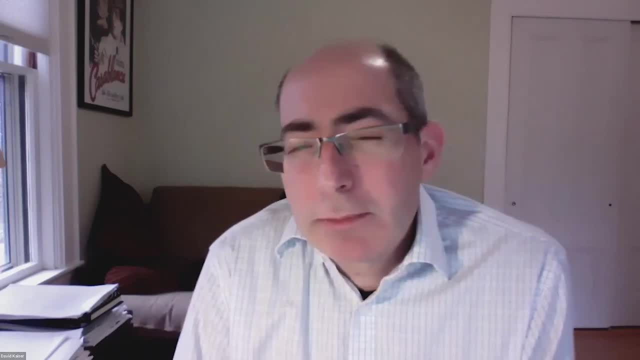 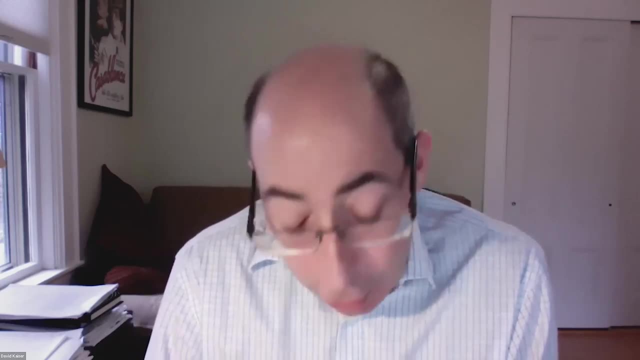 a colleague of mine. i know something pretty well. she wrote a really interesting popular book about a year or two ago- not too not too long ago- called uh lost in math um, and she's become a really outspoken, very trenchant and outspoken critic of developments like um string theory in high energy. 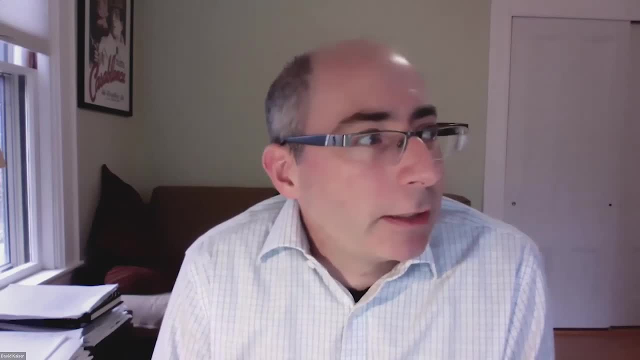 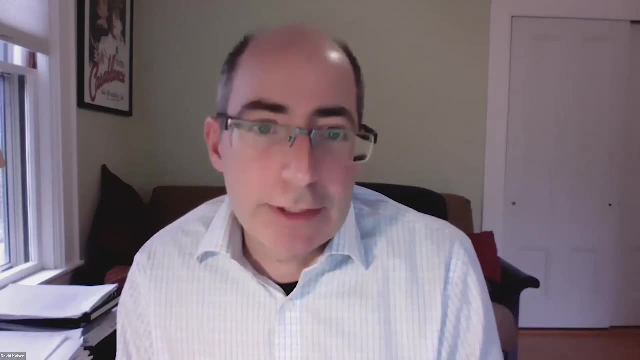 uh, physics. and so her argument, uh, in brief, um, is that sometimes, in more recent years, physicists have maybe become too enamored of these kind of symmetry arguments that just because there's a pattern, that nature must have taken advantage of what we consider a beautiful symmetrical pattern. 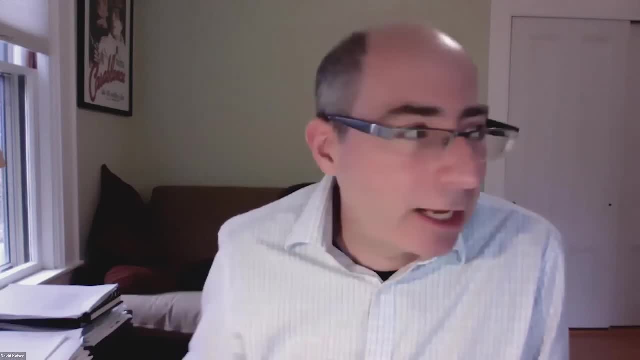 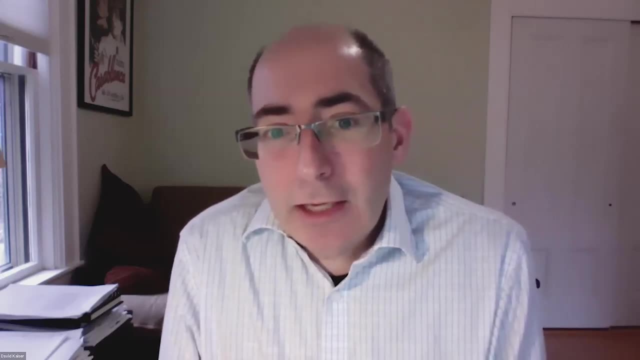 and could we have a little more input than that? i should say back in gelman's day, the early part of his career, he could make an announcement in 1962 with real confidence that his colleagues could. he could actually try to find empirical evidence that was consistent with it. 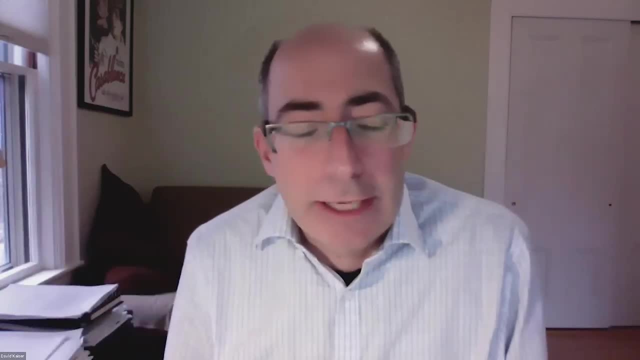 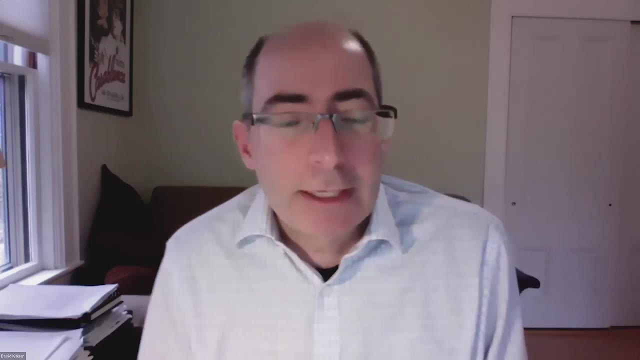 within a short while, let alone 50 years later, and so the the kind of symmetry argument was getting a lot of feedback, let's say positive reinforcement in the 60s, because these experiments were feasible in many, many places, could do it and and it actually wasn't. 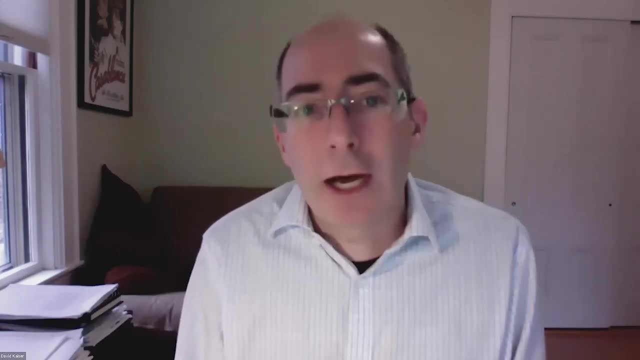 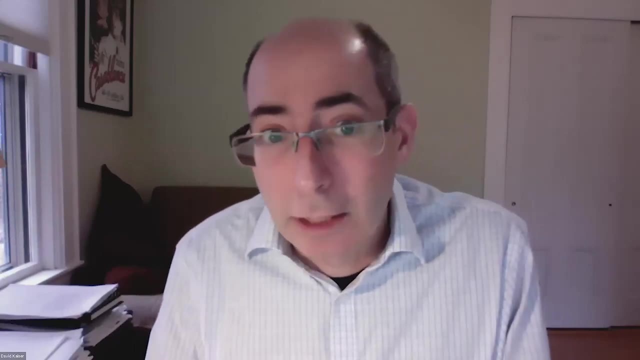 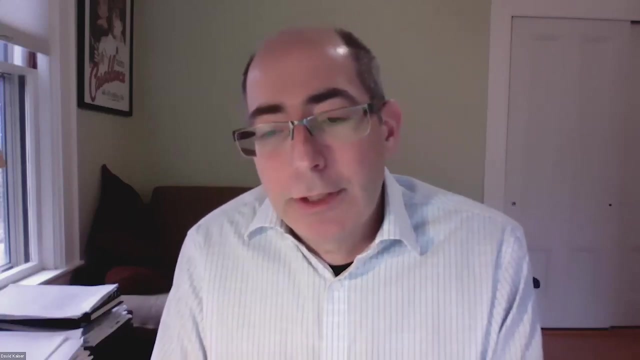 um, it wasn't a kind of uh wasn't based only on mathematical um beauty, but a kind of pattern that maybe one could then have a kind of empirical dialogue about. and i think sabine's point, quite well taken, is that more recently, uh, the energy scales involved in the hypothetical string theories. 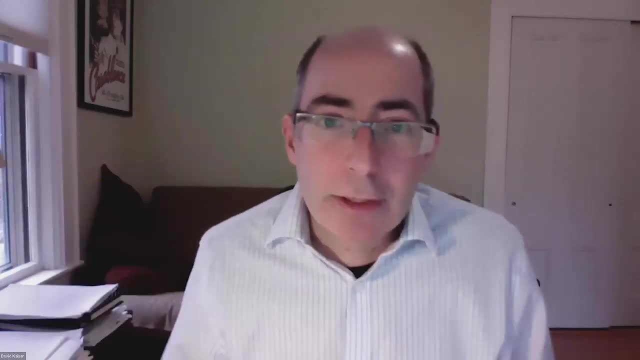 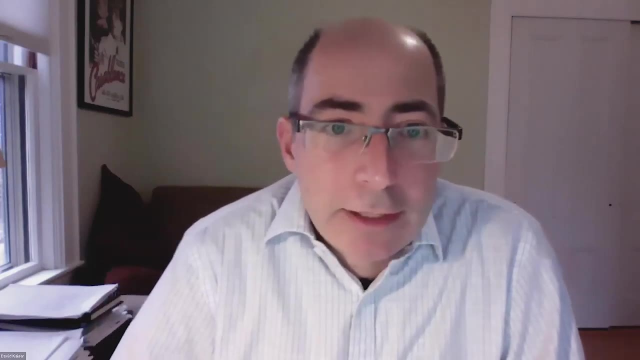 and so on, are so far removed from earthbound experiments that we've lost that kind of back and forth- uh um, kind of conversation, so to speak, between theory and experiment and a lot of these ideas, so that the what seems to some people like beautiful mathematics seems to others like groundless. 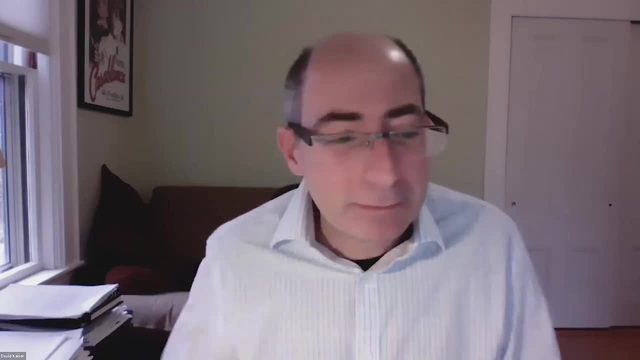 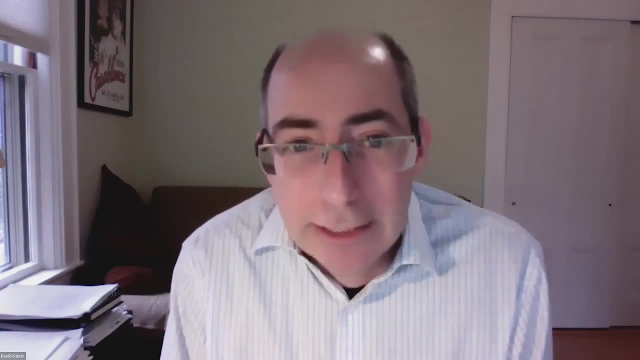 speculation, uh, and that seems to be a different situation than in the mid 60s. so she's a very good writer, i mean she's i i think she's a great kind of popular science writer anyway, let alone that she has, i think, really interesting insights into, um, some of the sociology of more recent 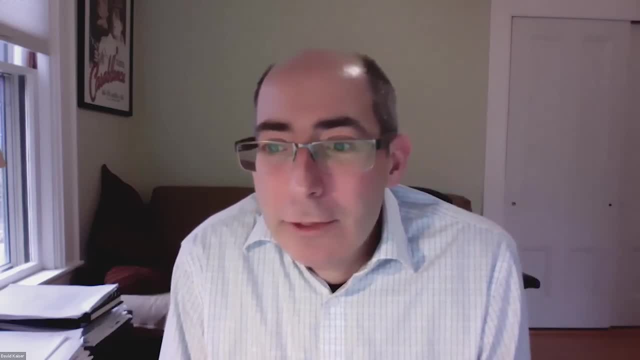 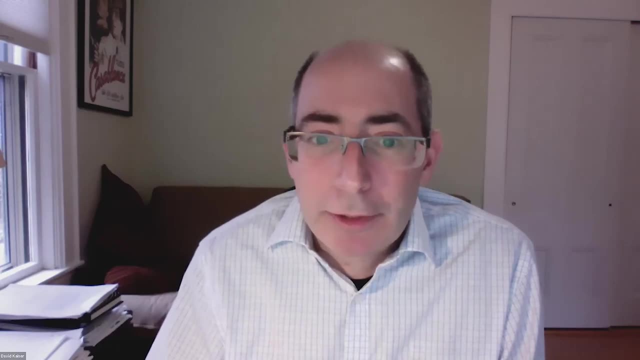 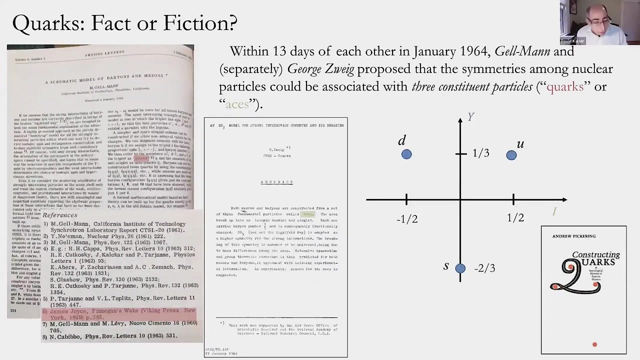 theory. yeah good, any other questions or comments? if not, i'll i'll jump into the next part, okay? well, let's see what people do with all this crazy, uh, symmetry stuff. so i mentioned that in 1962 gelman made this kind of great, very dramatic prediction at a. 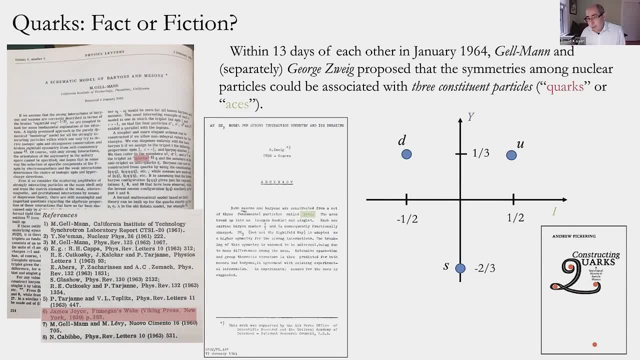 conference saying: go look for the omega minus, right where i told you to look for it. essentially. not long after that, uh, very early in calendar year 1964, gelman, and then again independently, another younger, much younger theorist, george zweig, separately suggested, proposed a new 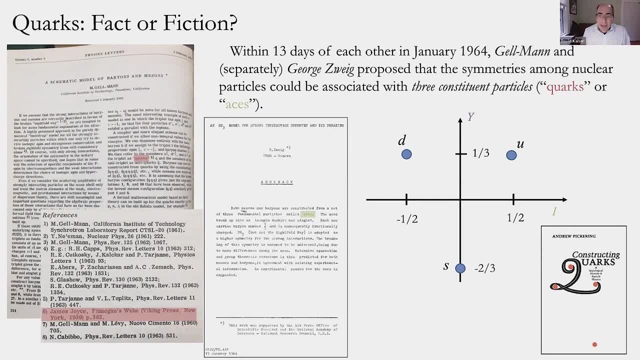 hypothetical way to bring order to these kind of hypercharged isospin groupings that gelman, by this point, had been doing for quite a while. so gelman's article was received at the journal you can see here, received on the 4th of january 1964. it was published three and a half weeks later. it was 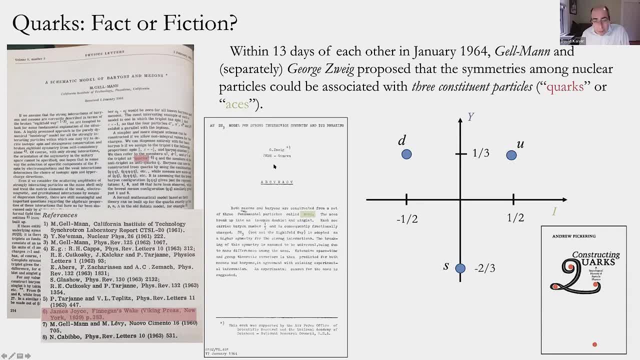 pretty quick to get through peer review. uh, george zweig's pre-print from cern. he was at that point a very new postdoc at cern. his pre-print was dated the 17th of january 1964. so they were working separately and not even two whole weeks elapsed between each of them committing this to. 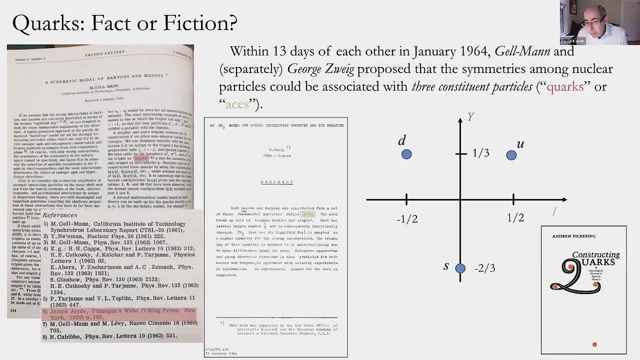 paper and they they came up with a remarkably similar set of ideas. that may be actually the order of that gelman and you've all name on and others have been finding for a couple years eightfold away, and the 10, the decouplets and so on. maybe that was due to an even more deeper 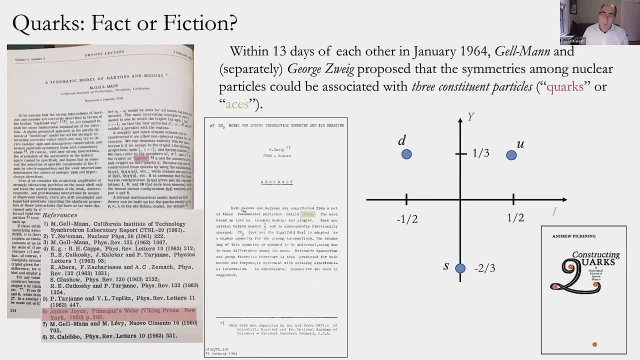 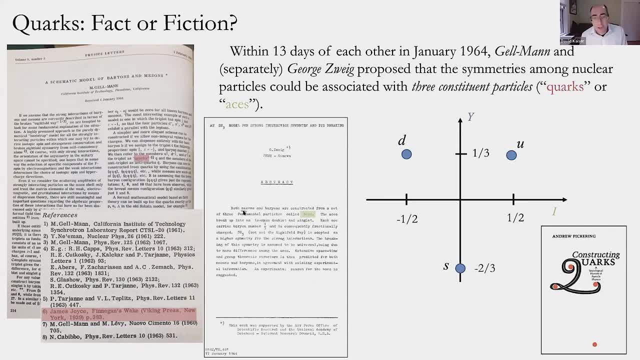 page of his. it was only a two-page article. uh, zweig had called them aces. these were really very, very similar ideas and they did all the patterns on these hypercharged isospin plots among the known, the then known nuclear particles could be reproduced under a very simple sounding. 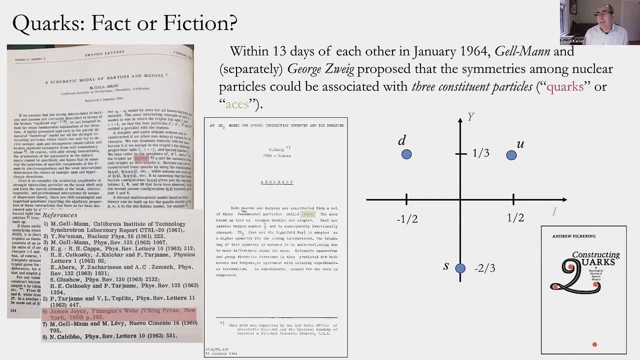 assumption there that there existed only three types of elementary constituents, quarks or aces, and if you were very careful in assigning them very specific values for hypercharge, isospin, strangeness and all the rest um, that you could reproduce those group theory patterns of uh. 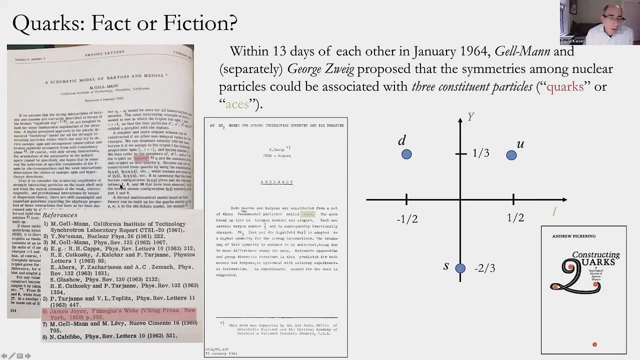 eightfold patterns and tenfold patterns. so gelman, as i mentioned earlier, loved to show off his, his wide-ranging knowledge of languages and literature and so on. so among this very short list, this is the entire references list. eight references only for this entire two-page article, number six of which is to james joyce's, a very famous and famously. 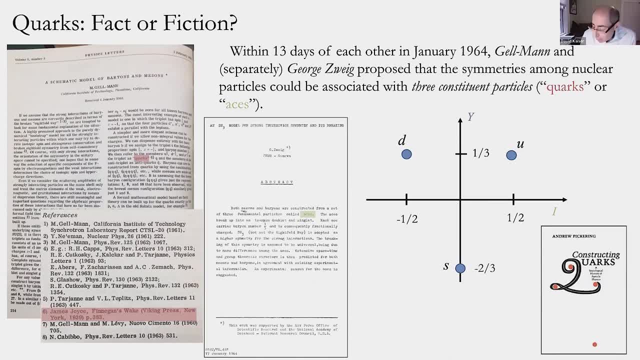 obtuse novel finnegan's wake, where this line many of you by now might recognize: three quarks for muster mark. if that doesn't make any sense to you, good it's, it's all nonsensical. uh, they're not. the irish novelist james joyce loved to make, basically making up his own. 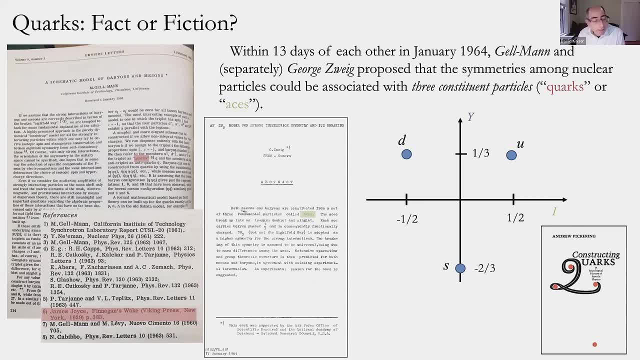 words and not bothering to, for example, you know, define them. and quarks was one of these kind of made-up names. he kind of liked the sound of it. well, gelman liked the sound of that, so he borrowed it. uh to to label this new hypothetical constituent: uh twig stuck with. 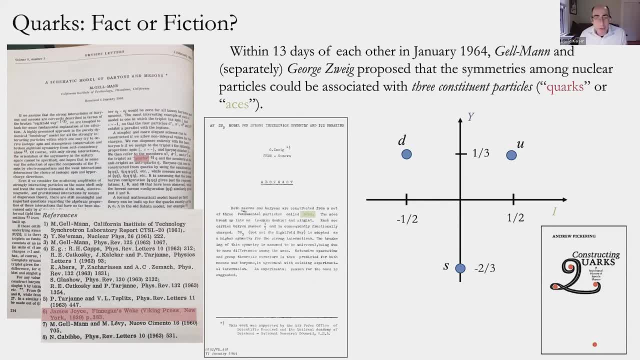 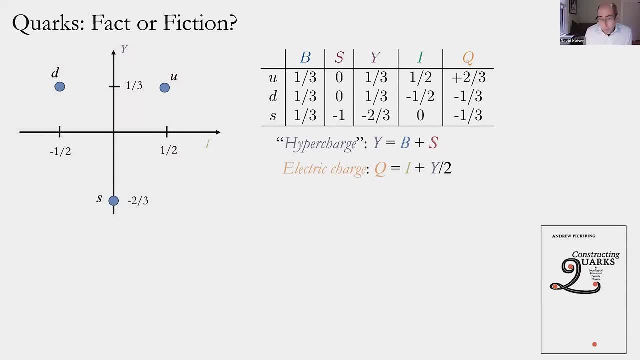 aces, which may be a little more familiar but still kind of a nonsensical word. so they could go through this exercise and assign baryon charge, strangeness charge, and therefore those two together would give you hypercharge. likewise, just kind of intuit or posit that the uh, two of those quarks would be, um, an isospin doublet, and the other two would be. 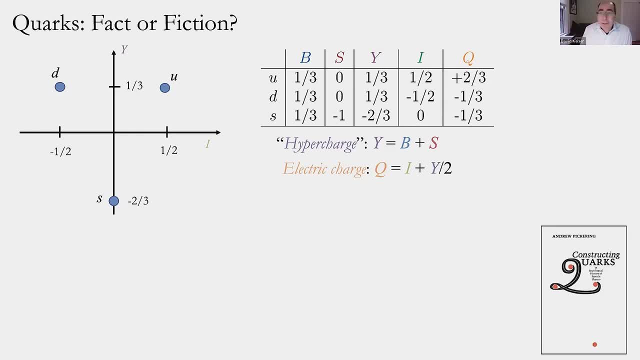 spin up, one would be isospin down. the third one would be what's called an isospin singlet, which means it had zero isospin, and if you do that, then again you can reproduce the electric charge assignments. so these became known as the up quark, the down quark and the strange quark and the idea. 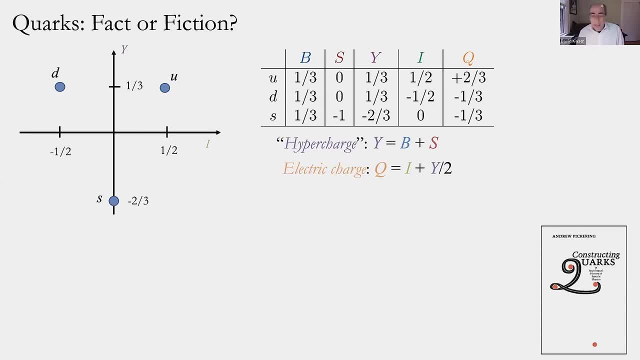 was that any of those so-called strange nuclear particles, the kaons, the um hyperons, the sigmas and all that, must include at least one constituent strange quark. that's what gave it strangeness charge, so it has strangeness charge, and then the other one would be spin up, one would be isospin. 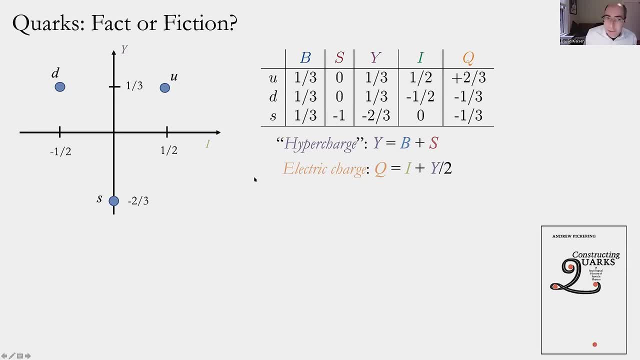 charge minus one, whereas particles that were made only from up and down quarks would have zero strangeness charge, like protons, neutrons and pions and so on. so with those assignments they could go through the known particles, even the more exotic or more recently found particles like the. 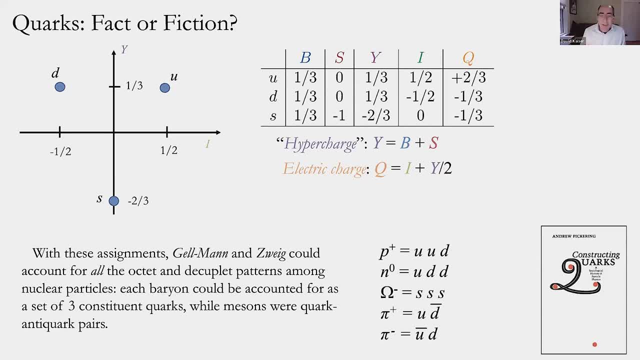 omega minus, and make these self-consistent assignments always on either triplets of these constituent quarks- if they were baryons like protons, neutrons or the omega minus, or a quark antiquark pair bound to the omega minus, or a quark anti-quark pair bound to the omega minus. 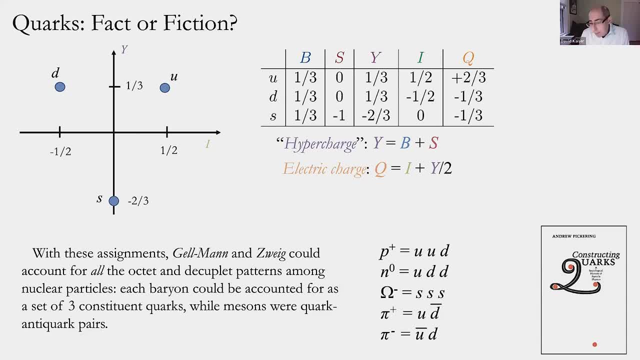 bound states of only two quarks if they were mesons like pions or kaons or others. so it was basically again even more a kind of um. it went from 2d sudoku to 3d sudoku, basically even more tightly constrained assignments for these three constituent, uh, hypothetical entities, and they 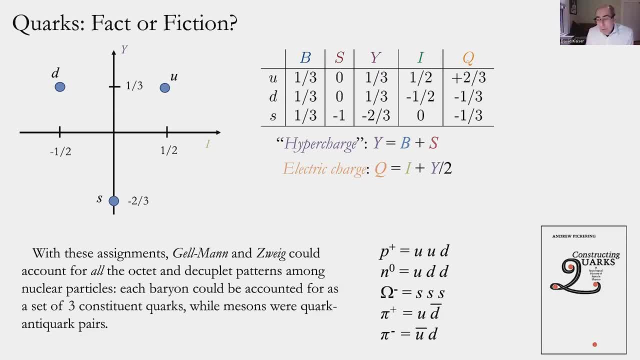 could reproduce all the kind of grouping structure in these abstract spaces like um, like hypercharge, isospin, and there's going to be a unique assignment for every one of those of those particles. uh, and so this looked like a remarkable kind of efficiency, right? instead of having a hundred, let. 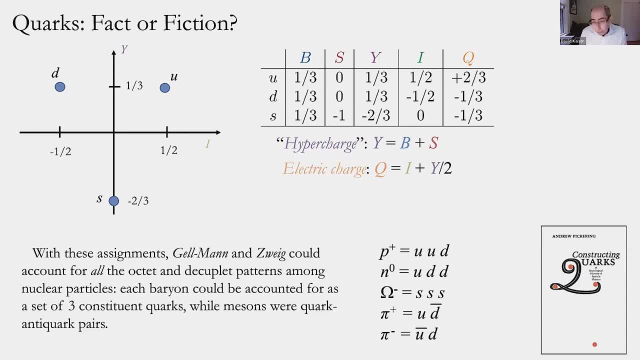 alone 300 seemingly elementary uh nuclear particles. you maybe only had to worry about three of them and then all these combinations. it looked more like the periodic tables from chemistry, where they're on the order of a hundred chemical elements, but based on developments from the early 20th century it looked like only a small number of elementary constituents whose combinations would 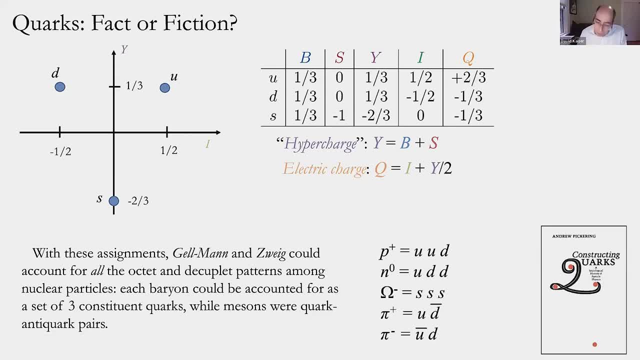 yield a hundred chemical particles. so this was actually a really interesting thing to look at the or more distinct chemical elements. It was that kind of move in the classify and simplify. So with these two papers written early in 1964, the idea was to put forward these very specific 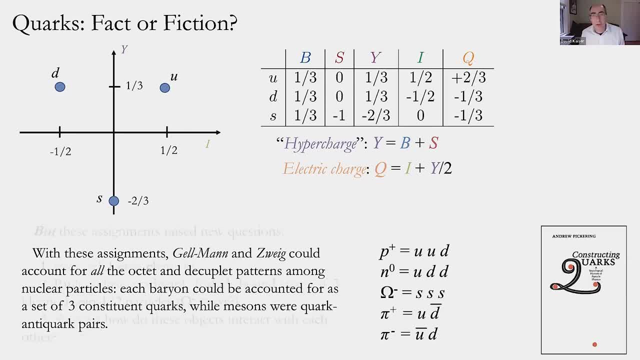 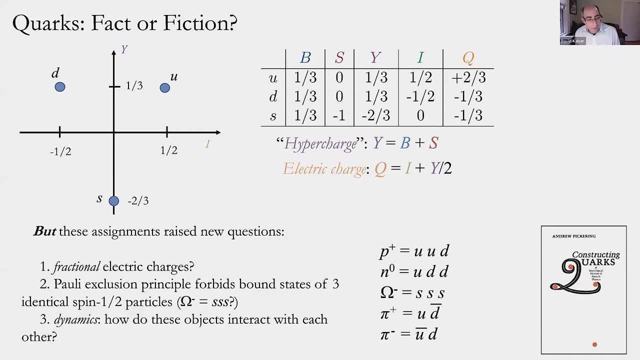 assignments for three constituent pieces within those nuclear particles. Now this raised new questions and it was not unfamiliar even to Gelman and Zweig themselves. The first one, and maybe the most obvious, is over here in this orange column, which maybe gave some of you pause. 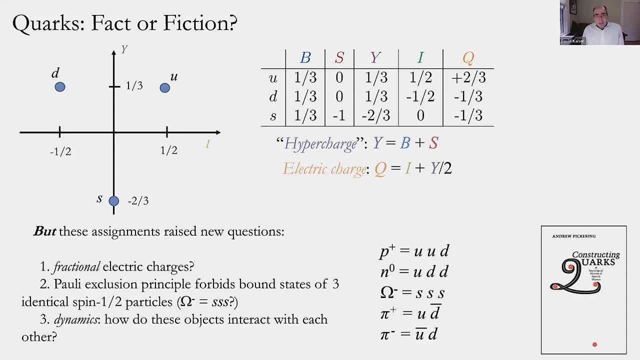 already, If not, I'll draw your attention to it. The suggestion seemed to be that these new particles of nature, the up, down and strange quarks, would carry fractional electric charge. The up quark would have plus two-thirds unit of charge in the unit of, say, the electron, Both the down and the 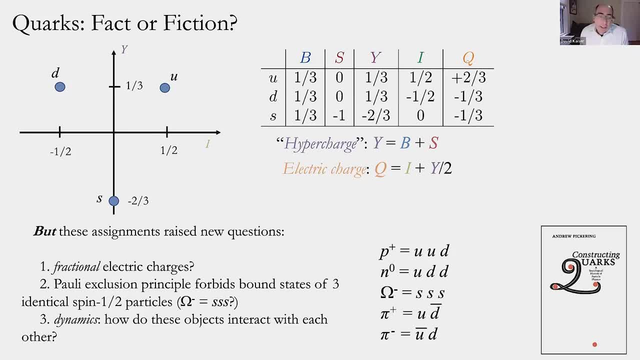 strange quarks would have minus one-third units of electric charge, and that, rightly, should give people a lot of energy. So you know, I don't know if this is a good idea, but I think it's a good idea. So you know, I don't know if this is a good idea, but I think it's a good idea. So you know. 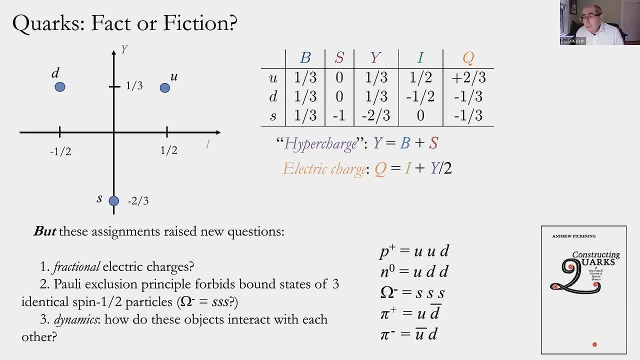 I certainly gave the authors of these ideas pause. There had been no compelling experimental evidence for half a century at that point for fractional electric charges. There had been early kind of ambiguous evidence in the early years of the 1900s and 1910s. It triggered actually some 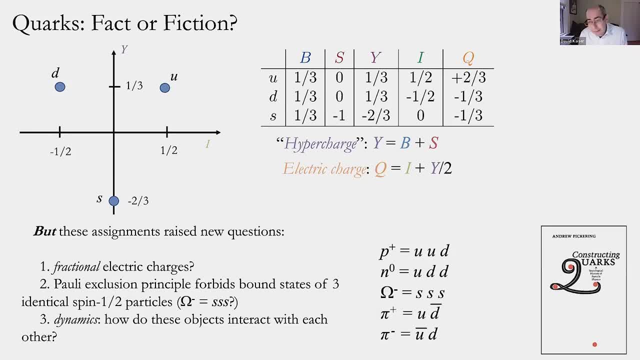 famously bitter fights among physicists back in the early 1910s whether labs had found evidence for fractional electric charges or not. By the 1900s there had been no compelling experimental evidence for fractional electric charges. There had been early kind of ambiguous evidence for fractional 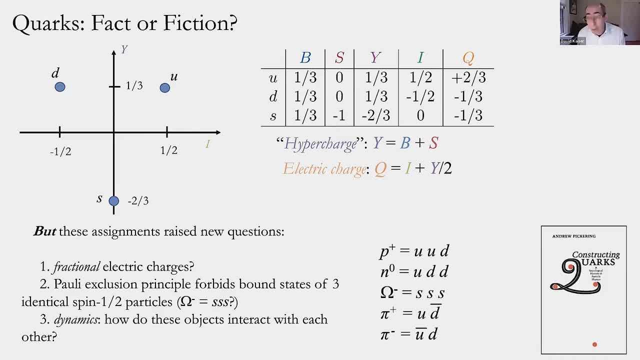 electric charges. There had been early kind of ambiguous evidence for fractional electric charges By the 1960s. that seemed to be very well settled and the answer was no. There was no compelling evidence. despite half a century of earnest experimental searching, no evidence for fractional 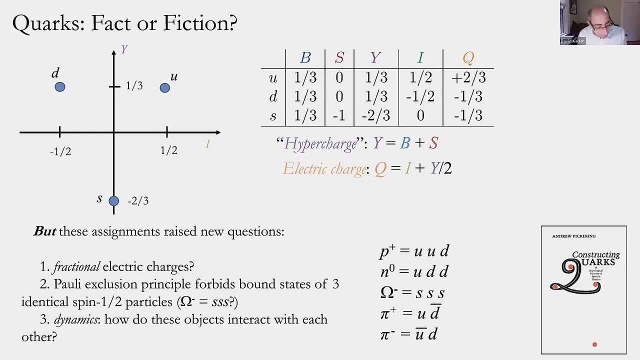 charges. And now they were saying that all of nature, all these nuclear particles, every constituent inside even very humdrum atoms like hydrogen and helium, is somehow teeming with particles of fractional electric charge. That seems hard to square with the evidence. So they 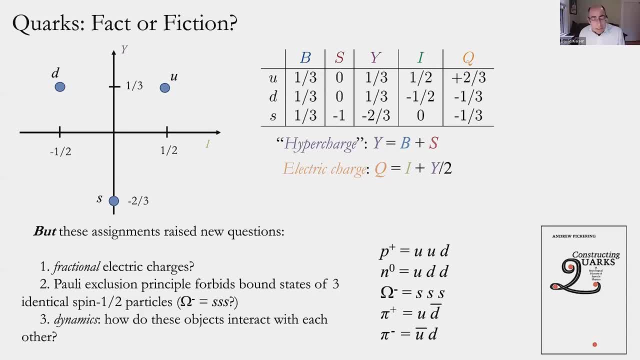 knew that. They wrote about that, as I'll mention more in a moment. There's a little more subtlety If you look at this great triumph of Gelman's earlier symmetry-driven approach, the omega minus particle. that was consistent on this new scheme with being a bound. 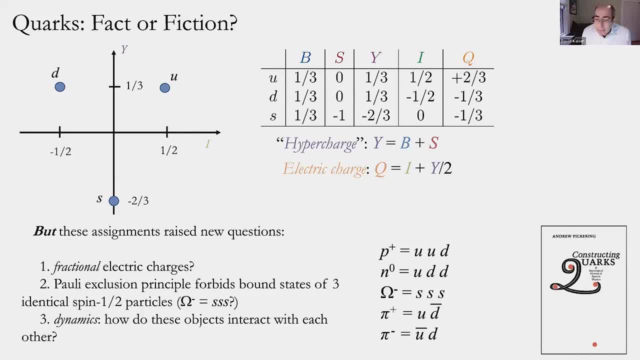 state of three strange quarks: S, S and S. But that now raises a little more subtle question for quantum theory, based on the Pauli exclusion principle, which we looked at together in this class a few weeks ago. The idea is that if you have spin one-half particles and these quarks 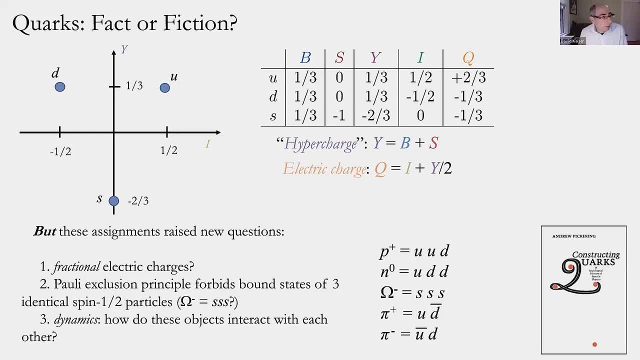 were assumed to be spin one-half particles, then you have spin one-half particles and you have spin one-half in the angular momentum kind of spin. then Pauli's exclusion principle forbids having any two spin one-half particles in the identical quantum state at the same time. So if 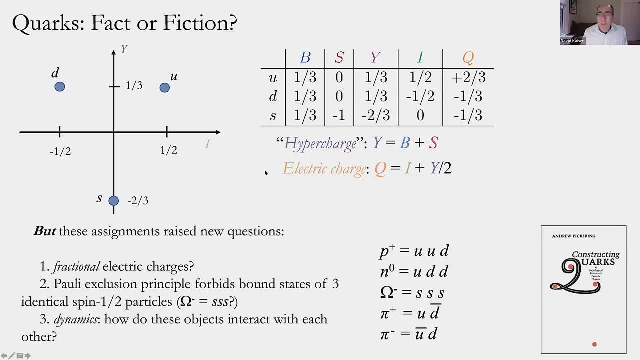 you're assigning all these internal quantum numbers to these particles, how could you possibly have three strange quarks bound together? That means at least two of them must have all these assignments plus also either be two of them spin up or two of them spin down The other, the last charge you have. 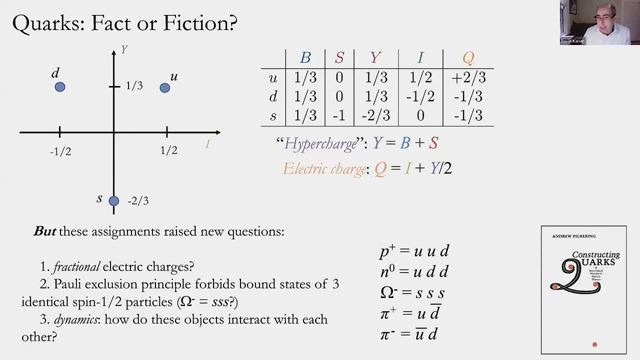 to assign to the actual angular momentum spin. that could also either be only plus one-half or minus one-half. If you have three of them bound together, two of them are going to overlap with spin. that seems to violate the exclusion principle. That's a bit more abstract than no evidence for fractional 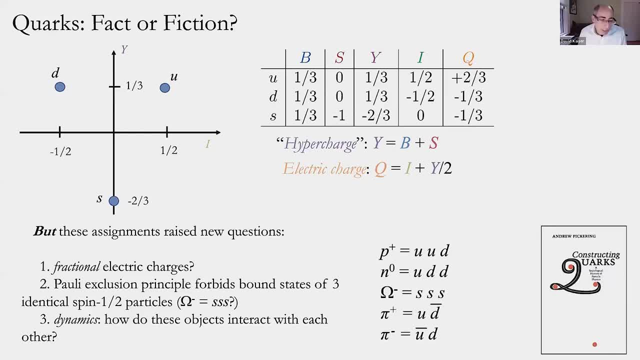 charge, but the exclusion principle had been awfully well tested by the 1960s. That seemed like a pretty significant conceptual challenge. And then, third, as I mentioned earlier, in neither Norzweig's scheme was there any discussion of forces of dynamics. Why do these objects interact? 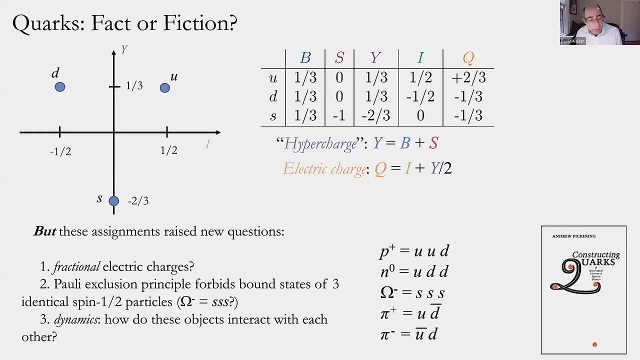 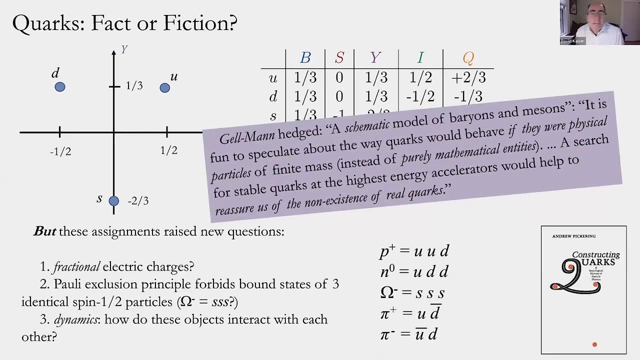 with each other. Why do some have very large reaction rates, others have very small reaction rates, and so on? So there's still no idea of the kind of forces that might interact either between these constituent quarks or as a result of them. And so, as a result of that, Gilman, who was no dummy- 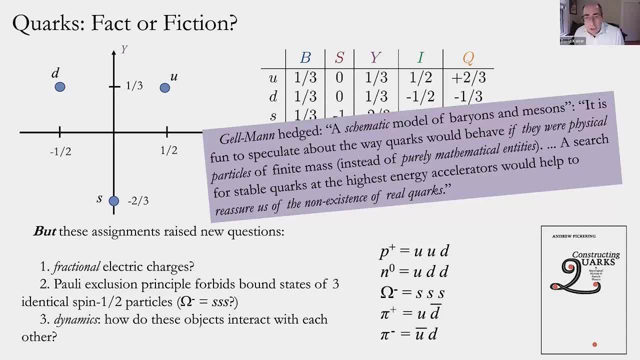 he hedged- you might have noticed on the very title of his article that I showed in the previous set of slides- was called a schematic model of baryons and mesons. You may remember it back to very early this term We talked about when Einstein introduced the idea of light quanta. he called it a heuristic. 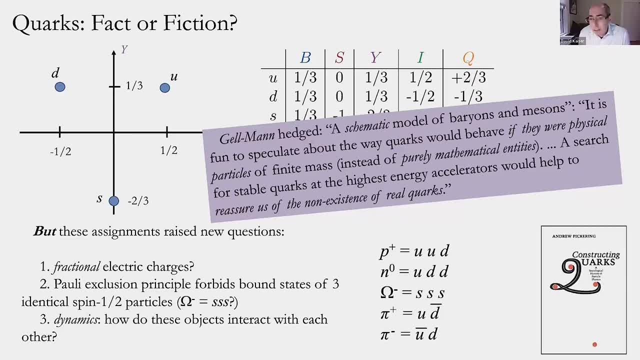 suggestion and that's very much like what Gilman is doing here. It's a schematic model he announces even in the title. He goes on to say: near the very end of the last main paragraph of this brief article, Gilman writes: it's fun to speculate about the way quarks would behave if they were. 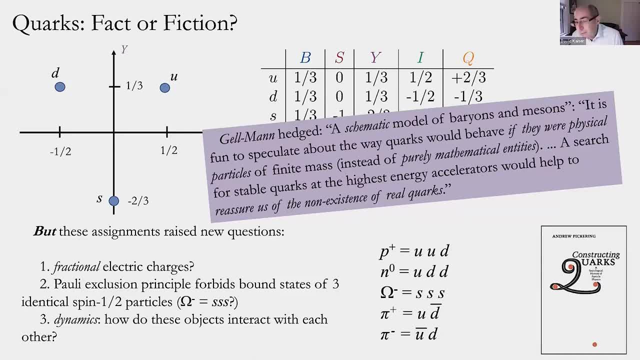 fixed. but it's also fun to speculate about the way quarks would behave if they were fixed. So he goes on to say: if you're looking at physical particles instead of purely mathematical entities- that's my italics- a search for stable quarks at the highest energy accelerators would 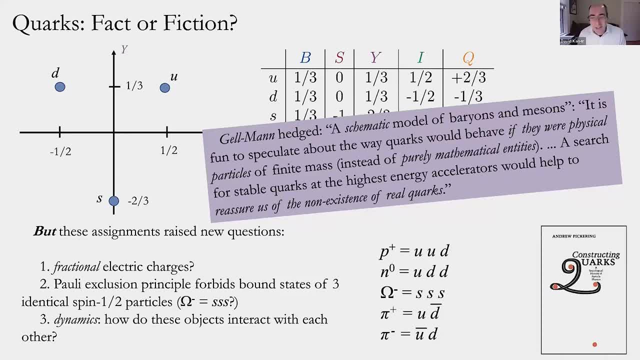 help to reassure us that they don't exist at all, reassure us of the non-existence of real quarks, precisely because of things like no one's ever found fractional electric charges, these subtleties about the exclusion principle, and so on. So Gilman, in his very first article from 1964,: 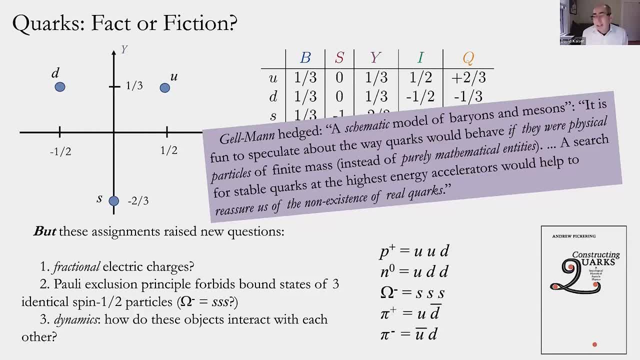 was not saying Eureka, I found them. He was saying it's helpful to think about, as if protons, neutrons and omega minuses and everything else were made up of these constituent parts. but it's really just a kind of mathematical shell game. 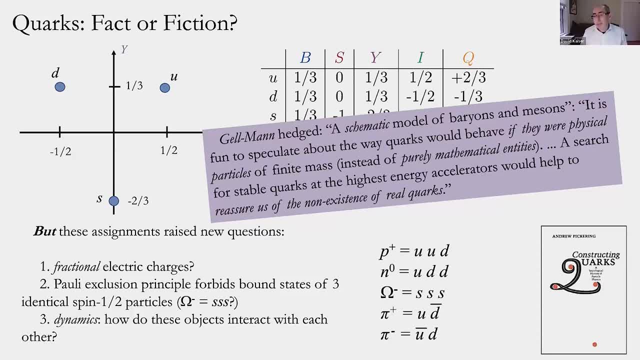 These are mathematical classifiers rather than parts of nature. That's, I think, a fair reading of what Gilman is saying in this 1964 article. Meanwhile, George Zweig, a couple years younger than Gilman, didn't even get the benefit of the doubt, So Gilman's paper was rushed into print. after three weeks. Gilman, in his very first article from 1964, was not saying Eureka. it's helpful to think about as if protons, neutrons and omega minuses and everything else were made up of these constituent parts. 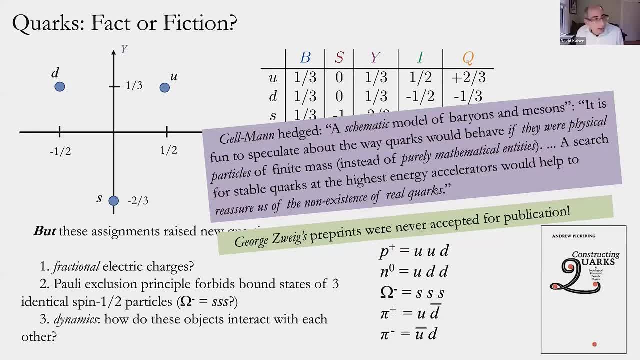 Gilman. he wrote two papers within a few days of each other, in January of 1964, both of which were rejected for publication. Neither of them even made it through peer review. He was a very young postdoc at that point And they said: this doesn't make any sense at all. no fractional charge. 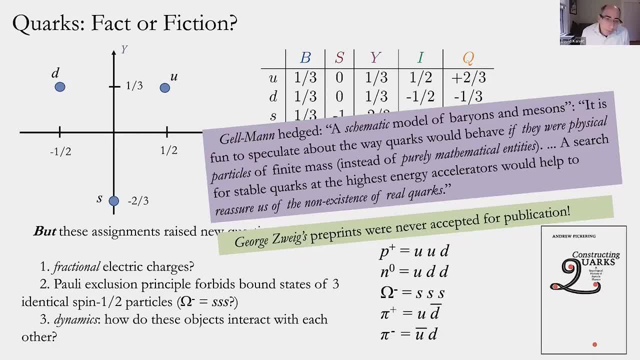 exclusion principle and so on. Plus, everyone seemed to have confidence. by this point. many people did that. actually Jeffrey Chu's approach, the kind of single, self-consistent bootstrap, was going to kind of save the day. That had made enormous progress. 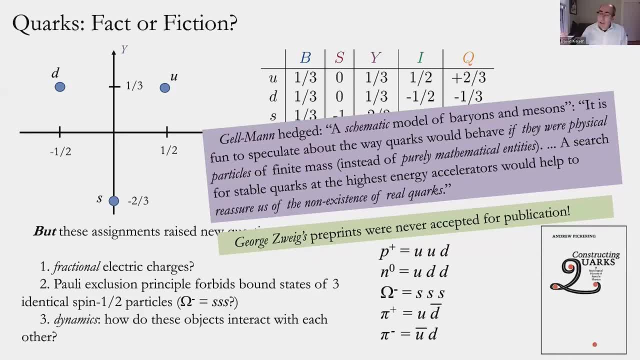 experimentally and it was going to save the day. So Gilman, in his very first article from 1964, experimentally by the late 50s, and this seemed to go exactly counter to that single, self-consistent bootstrap idea. This was reintroducing, or seemed to be reintroducing, the idea of a small set of 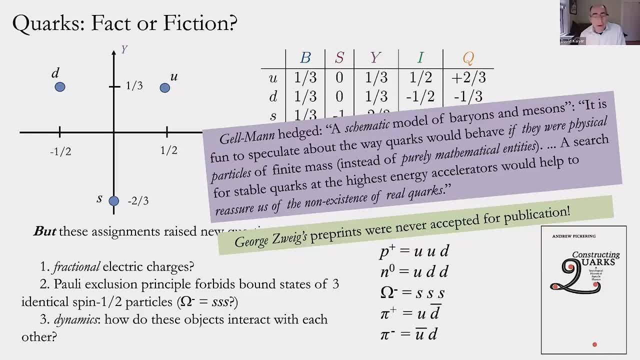 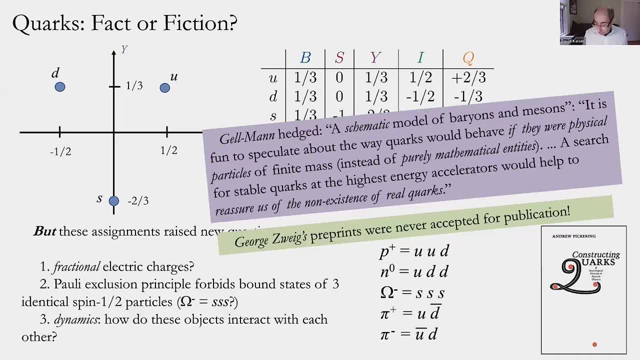 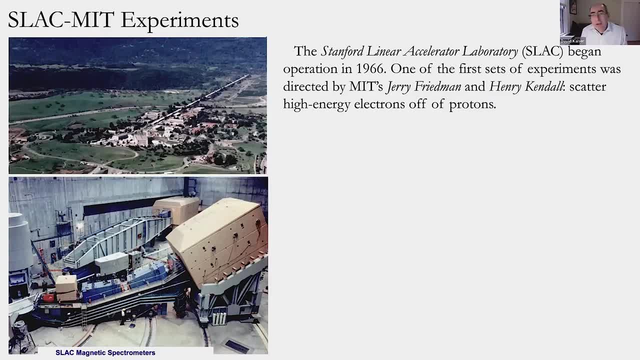 some very dramatic new experiments were conducted. These are often, depending on who you ask. they're either called the Slack MIT experiments or the MIT Slack experiments. I'll let you guess which coast prefers which version. These were some of the first experiments conducted. at what? 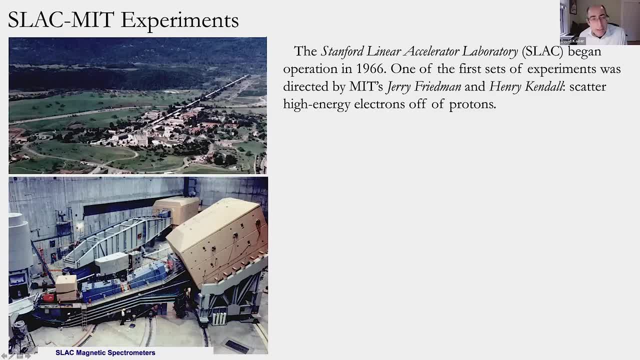 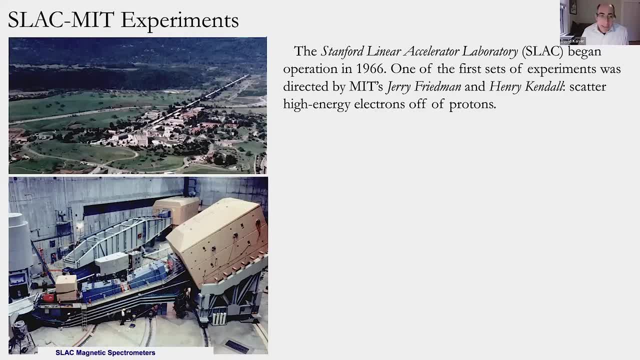 the Stanford Linear Accelerator Laboratory. It is a linear straight line, It's 3.2 kilometers, basically two miles long, And it's a series of electrostatic voltage gaps, So along which you can accelerate electrons to very, very high energies, basically up to a significant fraction. 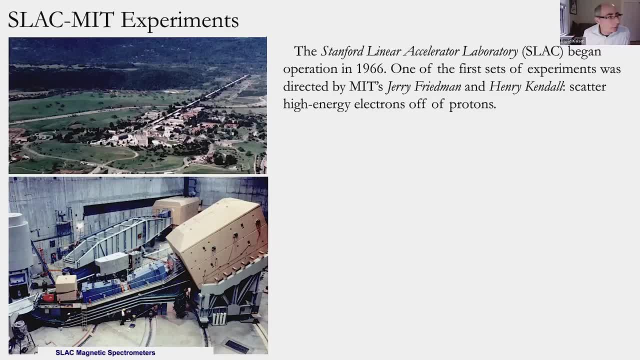 of the speed of light. You just keep shoving electrons with very clever electric fields down a two-mile track and smash them into stationary targets. And so one of the first applications of this new device built for the same reasons we've talked about before as part. 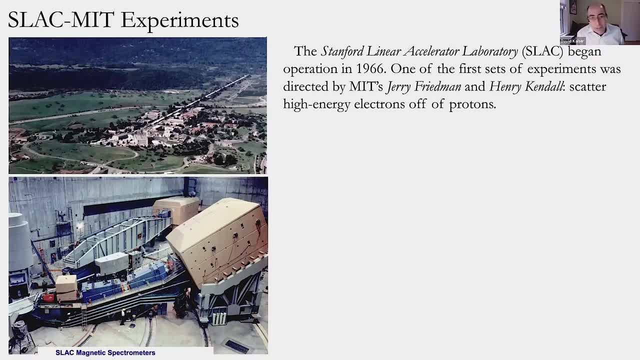 of the Atomic Energy Commission effort to get lots and lots of physicists kind of trained and at the ready. Not that this would help make weapons for defense, but it would make people well-trained who could be mobilized in a new Manhattan Project if needed. This is a huge version of that post-war. 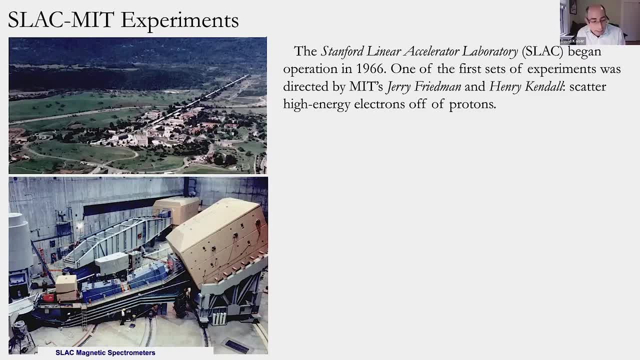 policy. It's making very, very expensive machinery available for non-military purposes to keep communities well-trained, even though this device itself is strictly for kind of peacetime questions. So SLAC came online in 1966. And one of the very first sets of experiments to go in 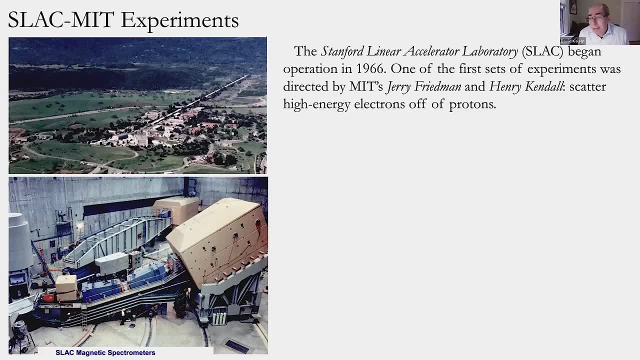 there was actually directed and designed by two members of the MIT Physics Department, one of whom is still with us. He's emeritus professor Jerry Friedman. You might have met Professor Friedman. He comes to colloquia and so on, And then Henry Kendall, who passed away some years. 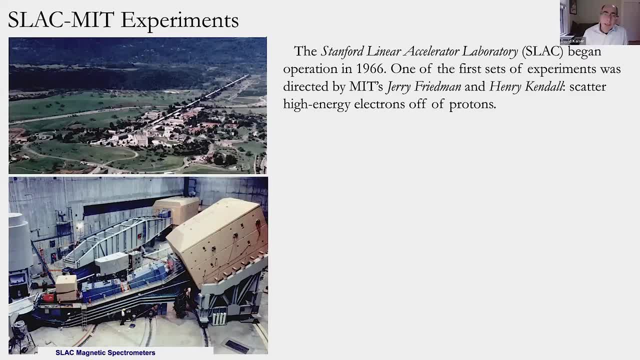 ago. The two of them were partners in these experiments. The idea was to accelerate these electrons to very high energies and smash them into very proton-rich targets. So you could actually study very high-energy electron-proton scattering In the detector bay at the end of that. 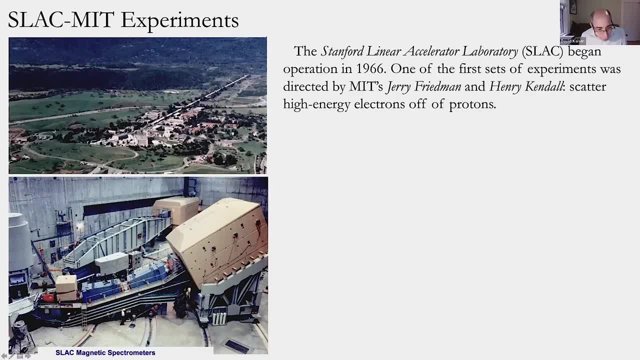 line you have this unbelievable equipment. You can see this is like train tracking, And here's a person for a sense of scale, where you could actually change the angle At which you measure the detritus that comes out of these very high-energy scatterings. 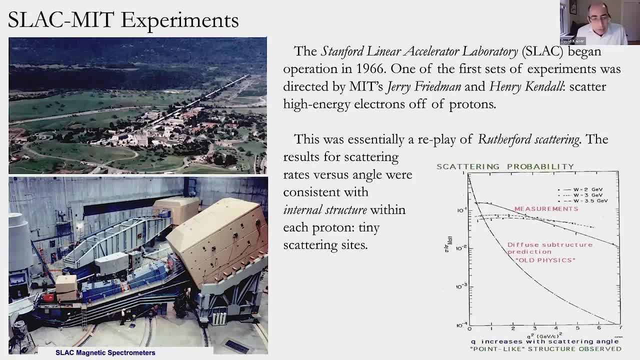 This is basically a redo of Rutherford scattering, but now across miles as opposed to across a single desktop. You may remember back from in the early several weeks ago. in our class we were looking at Rutherford scattering from around 1909, 1911, firing alpha particles at very thin gold foil. 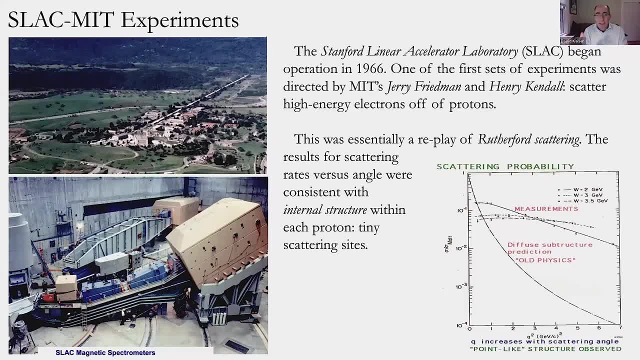 and then surrounding it with scintillating screen So you could get information for the number of scatterings per angle as a function of scattering angle. And Rutherford was so shocked when he found a significant number of backscatter events where the incoming projectile scattered almost all the way backwards, which was consistent only with a. 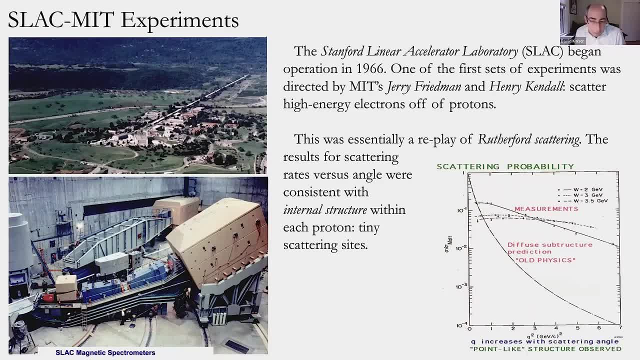 very small, very massive inner core to the atom that became known as the atomic nucleus. Now they're doing the same thing, but not with a thin metal foil, but literally moving these enormous, enormous detectors around in a semicircle on these kind of inbuilt train tracks so they could get things like scattering rates as a 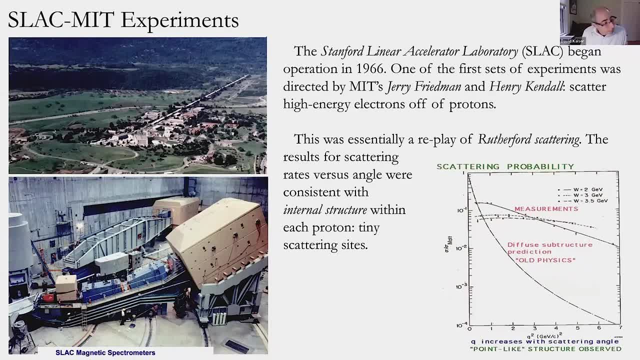 function of angle. I just find that astonishing that in that case, well, roughly 50 years or 60 years, maybe they'd gone from the same basic concept, but now taking miles and train tracks as opposed to a grad student sitting in the dark. Anyway, what they found, the 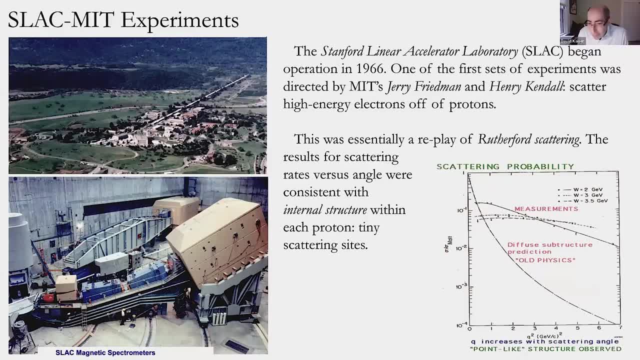 SLAC-MIT experiments was again very similar pattern to what Rutherford and his team had found about atoms When they were scattering off of protons. they found evidence for an internal structure within protons. Protons seem to have internal hard scattering sites, just like atoms. 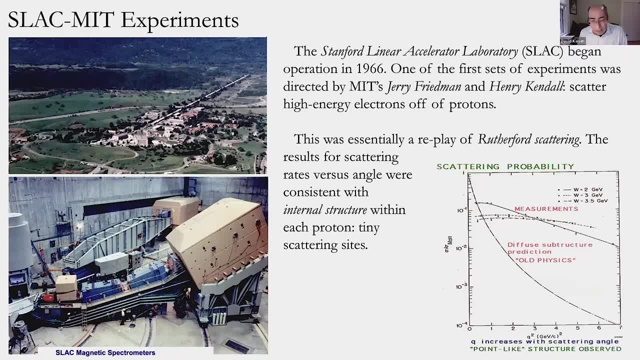 in that gold foil seem to have internal hard scattering sites that we now call the nucleus. The particle physicists by this point were using a bit funny method, which is to say, well, if you have a proton, you're going to be able to do a lot of. 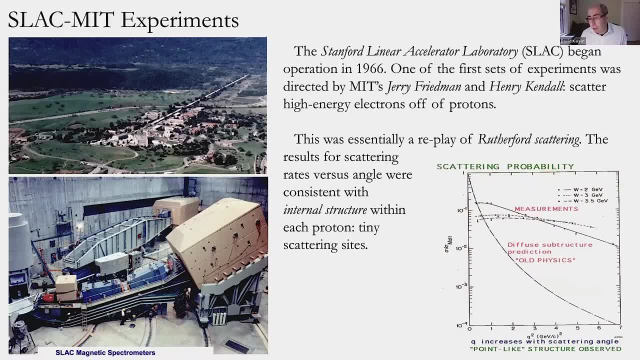 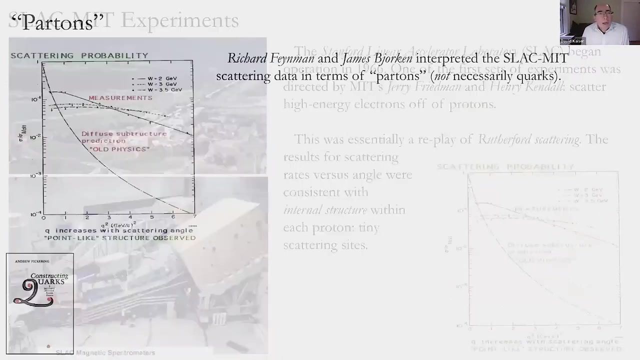 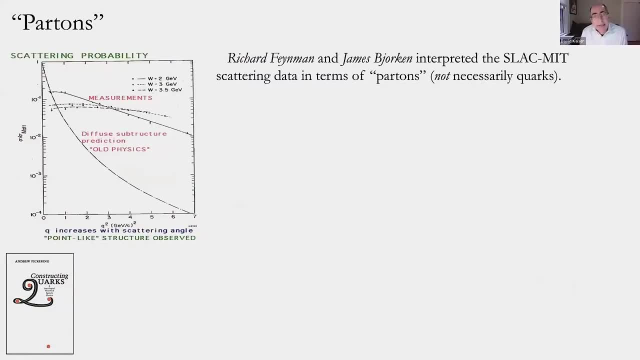 the fact that there seems to be a structure inside these proton targets. but could you actually reproduce those curves with a real, specific structure inside the proton? So a number of theorists who were following the SLAC MIT experiments closely- they jumped in, one of whom. 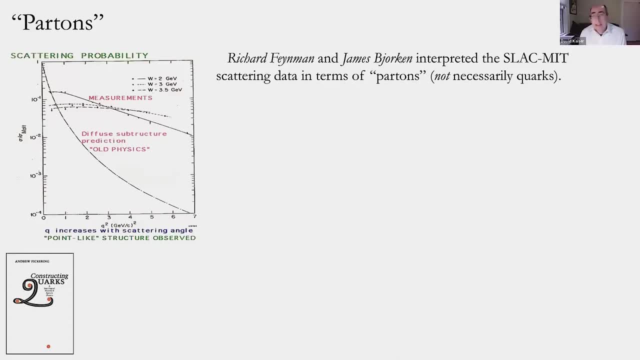 was Richard Feynman, some of whose work we already looked at together in this class. The other was, at the time, a much younger theoretical physicist named James Bjorken. He often just goes by BJ for the start of his last name. 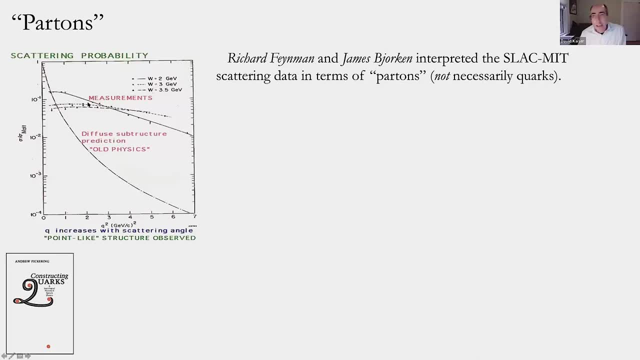 They were able to make sense of the scattering data quantitatively, not just qualitatively. there's a scattering site, But they could actually reproduce these very specific curves, those scaling laws, by introducing what they called partons. This was Feynman's kind of joke. 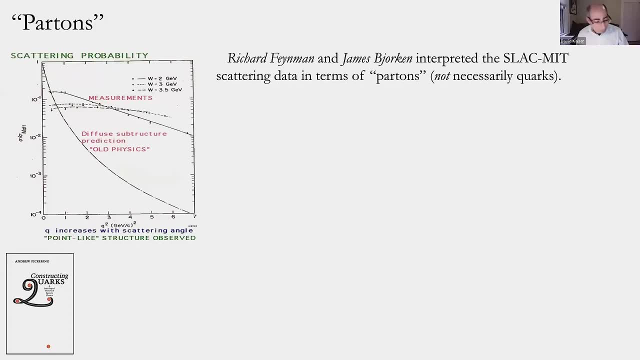 So he was absolutely clear not to call these quarks Part Because, as we'll see, they were conceptually quite different, partly because by this point both Feynman and Gelman were together at Caltech, in the same Department of Physics. 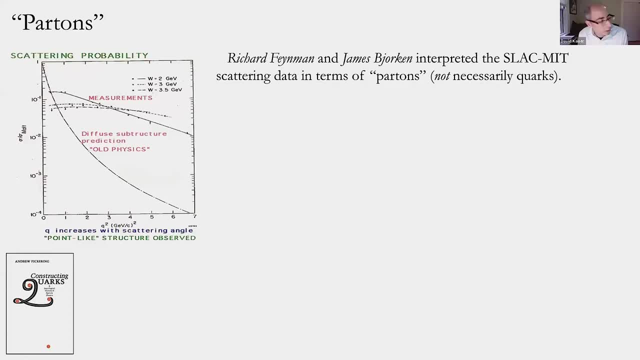 and they were kind of friendly rivals. Feynman had a lot of these relationships throughout his life, So by this point he traded Julian Schwinger as his main rival for Marie Gelman. Their offices were just down the hall, And so Feynman was as much tweaking his nose at Gelman. 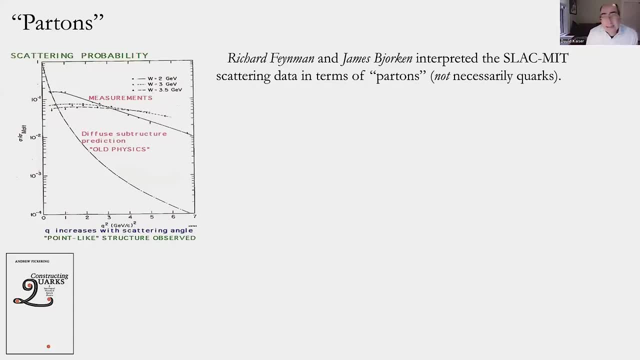 as being kind of- maybe appropriately- skeptical by very intentionally not calling his new theoretical particles quarks. They were called partons, meaning there are some parts inside of protons. I thought it was a cute name. These are parts inside protons. So the idea was: why would this help? 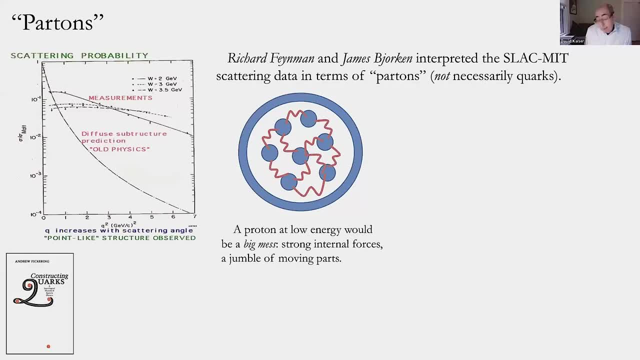 How would you make theoretical sense of these experiments? And this again, I think was kind of classic Feynman in his use of intuition At low energies. inside a nucleus, a proton would actually be a big mess if it has internal structure, whether they're. 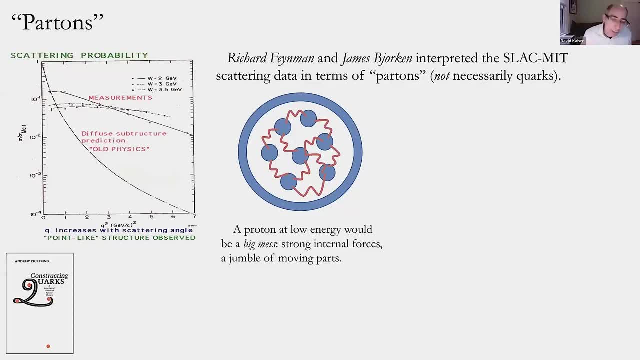 quarks or anything else. If there are parts within a proton, then they're going to be subject to very strong internal forces. After all, protons don't fall apart, So whatever internal parts it might have must be stuck together very, very tightly. 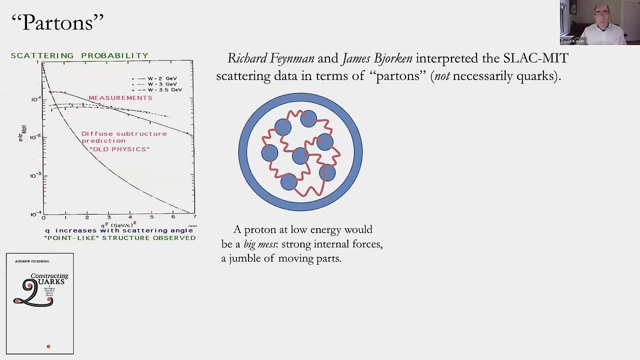 at very strong nuclear forces. So it would be some jumble of moving parts with a big dynamical mess And people had no idea how to calculate that. Remember perturbation theory failed and all that. So at low energies a proton would basically. 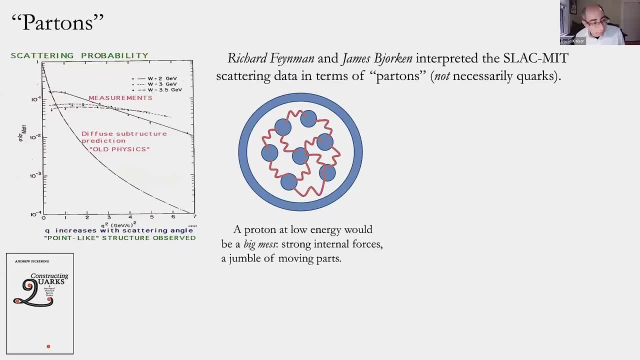 be extremely difficult to characterize quantitatively Right. Luckily for Feynman and Bjorken and their colleagues, that was not the situation at hand. To make sense of the slack MIT experiments, they were going to, in a sense, the opposite regime. 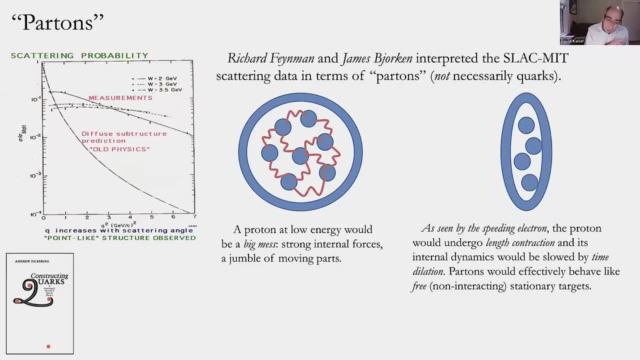 The protons were stationary targets, But what mattered was the view from the speeding electron, And the electron had just as much license as the person riding on Einstein's imaginary trains to pretend that the electron was fully at rest, and it saw the target racing toward it at very high speeds. 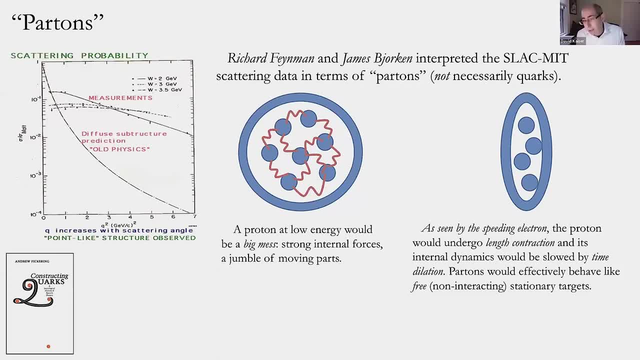 So if you imagine sitting on the electron, you could say you're sitting at rest while the proton target races toward you at a very high fraction of the speed of light. So from your point of view as the electron, you see the proton undergo length contraction. 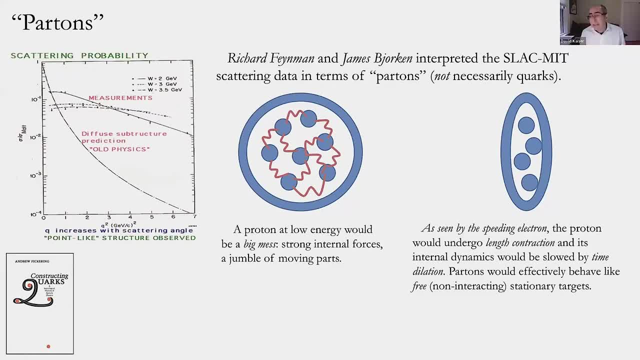 become a pancake along its direction of motion and its internal clocks will be slowed. It will undergo time dilation, at least as far as you're concerned. So all of the time scales for these very big, complicated nuclear forces would be slowed down. 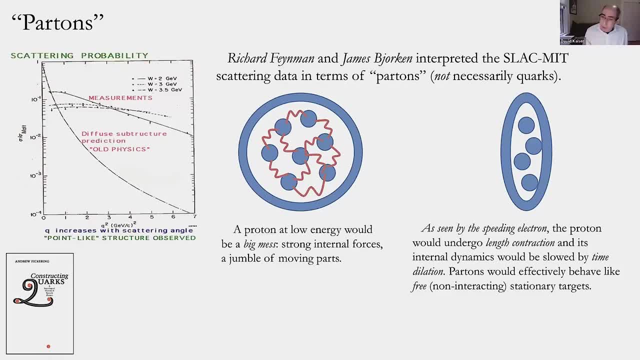 They would be slowed down as if they were frozen in time. What the electron would see in this target of the proton would basically be a frozen set of free, non-interacting stationary targets. All the stuff that people had no possibility to calculate, these strong, fast-changing nuclear forces. 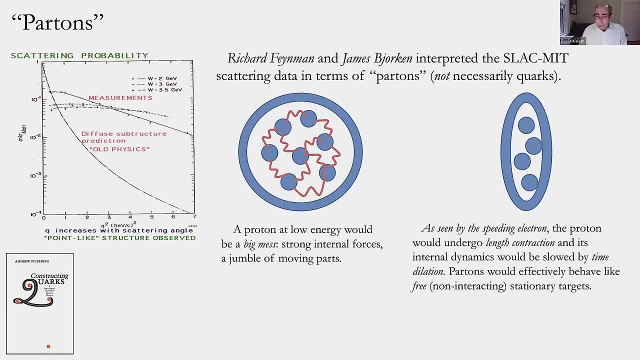 become irrelevant in the limits of very high energies as relevant for these slack MIT experiments. So you can go for these internal parts called protons and analyze all this very specific scattering data based on kind of free protons, because in the energy regimes 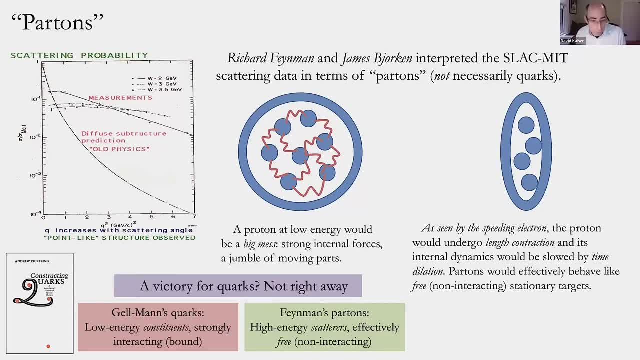 of interest. the dynamical forces should basically be irrelevant or subdominant. So you might say, was this a victory for quarks? Well, not right away. As I've mentioned, Feynman went out of his way not to call these protons quarks. 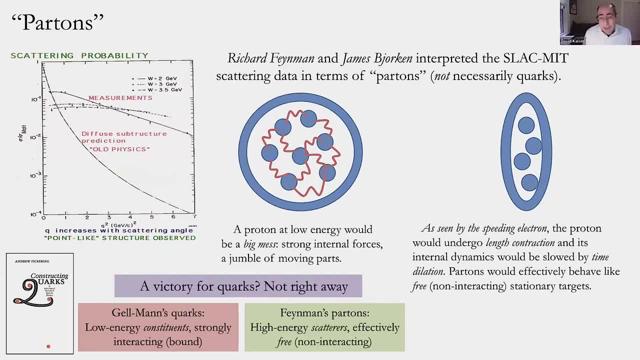 The two sets of ideas really were answering different kinds of questions. So Gell-Mans or, even more importantly, George Zweig's notion of quarks from early 1964, that was really a kind of constituent model. What are the little pieces that are bound tightly? 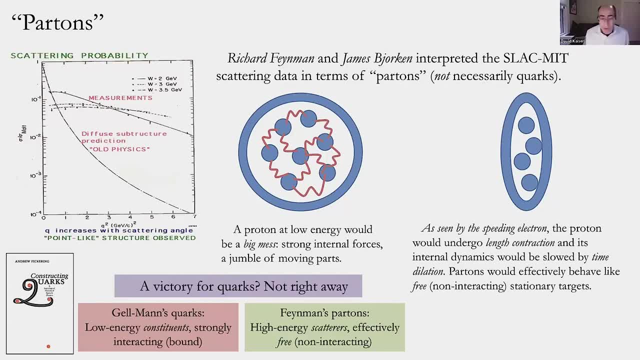 inside protons, neutrons, hyperons and all the rest. It's about the kind of internal parts and, eventually, the forces that must keep them bound together so that we don't see things like free fractional charge, And Feynman's partons were really. 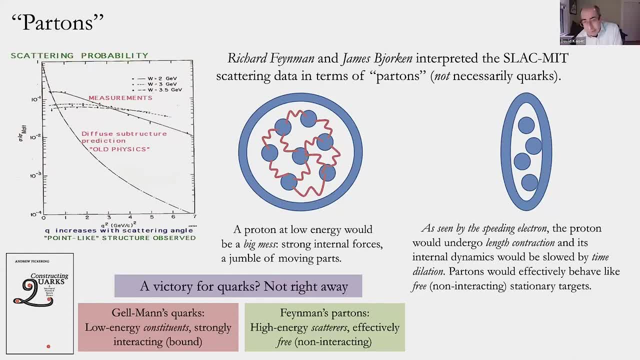 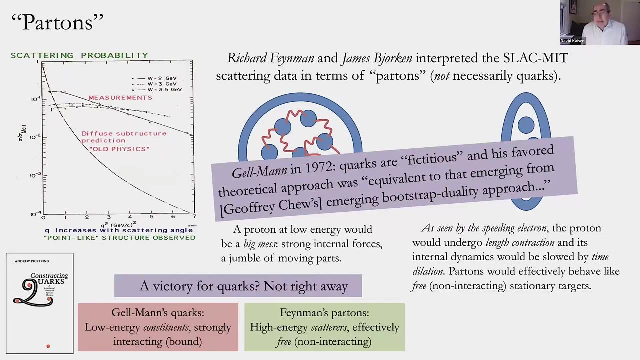 answering just an entirely separate set of questions, very high-energy behavior. when you basically ignore the internal forces, You have effectively free scatterers as opposed to bound, strongly interacting particles. And again, you don't just take my word for it that this wasn't seen in his day as direct evidence for quarks. 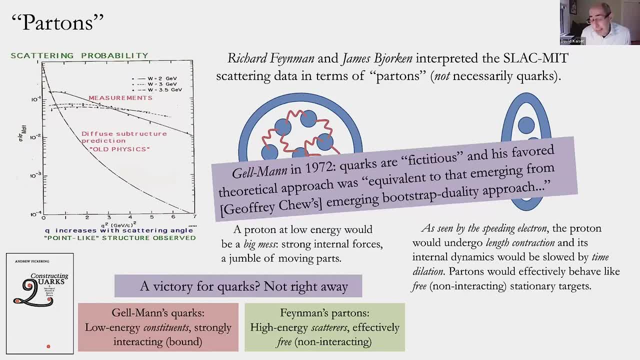 Gell-Man himself three years later. three and four years later mentioned at a very well-attended conference for high-energy physics that quarks were still fictitious- his word- and that his own favorite theoretical approach was actually equivalent. Gell-Man himself three years later. three and four years later. 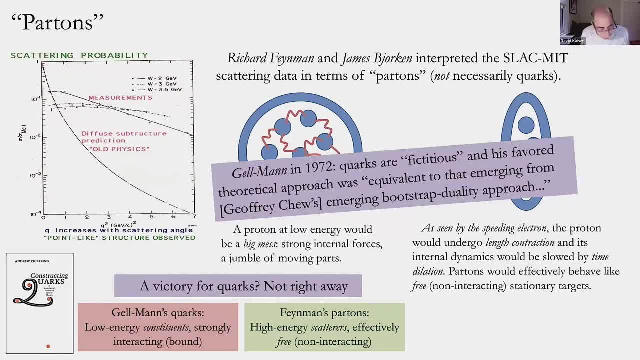 mentioned at a very well-attended conference for high-energy physics that quarks were still fictitious- his word- and that his own favorite theoretical approach was actually equivalent to the kind of ongoing work from that Berkeley tradition called On the Bootstrap, which disavows a set of literally elementary particles. 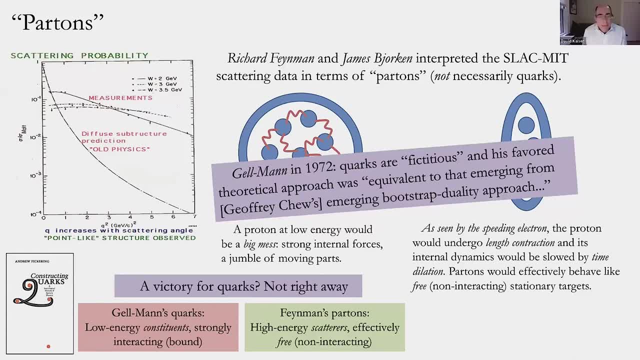 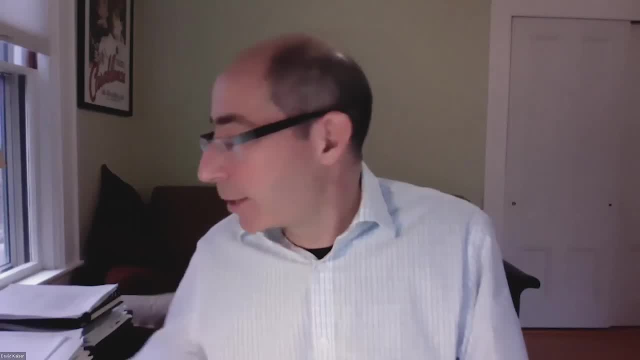 and talks about the kind of self-consistent composites one can make from the nuclear particles. So Gell-Man himself didn't leap on the SLAC, MIT results to say: now we've found quarks, let alone Feynman. So this was again a kind of slow drift. So let me pause there and see if any questions on SLAC, MIT or any of that kind of stuff. 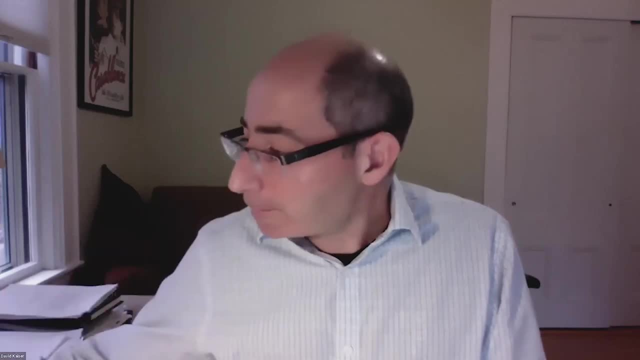 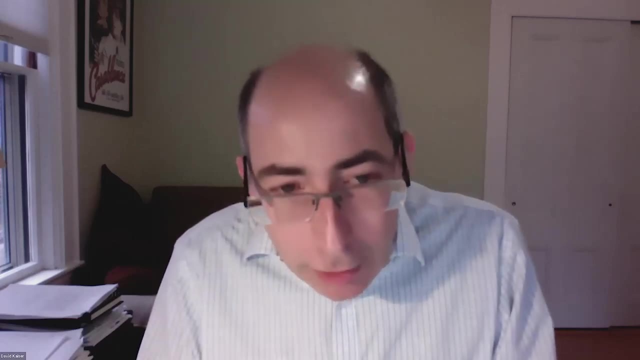 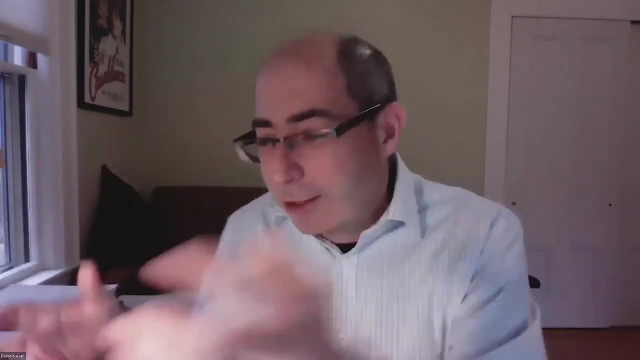 I know I've said it before but I just love that contrast from the Rutherford. scattering of the whole apparatus was maybe a meter across to two miles with that train track to change scattering angle of your detectors. I just think that's pretty, that right there. 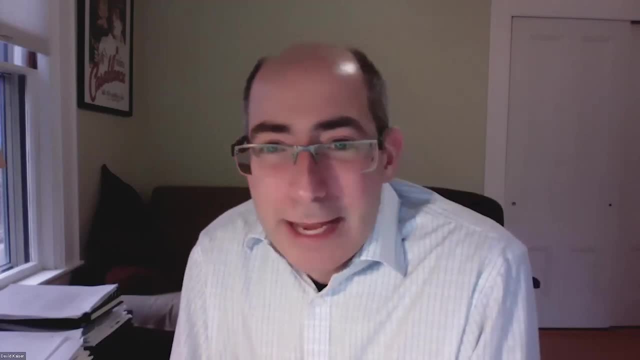 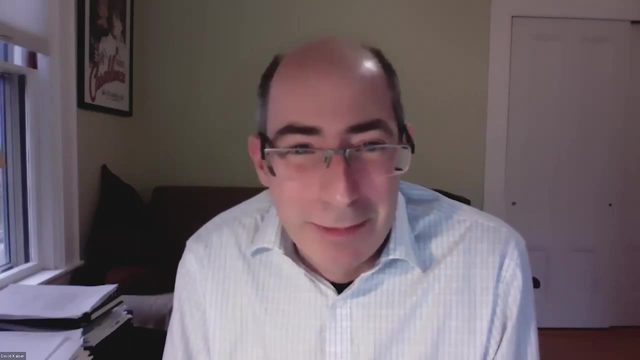 is the story of high-energy physics in the 20th century, that transition. You're asking basically the same question, getting remarkably consistent results, but you had to do a lot more. You had to do a lot of work in between and convince a lot more people to pay the money to let you do it. 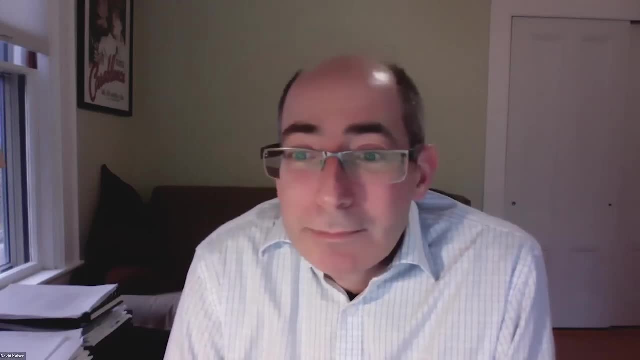 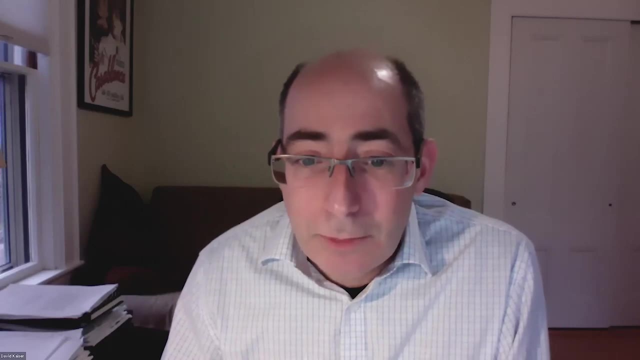 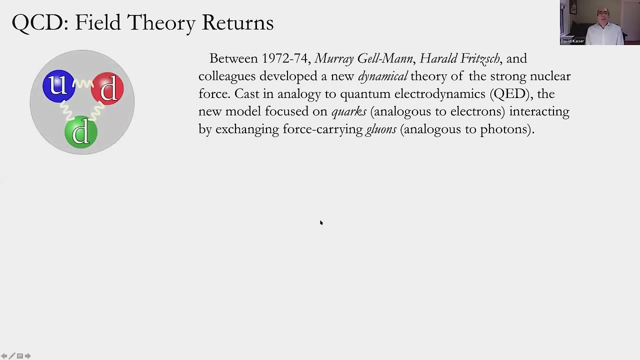 Any questions on that? Okay, I will press on. If any questions come up, of course, please chime in. Let's go to that last part for today and talk about quantum chromodynamics. So right around the time when Gell-Man stood up at the conference in Florida. 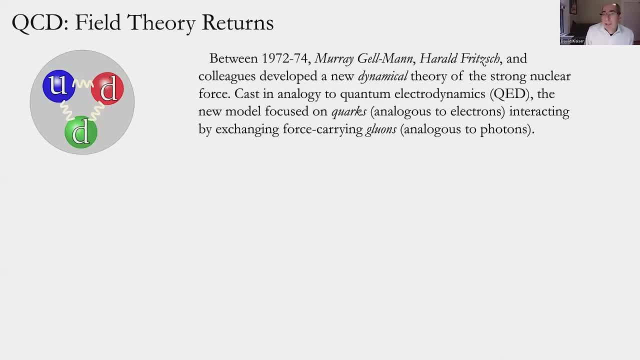 and said quarks, as we all know, are fictitious. he was actually working on a whole new theoretical approach, sometimes with co-authors and others working independently. Another key architect of this was a younger theorist named Harold Fritsch. 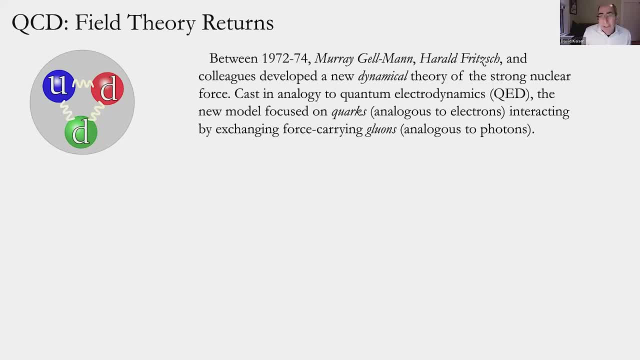 They were developing what came to be called quantum chromodynamics or QCD. The idea now was to in some sense to finally ask this question about dynamics, about forces which Gell-Man himself had very successfully kind of bracketed or left aside. 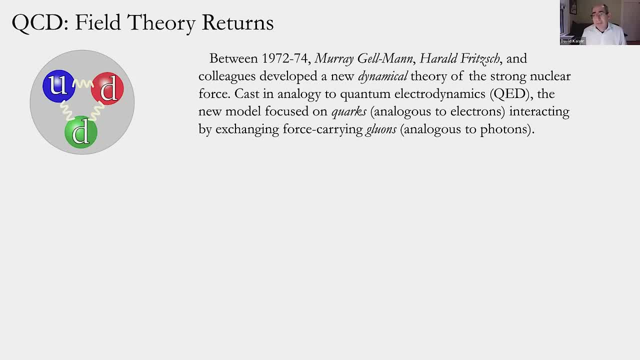 from the 1950s. The idea now was to try to look more squarely at forces and try to find a quantitative way of making sense of these nuclear constituents. So they're working in very explicit analogy to QED, to quantum electrodynamics. 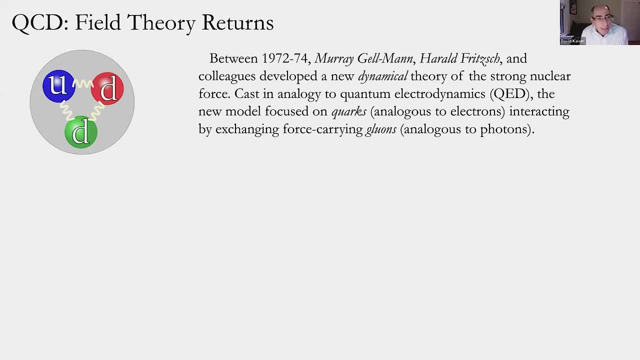 the work that we saw in previous class sessions that really had kind of come together soon after the Second World War, in the late 1940s, though the roots of it went back to the early days of quantum theory, So there really was a kind of step-by-step analogy. 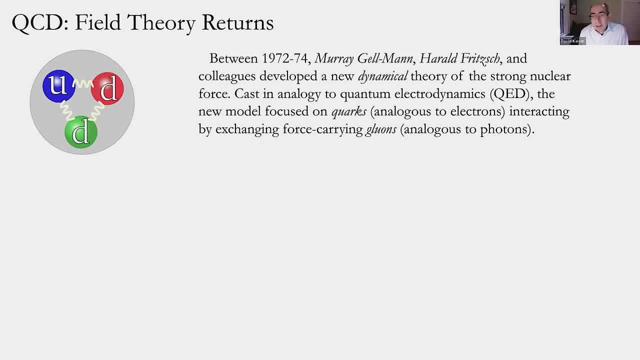 In the new work. in place of electrons and positrons, the new work would focus on quarks. Those were the kind of elementary particles that would be subjecting each other to forces. So just like electrons could repel electrons, quarks could repel or attract other quarks. 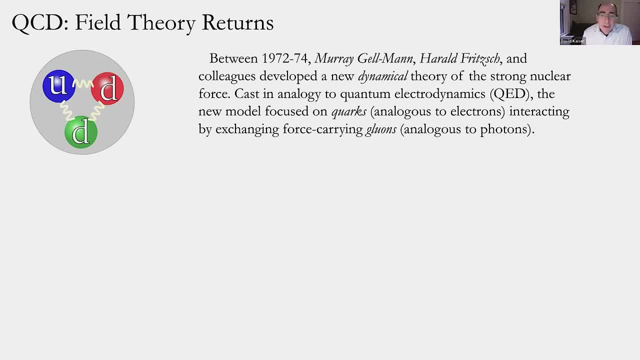 And the quarks would interact in the new scheme by exchanging a new kind of force-carrying particle called the gluon. This would be the glue, the nuclear glue that would keep, say, an up, down and down quark bound within a proton or within, in this case, a neutron. 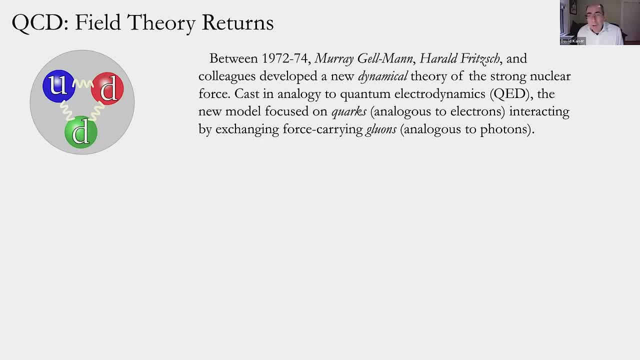 So the gluons, which were maybe not the most creative name, they were meant to be nuclear glue. they would play the analogous role to the photons. Remember we saw electrons on the idea from quantum field theory would repel each other by firing force-carrying photons at each other back and forth, the virtual photons. 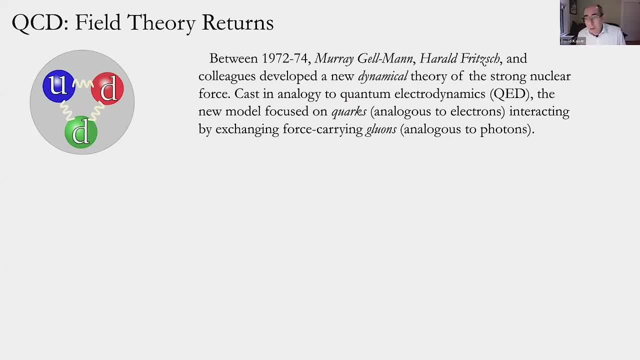 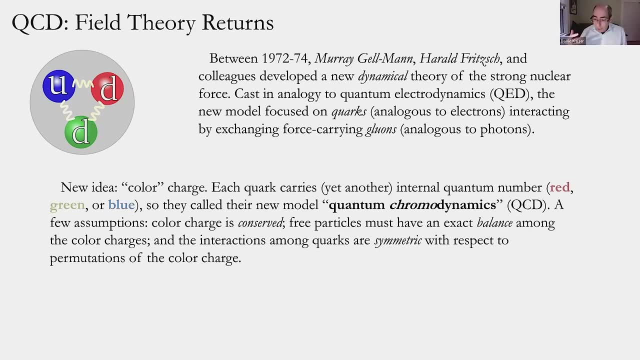 And now you have a similar structure, at least hypothetically, about quarks interacting by the exchange of gluons. OK, So there are some new ideas again to try to make sense of all the newer sort of classifications and symmetries and internal charges and stuff that had been introduced. 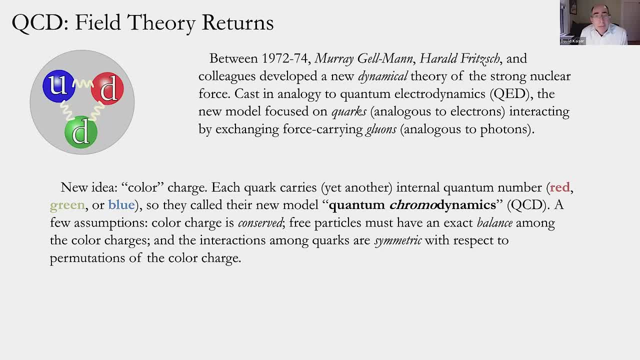 for the nuclear particles over the previous 20 years. The main idea, the main new ingredient conceptually for this newer QCD was to introduce yet another internal quantum number or charge- Again strictly hypothetical at this point, And they called it color. 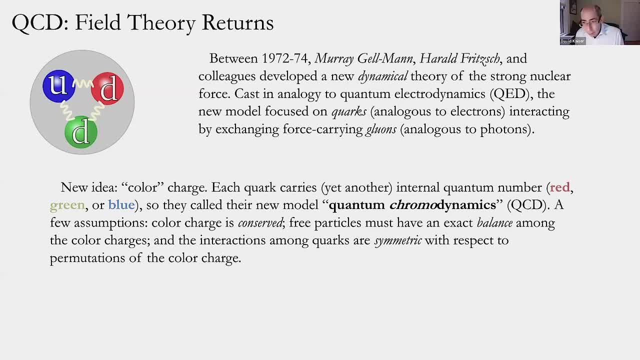 The idea was that each quark carries yet another internal quantum number. This one could have one of three values. So instead of spin or isospin, which were usually one of two values- spin up or spin down- the color charge could come in one of three values. 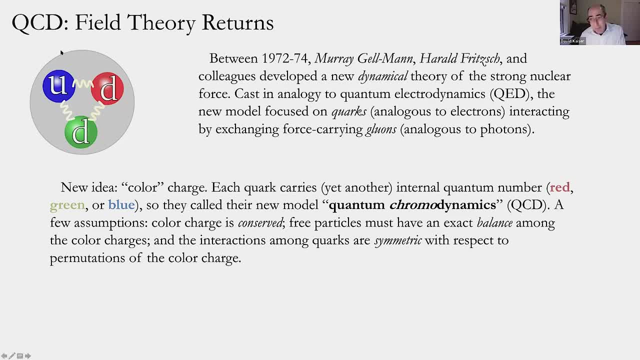 And rather than call it minus one, zero or plus one, they called them. they gave them names like colors, the primary colors red, green and blue, And they did that because they posited several features of this color charge. 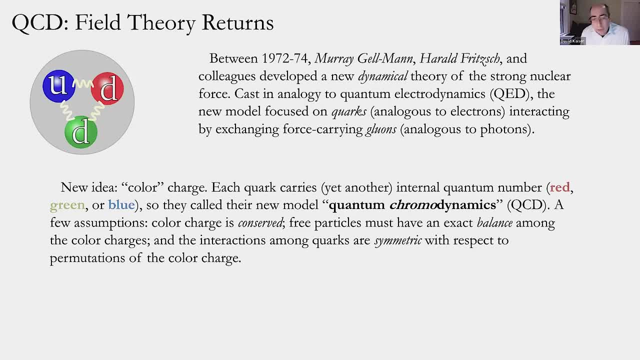 that the color charge overall is conserved. You can neither create nor destroy, say, red quark charge. That the free particles you could ever measure or experience in nature, bound protons, neutrons, ions or anywhere else- have to have an exact balance among the color charges. 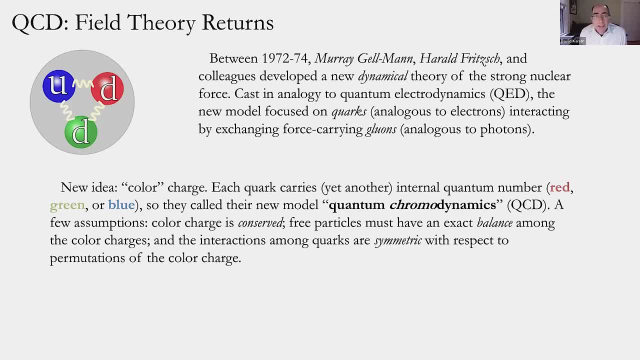 So if you have one unit of red color charge, you must have exactly one unit of both green and blue, and vice versa, And that's why they appealed to the primary colors. If you mix red light, green light and blue light in equal intensity together, 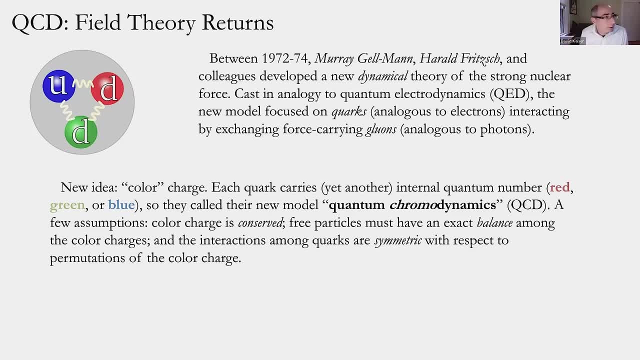 they will make white light or all the color will vanish. basically, You'll have perfect color balance. So that's what they were positing among the color charges on these quarks: That a baryon, a bound state of three quarks. 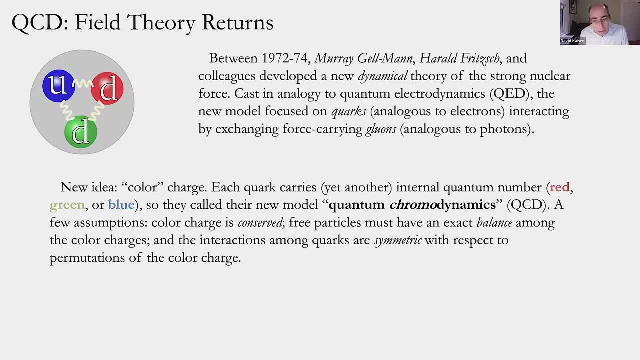 must have exactly one of each color to balance out. The mesons which were like a pion, which is one quark and a bound anti-quark, would have to have one red and one anti-red quark. So together the color charge would exactly balance. 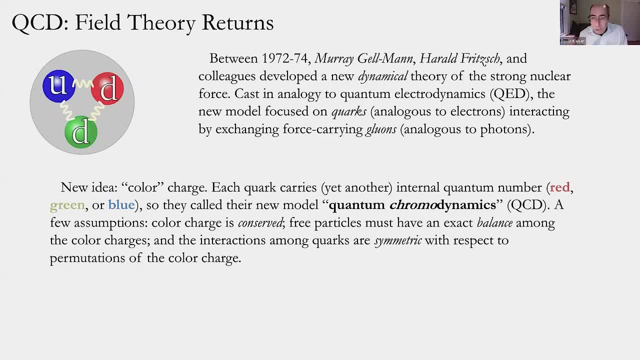 Or one blue and anti-blue and so on. So that's the first two assumptions. Color charge is conserved and you have to have an exact balance. And the last one is that this new force law has to be symmetric with respect to kind of random permutations of the color charge. 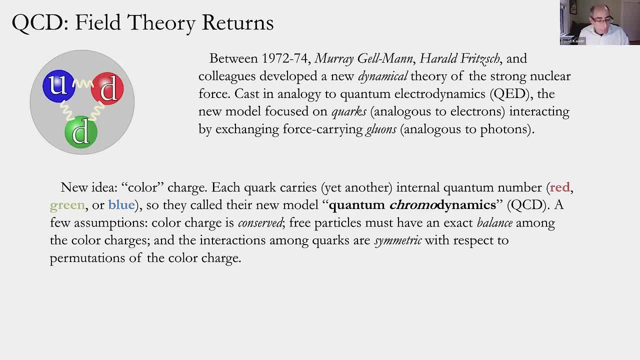 And that's again a lot like the symmetries of isospin. that when you consider a lot of these nuclear interactions about, say, proton-proton scattering or proton-neutron or neutron-neutron, it didn't matter. 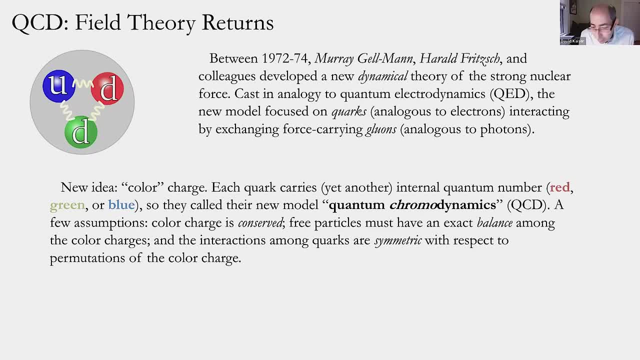 Any random permutation gave the same results. It was a random permutation of isospin, So the nuclear reactions were isospin symmetric, And the idea was that maybe that same kind of symmetry held among this as yet unobserved, maybe even unobservable charge on these elementary constituents, the quarks. 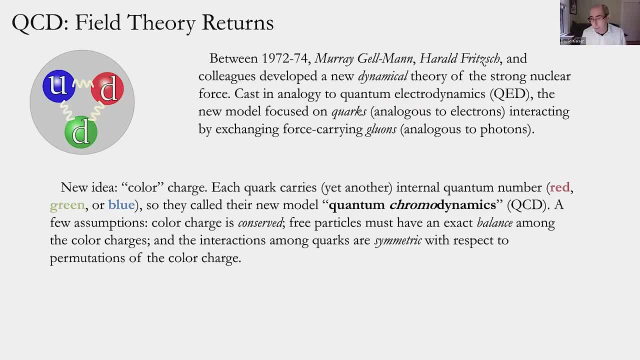 and they could be jumbled up in any old way as long as the total balance remained. So you'd have no free color charge leaking out, because you'd have an exact balance. So those are the assumptions, Then, that you could go back and resolve it. 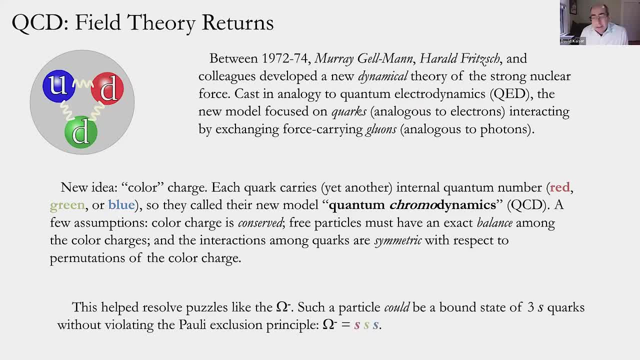 So you could go back and resolve it. So you could go back and resolve it. So you could go back and resolve some of the puzzles like the omega-minus. So now, maybe the omega-minus would not violate the Pauli exclusion principle because it was not three literally identical spin-one-half particles in a balanced state. 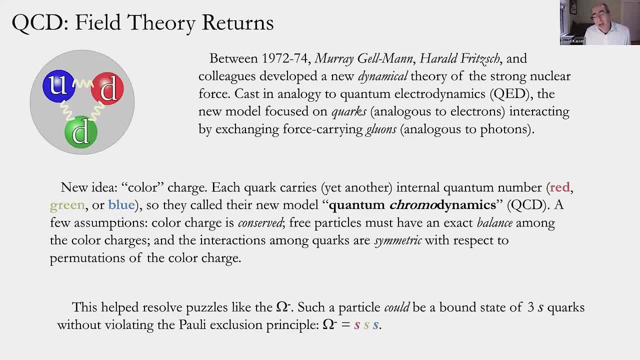 They differed on one more set of internal quantum numbers that had not yet been taken into account. The omega-minus would have to be a balanced state of one red, one green and one blue- strange quark. So no two of them would be in the same quantum state. 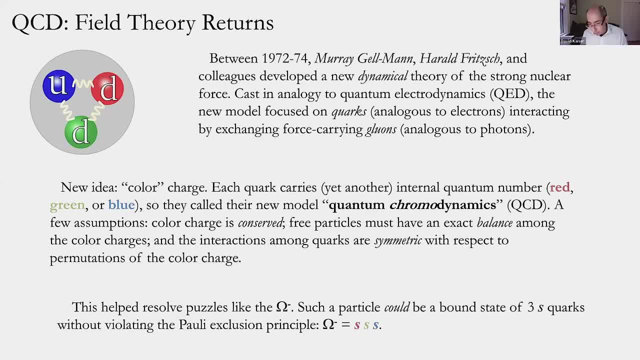 even if they had the same values for all the other quantum numbers, including spin. So now you could have bound states like the omega-minus. This also suggested at least why it might be possible to avoid having fractional electric charge If you always have to have this exact balancing. 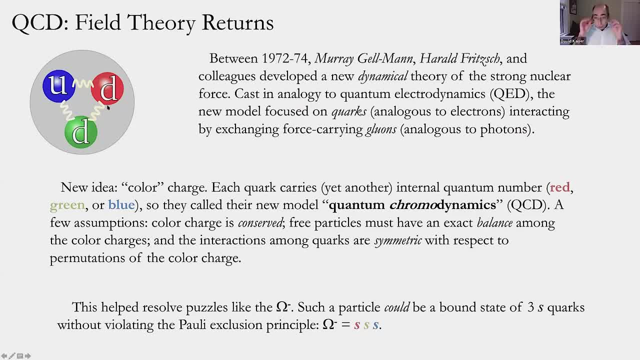 maybe the electric charge always has to come in integer units and never see, say, a plus two-thirds charge that wasn't appropriately balanced by the color charge-preserving quarks. that, as a consequence, would also have to be balanced. It would also get you back to only integer values for electric charge. 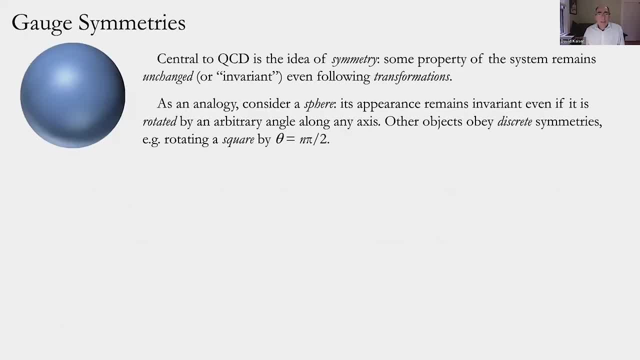 That was at least a hypothesis. Okay, So, as I mentioned even just in that brief discussion a moment ago, really essential to the idea of quantum chromodynamics, or QCD, is the idea of symmetry, that some property of the system remains invariant or unchanged. 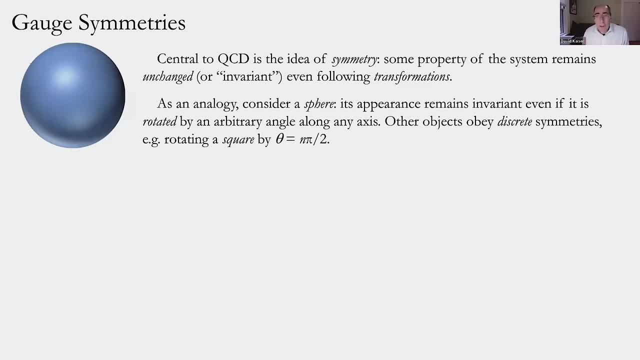 even when certain parts are changed, undergo what we call transformations. We saw how important this was in the study of relativity. It plays an increasing role in quantum theory And by this point, by the early and mid-1970s, the theorists like Gelman and Fritsch and their colleagues were elevating this to a kind of guiding principle. 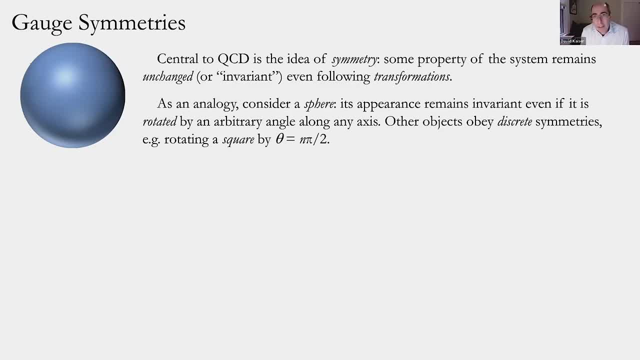 to be driven by what has to remain unchanged, even among symmetry transformations. So again, we're all familiar with symmetries. You can imagine, for example, a sphere: It will appear unchanged, Its appearance will remain invariant, Even if you rotate the sphere by an arbitrary angle. 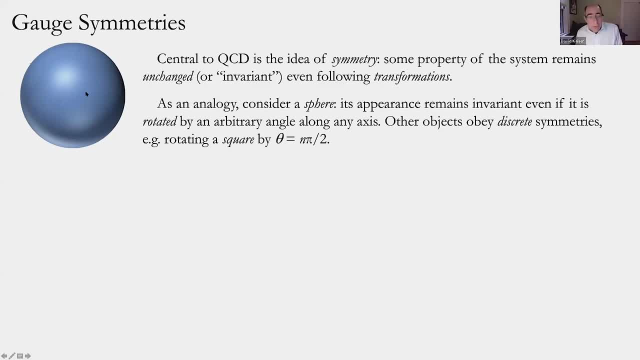 around an arbitrary axis. that's an example of a continuous symmetry. The transformations could be by any angle: 7.1 degrees, 7.1003 degrees- any continuously variable transformation. Likewise, you could rotate the axis itself by any amount. 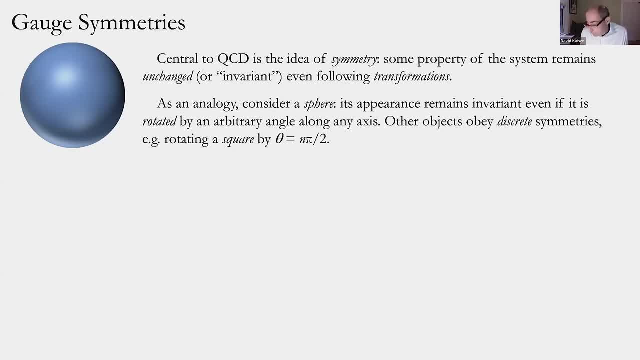 We're also familiar with things like discrete symmetries. Imagine a square, a simple two-dimensional square. Its appearance will remain invariant if you rotate it by any integer number times 90 degrees. Rotate it by 90 degrees. you can't tell the difference by 180, by 270.. 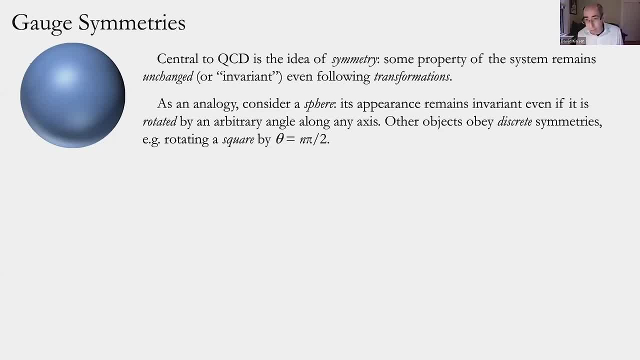 If you rotate a square by 37 degrees, you can tell the difference: It no longer looks unchanged. So that's an example of an object that remains invariant under discrete symmetries, a more kind of constrained set of transformations that will nonetheless leave the appearance unchanged. 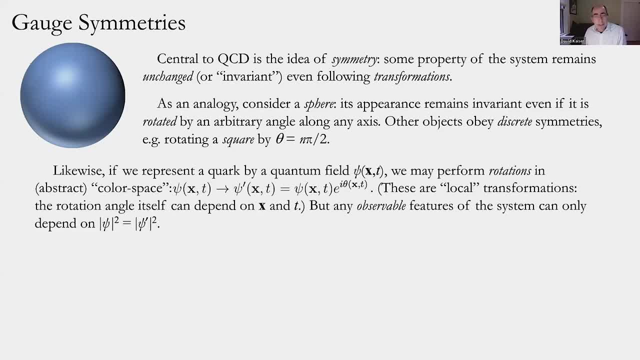 So we're familiar with these kind of everyday examples from geometry. Then we're going to start applying this to these more abstract internal mathematical spaces of these things like color charge. And what if there were symmetrical rotations, in this case discrete ones? 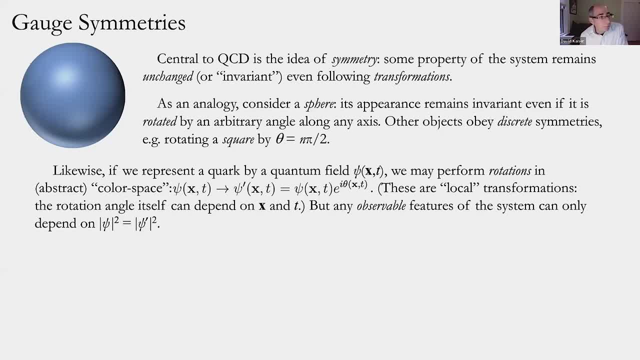 because there are only three values of the color charge: red, green or blue. So that's more like the square. You could rotate a red quark by kind of one unit in color space or two units or three, but not by 1.2 units. That would be like the square being rotated by something other than 90 degrees. 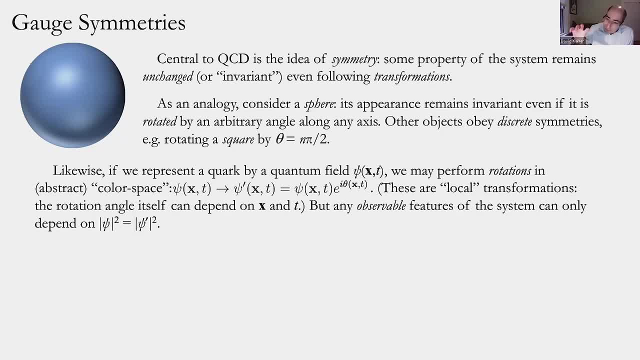 So it's a discrete symmetry and not that you're literally picking up a quark and rotating it, but you're changing Its description in this abstract mathematical space, of color space, So you could perform rotations on your quantum field that represents a given quark. 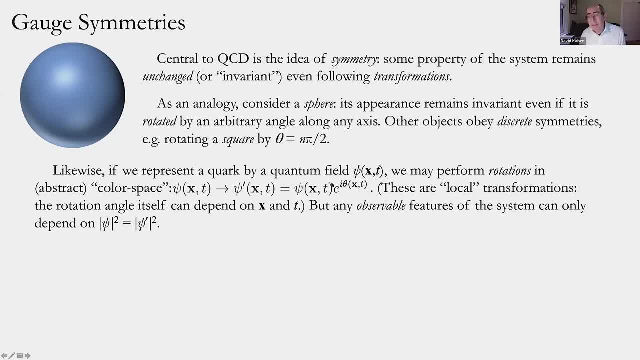 You could transform it by rotating it by some angle. in color space, The angle has some constraints. like I mentioned, it's a discrete symmetry. Moreover, in this case, you could be changing the angle of rotation at different times and places. This is what's called a local transformation. 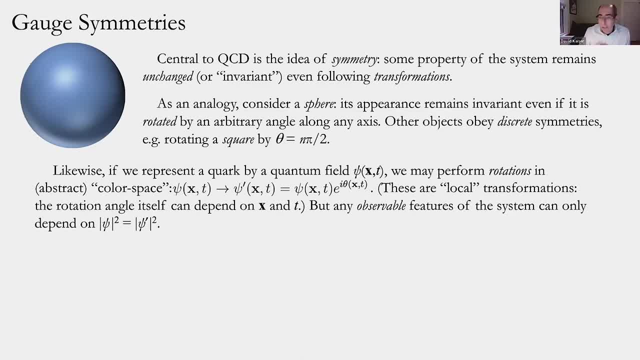 So it's not just that you take a red color quark and you rotate it once and you're done That same. the excitation of the quanta of your quark field could be rotated by two clicks of the turn over here. 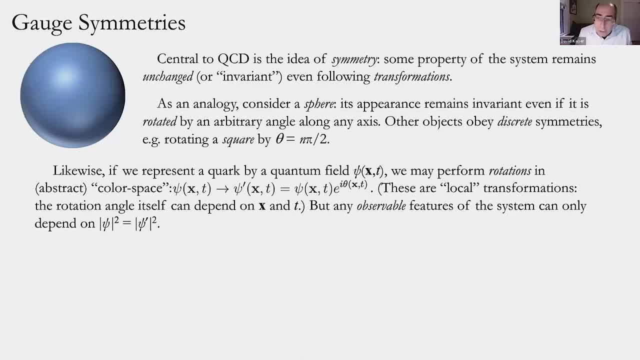 but by minus one click over here and you could change your mind over time. So these are called local transformations And the idea, which was really just a hypothesis, that was driving people like Gelman and Fritsch and others, was that: what would it take to leave any observable features of such a theory invariant? 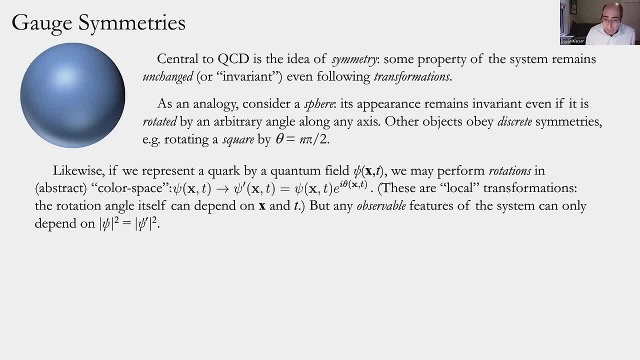 even under that set of quite wide spans. Well, you could do that by expanding transformations. So one thing you could do is make sure that the observable features of the system only depend on the kind of length of that quantum field. That would be like a radial symmetry, if you think back to the sphere. 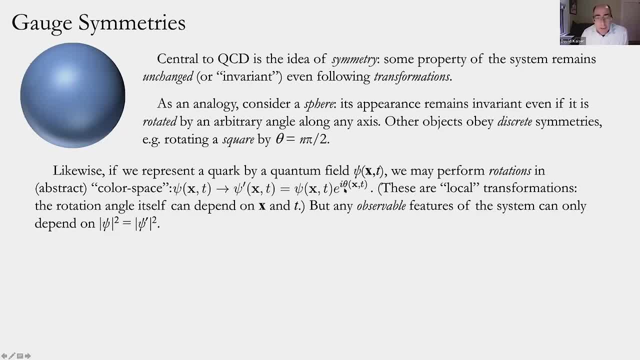 If you rotate your quantum field by some fancy phase here, if the observables only depend on the absolute square, then the rotations will cancel out. You would, you would any, any trans, any local transformation would fall out. Remember, they're now trying to handle dynamics. 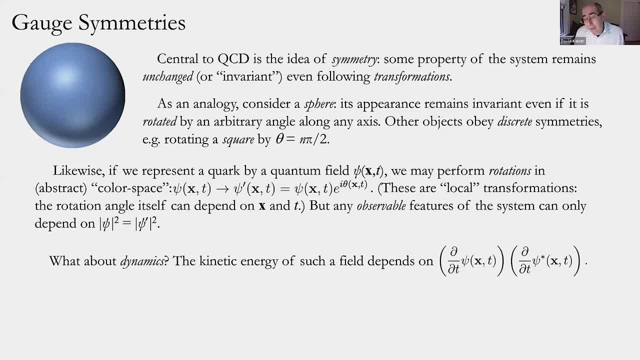 They're trying to explain change over time and not just a static configuration. And that's when it gets much trickier. And this is really where the real work had to come in If you try to describe the behavior of that quantum quark field over time quantitatively. 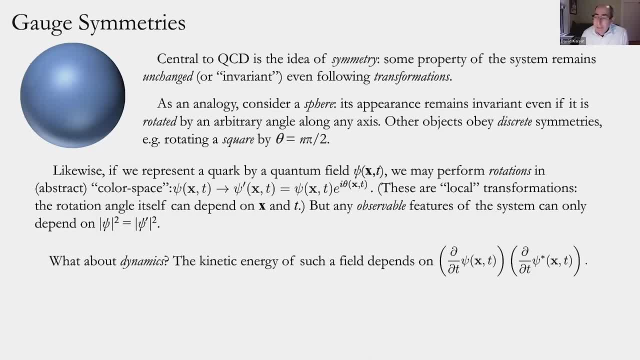 it obeys an equation kind of like the Schrodinger equation, a little different, but it has sort of time dependencies, it has spatial gradients, it has derivatives. Well now, if you perform these local transformations where your rotation angle itself can, in principle, depend on both space and time, 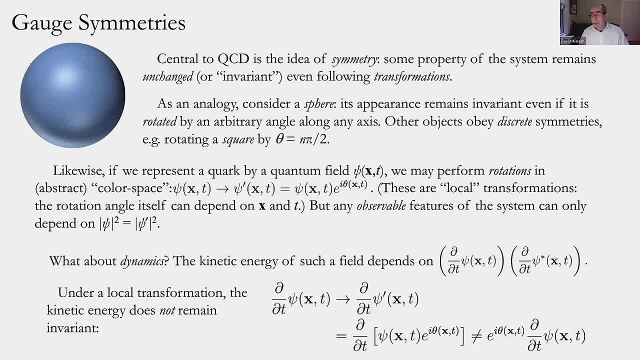 you get in trouble with the, with the kinetic energy, with the change of that quantum field, If the field itself undergoes a rotation. so psi goes to psi prime. now we're taking the time change of this slightly more complicated object and we'll have a chain rule. 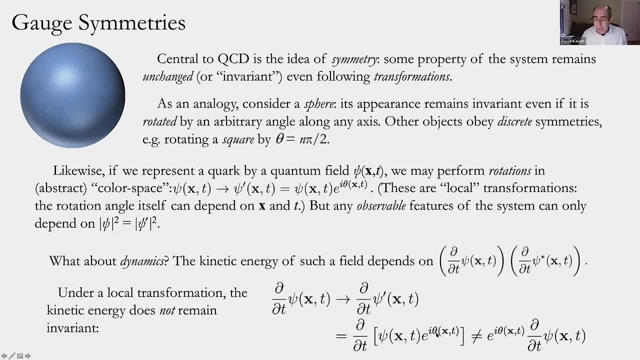 There'll be psi times the derivative of theta, plus theta times the derivative of psi. It will not be such that the phase terms will just cancel out If we go back to this term for the kinetic energy. if the if the derivative of the rotated quark field had just the phase pulled out front, then it would cancel. 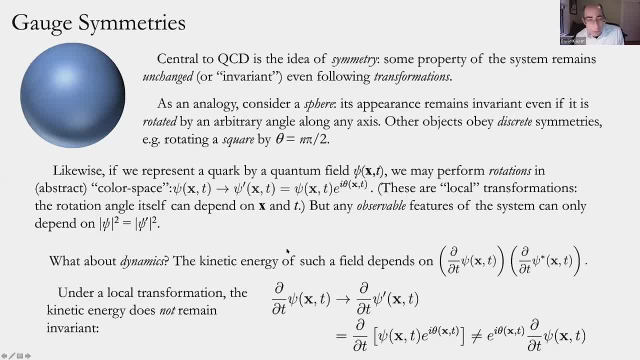 We'd have one term times its complex conjugate. It would be just like the radial symmetry here. But we don't have that anymore because of the chain rule. We have to involve a more complicated set of dynamics To ensure that that overall symmetry is preserved. 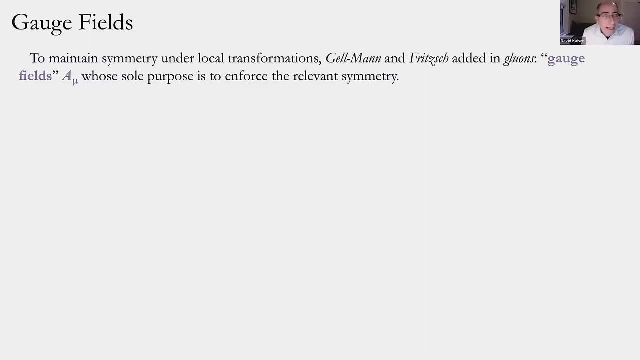 And so that's, that's what then Gelman Fritsch and their colleagues do next To maintain that symmetry under local rotations in that color space- red, green and blue quark color- they add in this these force carrying particles with very specific properties. 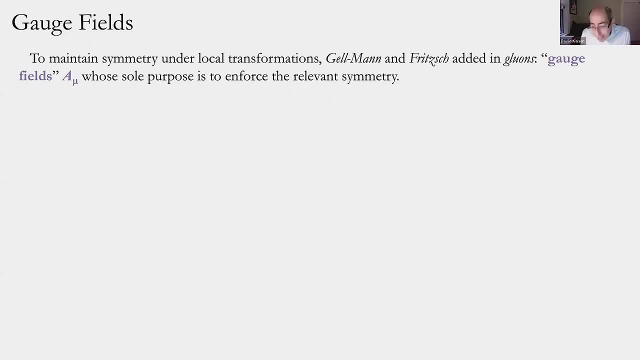 that the gluons have to behave a certain way as well. In fact, the gluons in some sense are added for the sole purpose of enforcing that symmetry. So the quark field could, to undergo these very fancy rotations, all the permutations of color charge. 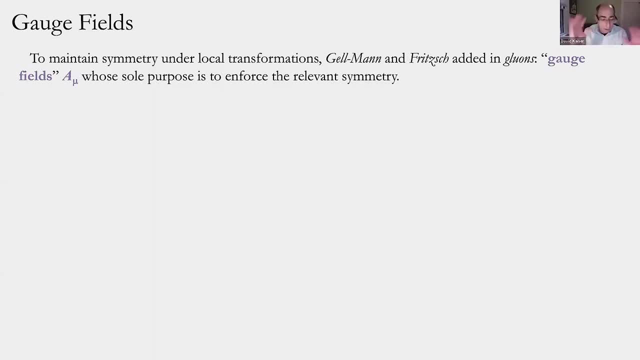 and to leave all the observables, including dynamics of forces over time, to leave all those unchanged. these other kinds of matter. the gluon fields have to have very specific properties And this goes- this is a little technical, Don't worry if this goes by too fast. 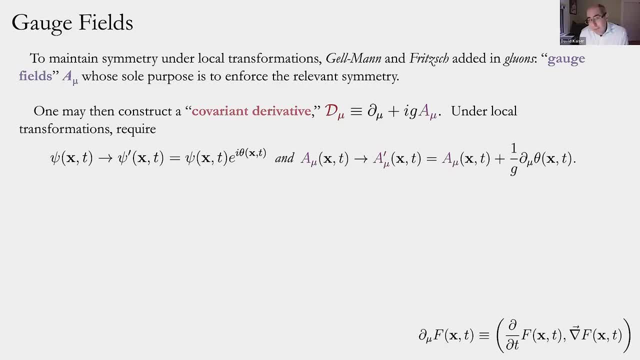 There's no quiz. But what they do is they construct what's called a covariant derivative which combines the, the change in- sorry, the change in- space and time. This is just shorthand for taking the time derivative and the spatial gradient. 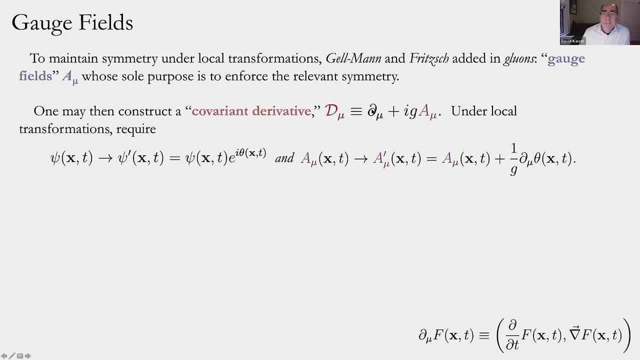 This is just the derivative of the quark field in time and space. But instead of only worrying about its change, that way you say, it also couple. it also interacts with these gluon fields. And if the gluon field itself has a very specific transformation? 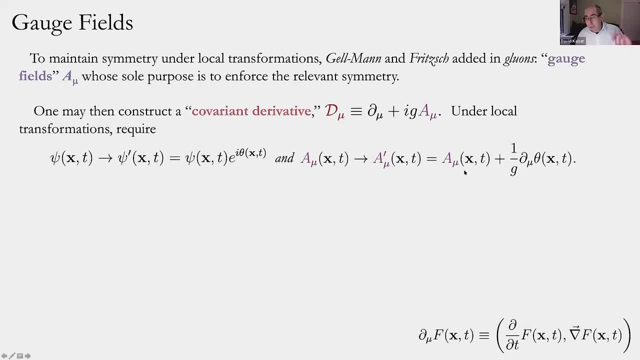 so if you rotate a quark color, you also have to do a transformation of the gluon field at the same time. If you choose that transformation very cleverly, then your covariant derivative, this combination of changes in space and time, plus the very particular way that the quark field interacts with the gluon- 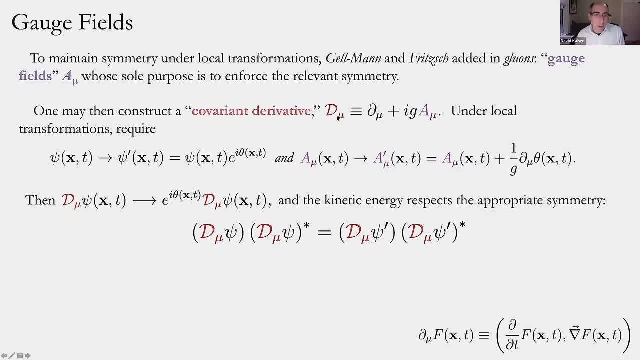 field. that will leave this souped up derivative, the covariant derivative, such that you actually get this overall phase factor out front. And now the kinetic energy remains unchanged. Now your e to the plus i, theta is exactly canceled by its complex conjugate. 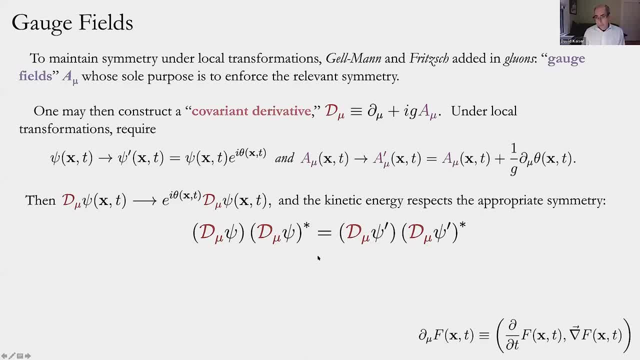 So now your your souped up kinetic term remains unchanged. So you can see that the quark field is totally invariant even under these more elaborate color charge symmetries. So you can have quarks that run around the world with different colors. 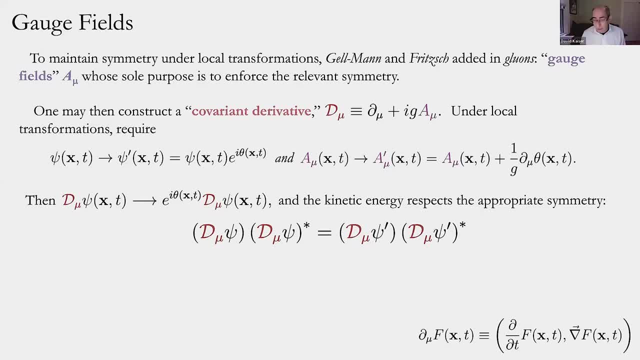 red, green, blue. the color assignment to a given quark could change over time and across space And as long as you have an additional kind of matter running around with them, these gluon fields, And if you specify very quantitatively. 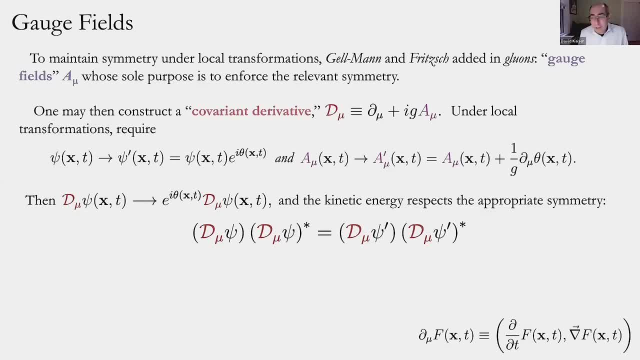 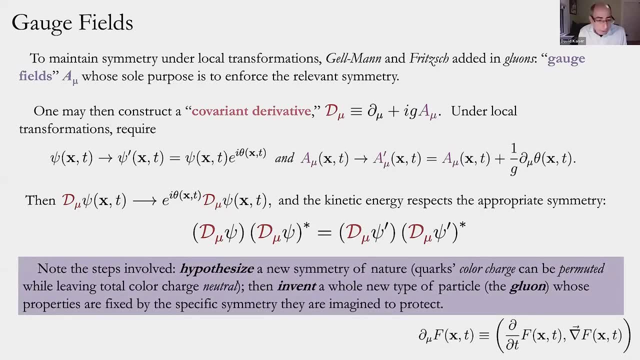 how the gluons have to behave, much like the quarks together. you can see that the quark will remain symmetric under that symmetry. That's again a bit more abstract, But the idea is conceptually is, I think, really pretty astonishing. Basically, gelman and French and their colleagues have to dream up 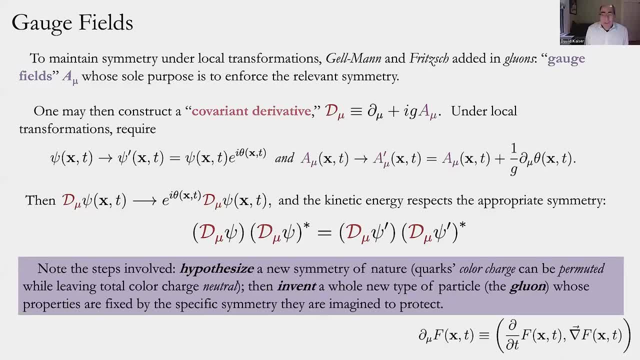 have to hypothesize a whole new kind of matter, The glue on fields, Strictly to enforce a symmetry which was just of their own thinking in the first place. So they, because they're so enamored by the symmetry properties that made sense of. 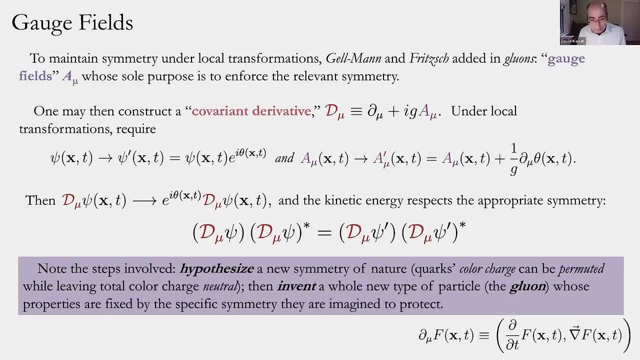 all the kinds of classifications of the nuclear particles. they're so enamored by the symmetry properties. They're so enamored by the symmetry properties That they're really smitten with this idea of an underlying symmetry. But when they really really want to describe the forces that would owe, that would. 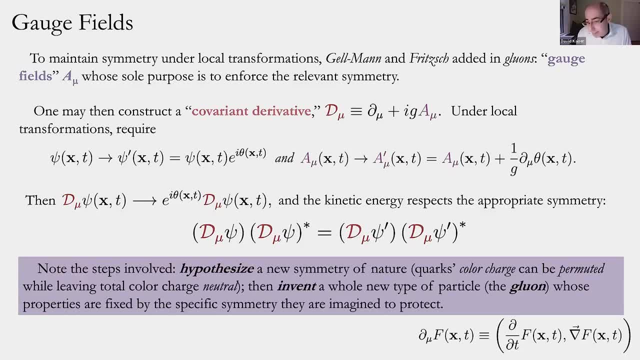 Obey that symmetry, Remain consistent with that symmetry. They can't do it with quarks alone. They have to have quarks interacting in a very specific way Within the whole separate family of matter: the glue on fields And it is kind of coordinated dance, And then the whole collection. 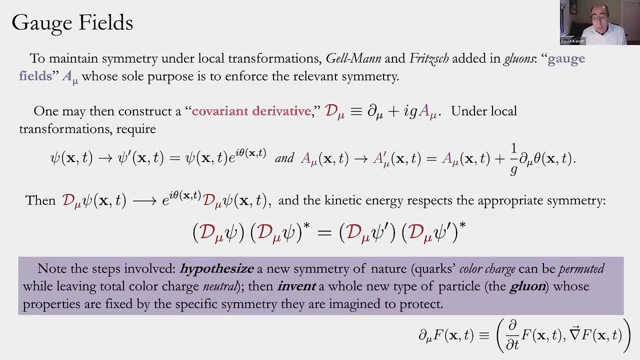 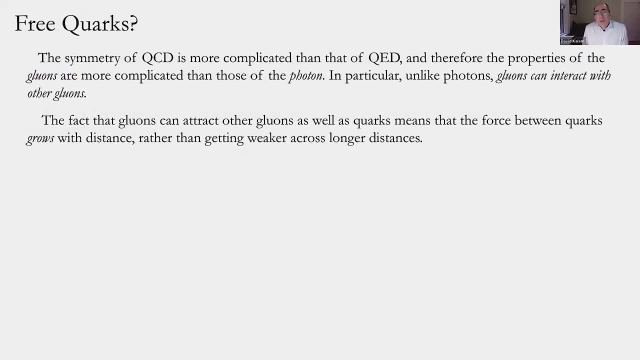 this kind of rickety collection Would, would protect or enforce that symmetry. I find that pretty astonishing. So the symmetry of quantum chromodynamics is more complicated than that of other examples of these kinds of models, like quantum electron, And therefore the properties of the glue ons are actually more 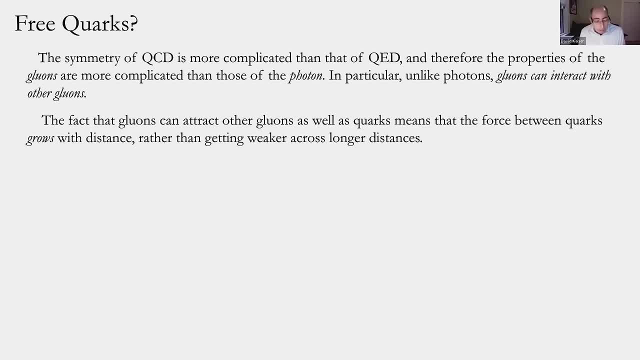 complicated than those of the photon. in particular, The color charge is a discrete symmetry, Whereas the phase freedom for the electric charge is a continuous symmetry. So the gluons really have much more kind of articulated mathematical structure, And one consequence of that is that the gluons can actually interact. 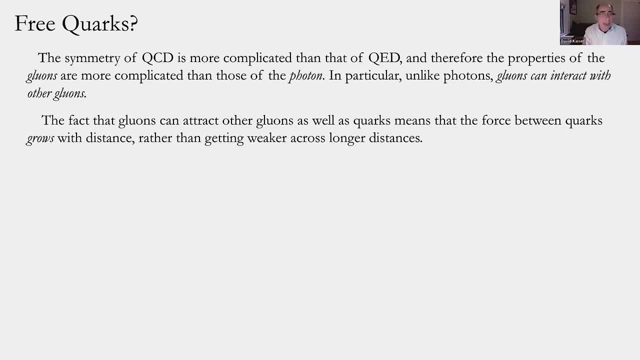 with other gluons, or at least they're all still hypothetical at this stage. But in order for all that symmetry preservation stuff to work, for the math to work out, The gluons have to be able to scatter off of other gluons or attract. 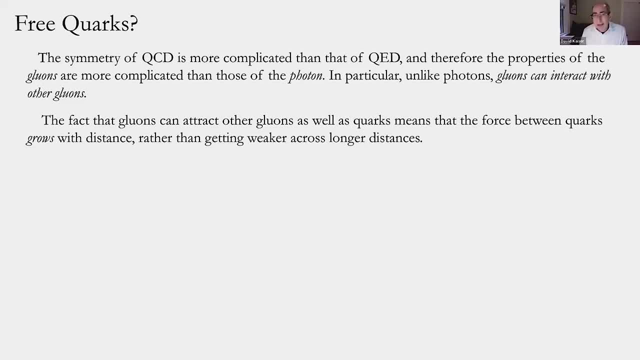 other gluons, Whereas photons don't do that. Photons don't have electric charge, So photons only scatter off objects with electric charge, at least according to QED. So photons will scatter off of electrons or positrons or protons. Photons won't scatter off of neutrons, at least not directly. 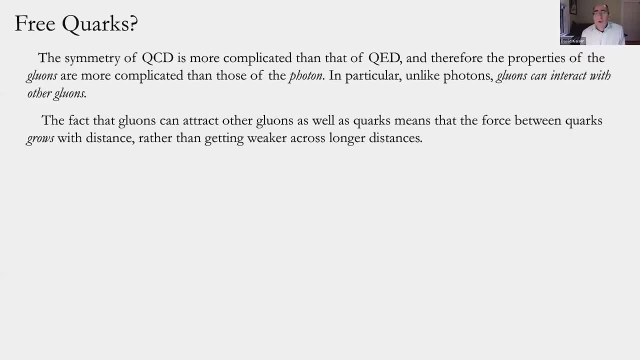 And they certainly won't scatter off each other, Whereas gluons can scatter off each other as well as off of the quarks. Another way to say that a bit more succinctly is that gluons also carry color charge, Much like quarks do, whereas photons not carry electric charge. 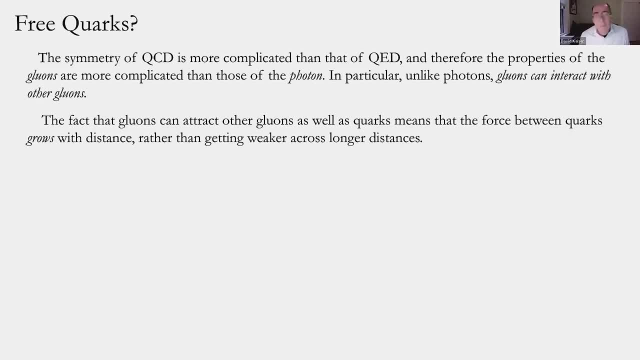 Okay, So the fact that gluons can attract each other Actually changes the kind of force law between quarks, The, the, the. the force between quarks will actually grow with distance, Because the distance between them is filled with gluons and the gluons. 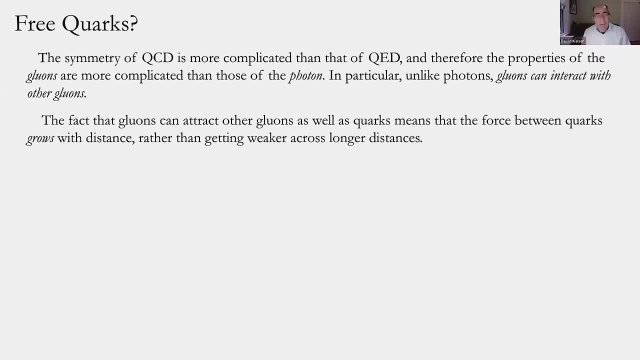 themselves can interact with each other. So it starts looking a bit actually like a kind of stretched rubber band. There's a kind of elastic Restoring force, at least as predicted By quantum chromodynamics, which has no analog In, say, the force between an electron and a positron. 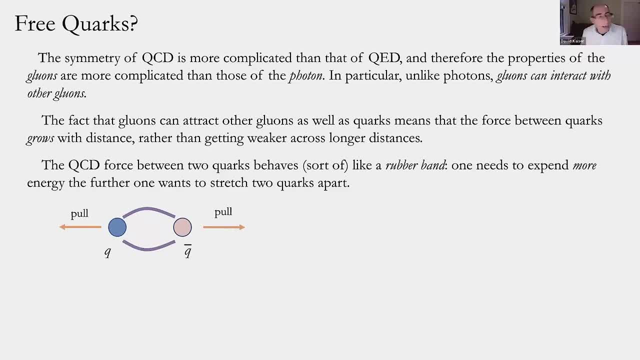 Remember the, the attraction of the electron and the positron. It's not the same thing, But it's the same thing for the electric charge. It's one of the things that's actually. It's not the same thing. So actually, a force between two electrons is in the same direction. 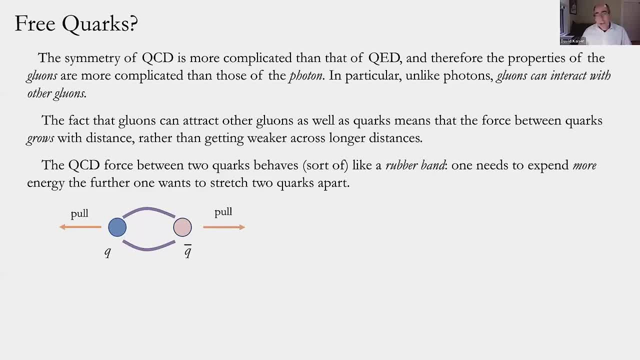 So the electric charge, The attractive force between opposite electric charges, Falls off with the distance. That's a famous crew load law. In fact, the force falls off like the square of the distance. So they could still exert an attraction across space. 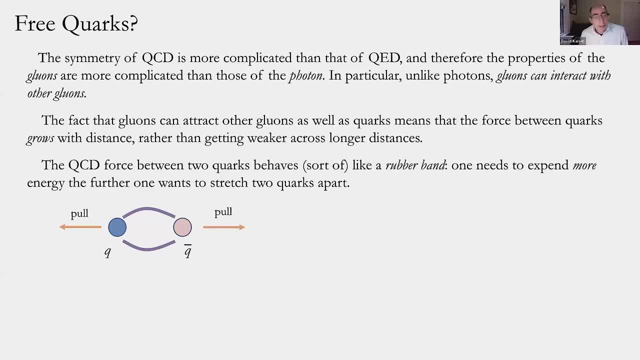 But if you double the, the distance, The, the, the strength of the attraction Falls by a factor of four. With glue up with a, with quarks Attracting each other by this Highly symmetric, strong nuclear force. 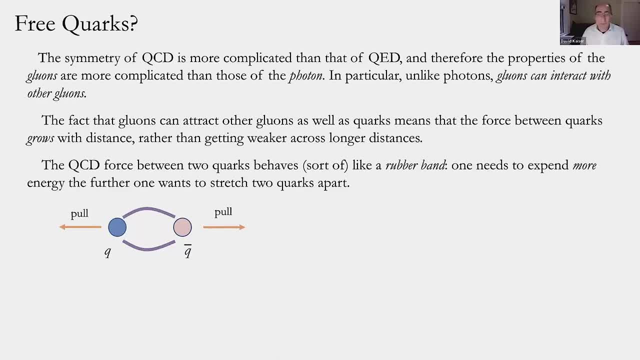 It seems to go the other way, That the forest explanation of why it's so different is because the gluons that are mediating that force can actually kind of glue onto each other, so to speak, and attract each other. So if you imagine, 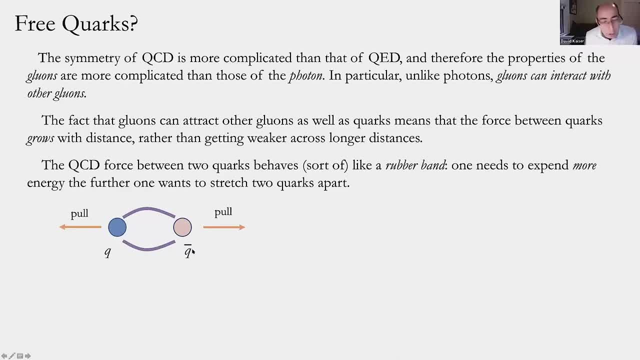 trying to stretch to a bound state of a quark and an anti-quark apart. this could be, for example, a pion, some sort of meson, and you could instill external energy by pulling on these two particles. try to pry them apart by adding external energy to the system. At some point you'll have to add. 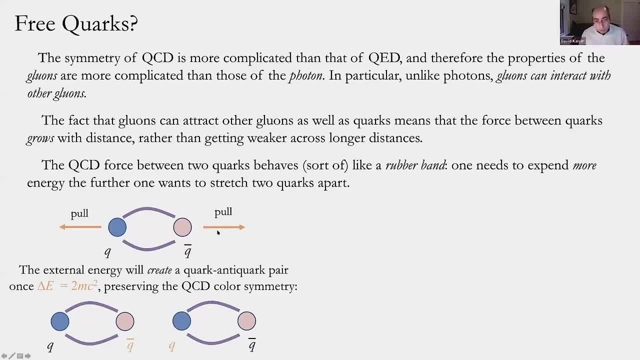 so much external energy. You'll be tugging so hard, adding so much external energy that you'll actually create a whole new quark-anti-quark pair. In a sense, these were already around. They were virtual quark-anti-quark particles, but they can now borrow the energy you've given. 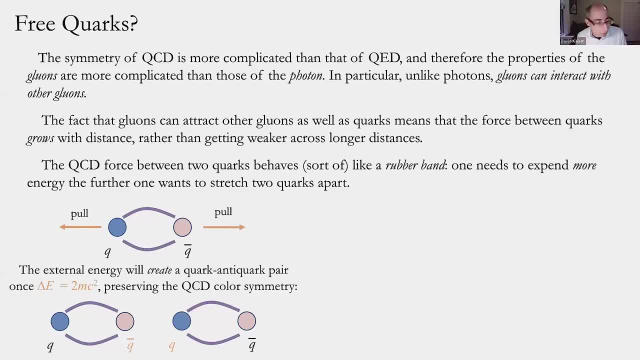 that system to become real particles, They now can pay off their debt to the vacuum. If they were virtual particles, they now can pay off the energy they borrowed As soon as you give to the system enough energy to cover their masses. So, in fact, when you try to pull a quark and an anti-quark apart within this scheme, 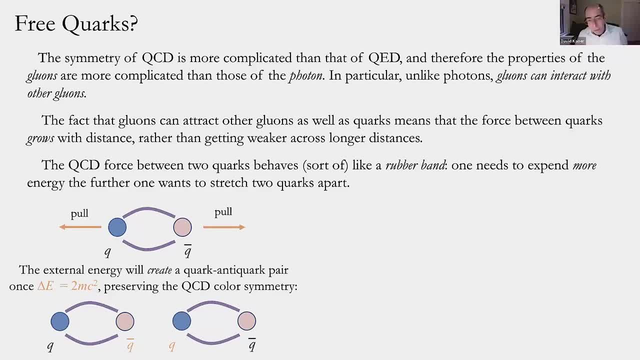 at least hypothetically. you'll never get a free quark isolated, You'll never see a fractional charge. In fact, what you do is you'll create two bound states of quark-anti-quark pairs, where before you'd only had one. And so that again comes because the gluons can interact. 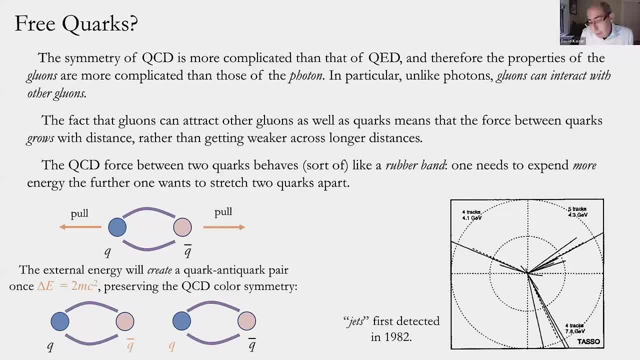 with gluons directly. So that was a prediction from QCD By the later 1970s that worked out A few years after this symmetry-preserving scheme And that again gave experimental colleagues something to look for, some specific kind of thing to look for in the high-energy. 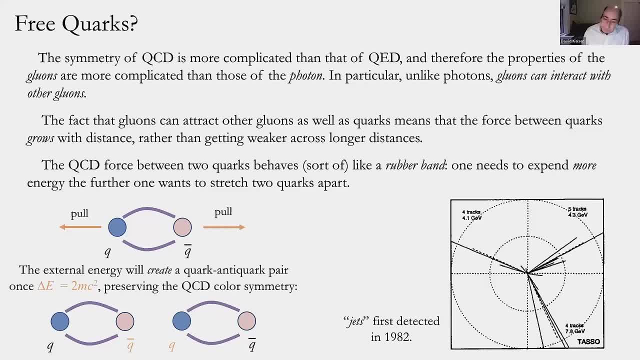 scatterings of these nuclear particles And the first evidence in concert with that idea was presented by an experimental team in Europe. I think this was a group in Germany in the early 1980s. These came to be called jets. The idea was: you would have these sort of jets. 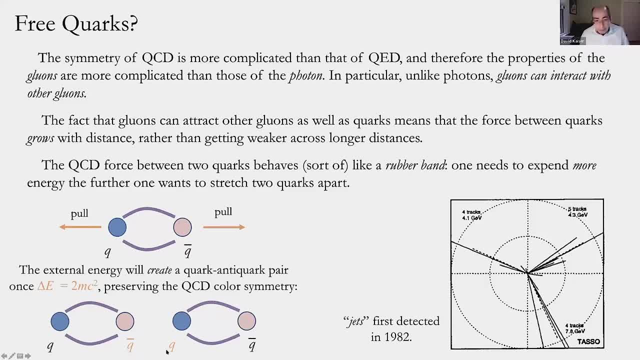 streaming off where the original beam might have gone One direction and this sort of not quite torn apart but rapidly reassembled pair of mesons would jet off in opposite directions or nearly opposite directions, So you could have a very specific pattern of the debris coming out of the very high-energy collisions of these. 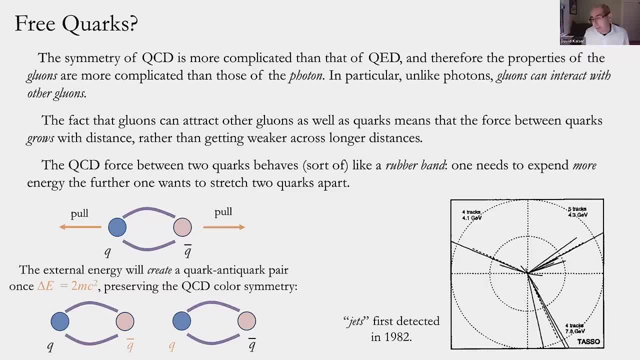 particles, because in the effort to crack apart a quark and an anti-quark pair, for example, you wind up making more kinds of particles that will jet off away from each other. So these were actually predictions of this new theory, based again on the idea of preserving symmetry. 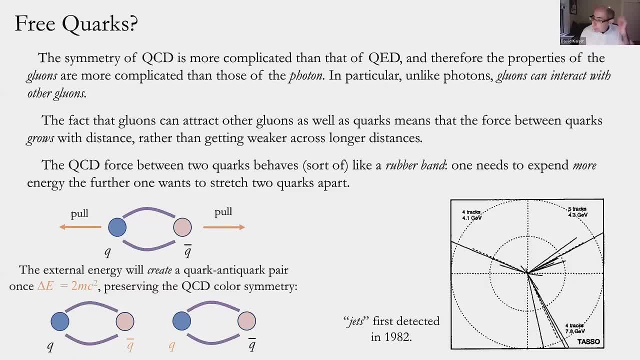 and having a certain way in which the force-carrying particles interact with the quarks, And that was at least consistent with some of the new experimental data- within just a few years- It was at that point by the late 70s, early 80s, not in 1964 or 1967 or any other steps along the way. it was really 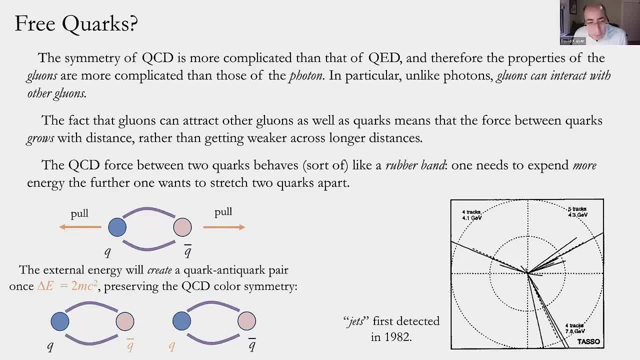 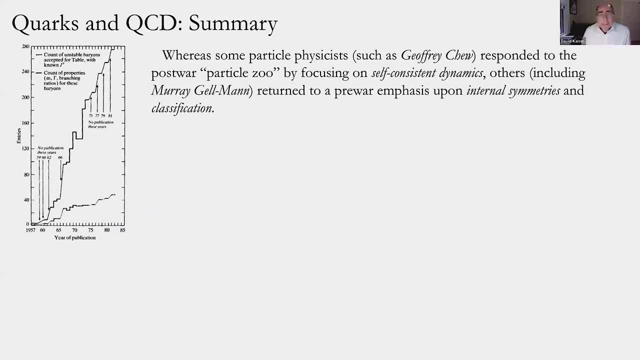 at that point that the community began to coalesce around the idea that quarks might actually be real particles in nature and not just a mathematical abstraction. So let me wrap up here One of the responses to this particle zoo after the end of the Second World War, as we saw, 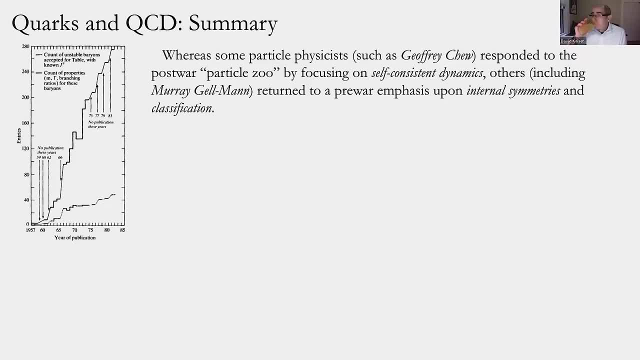 was to kind of double down on dynamics, like Jeffrey Chu, to say all these particles are in some deep sense equally elementary because they're all composites of each other. But as we've been tracking in today's class, there's a kind of parallel, complementary approach, really, kind of led by Murray Gell-Mann. 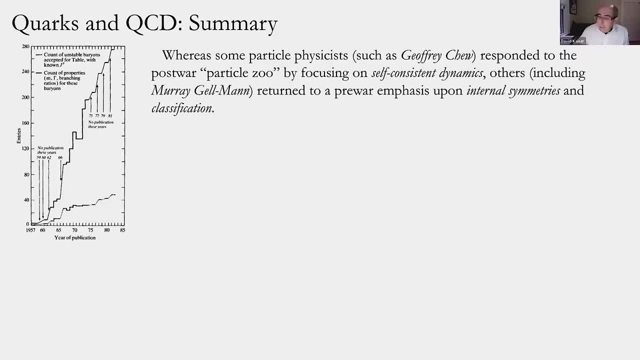 though many other people were making contributions along the way- which was to kind of bracket the question of forces or dynamics for a while- really for 20 years- and just to try to figure out: are there patterns in the kind of detritus that comes out of those new accelerators? 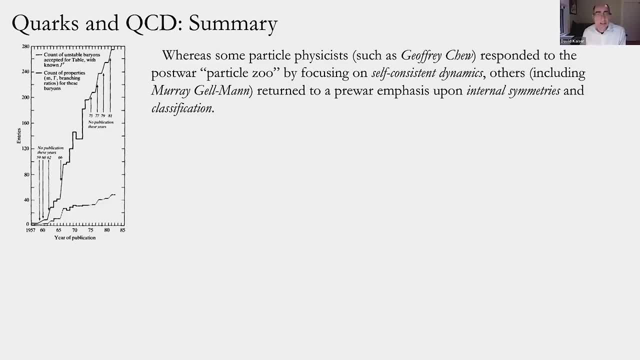 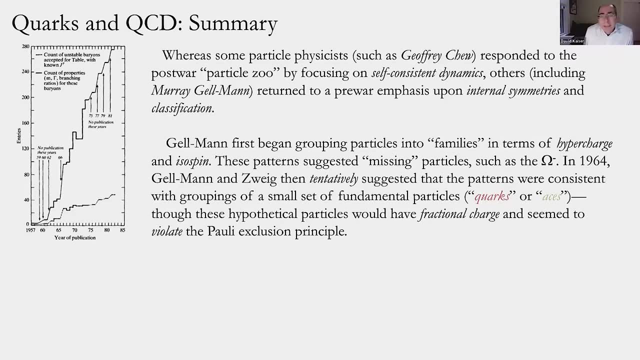 to emphasize classification and internal abstract symmetries. So Gell-Mann and others- but Gell-Mann again really took the lead at this- began grouping these particles into families based on these kind of invented new quantities that did not have an obvious relation to kind. 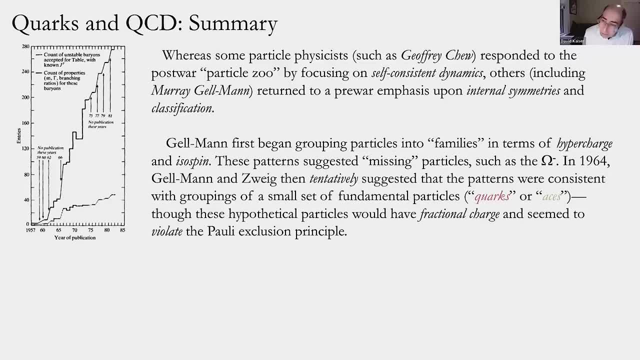 of measurable properties. So he invents hypercharge, he makes use of Heisenberg's older notion of isospin and he starts grouping these particles in these very abstract, mathematical, highly symmetric spaces of hypercharge versus isospin. That enables him to find kind of gaps. 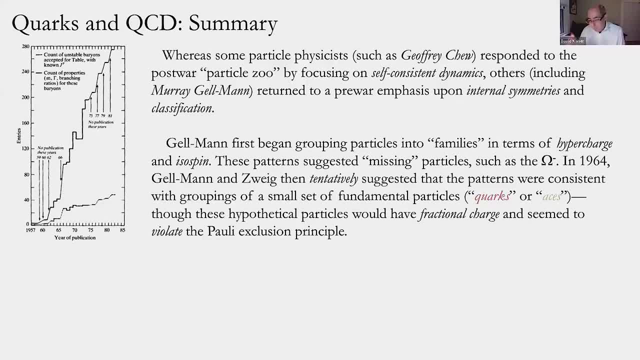 between these kinds of patterns and he predicts very boldly that there should be actual particles out there. famously this works for the omega minus. And then he finds, he suggests very kind of schematically, heuristically, early in 1964, that maybe those patterns were consistent with. 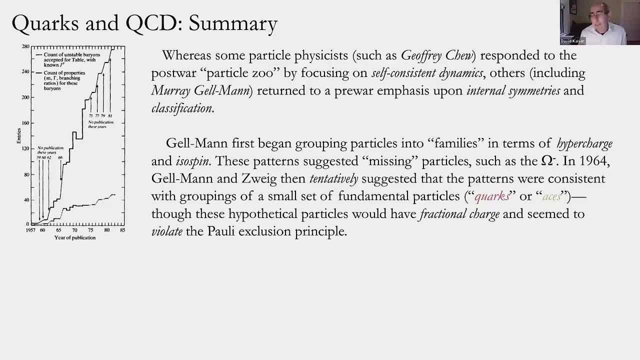 a small set of something more fundamental that might not actually be real bits of matter. So the quarks, or what Zweig calls aces, are very kind of tentatively suggested as a kind of way of accounting for symmetries, because they're out there, part of the world, in part because there were such. 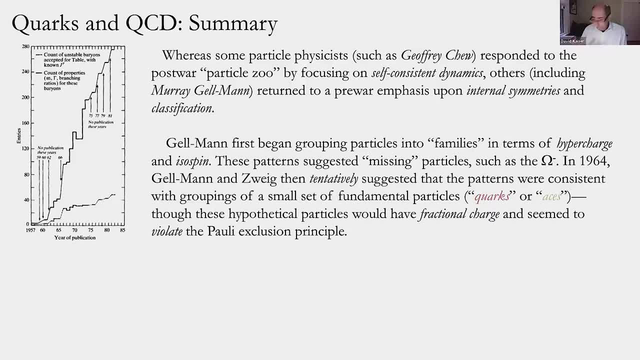 steep conceptual challenges to thinking of them as part of the world fractional electric charge exclusion principle and all the rest. The SLAC-MIT experiments, or I should say the MIT SLAC experiments from the later 60s, produced suggestive compelling evidence that protons and similar nuclear particles 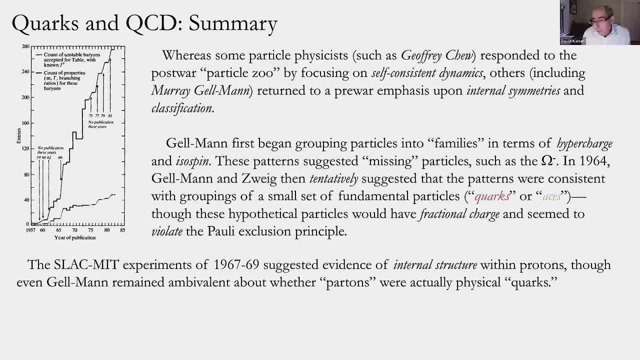 had internal structure. but it was not at all clear to the community, even to people like Gell-Mann, let alone to friendly rivals like Richard Feynman. It was not at all clear right away that those internal scattering sites were the same as these. 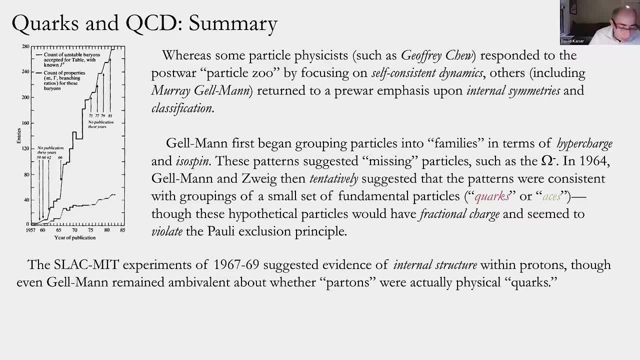 quarks. In fact, even years later Gell-Mann would say that quarks are fictitious. There might be parton structure within protons, but that need not be the same as quarks. We saw that was in hindsight taken to be very, very compelling evidence that quarks exist. Friedman, Jerry Friedman, won the. 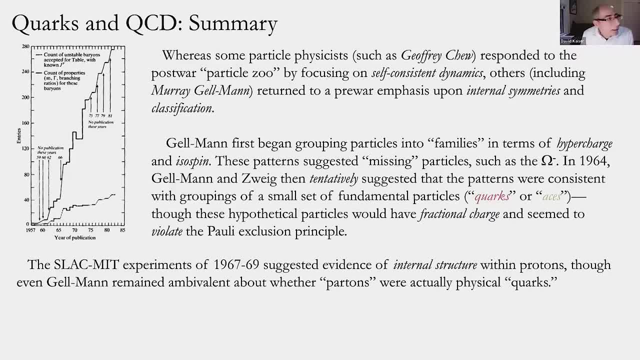 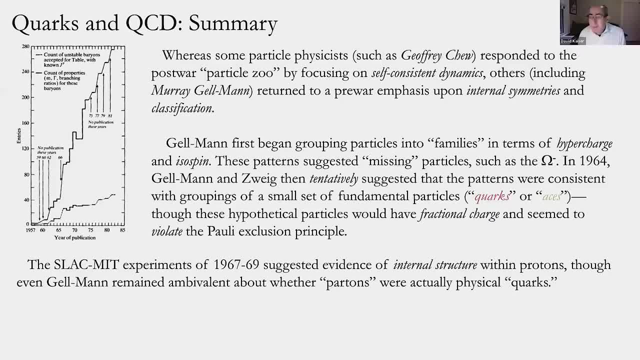 really important touchstones where we think quarks are physical particles. But again it's important to see there was this. didn't tie everything up with a bow right away. There's really the combination of that plus follow on experiments like the jets from. 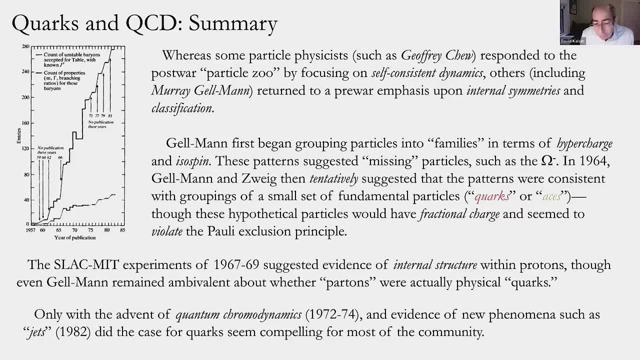 from 15 years later, plus a much more articulated theoretical structure which reintroduces quantum fields, doubles down on these internal symmetries. It becomes known as quantum chromodynamics. These combination of theoretical and experimental ideas and contributions come together over a kind of 20-year period, by the end of which most physicists then would say: